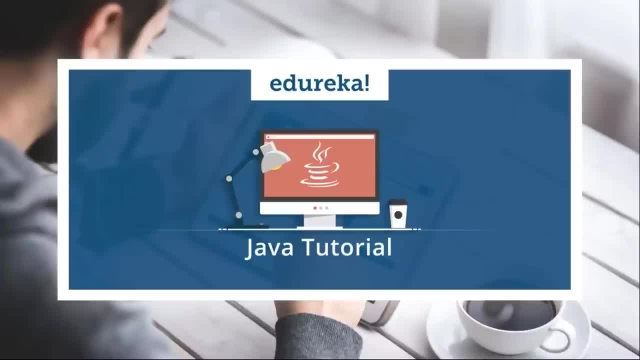 Hey everyone, this is Neil from Edureka, and welcome to today's session on Java Tutoria. Now, we've all heard of Java, either from our friends or from the internet, and Java is something that you would quite often hear across from different sources as well, So you may all be 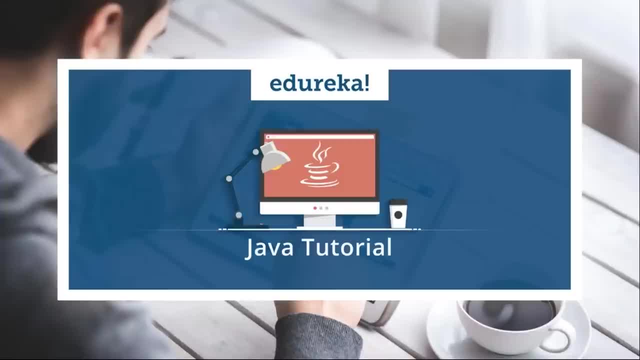 wondering what Java is and what does it exactly do, and we're going to understand what Java is, how it functions, as well, as I'm going to help you build a good fundamental knowledge in Java as part of today's session. Now, keeping that in mind, let's move forward and look at today's 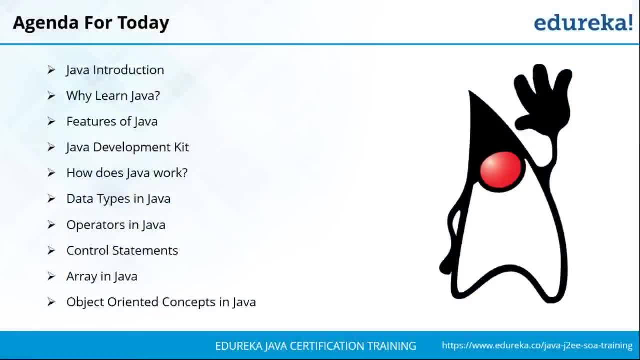 agenda. Now. we'll start off with an introduction to Java, Then I'll help you understand why you need to learn Java, and then we'll be discussing the various features of Java. After that we'll be looking at the Java Development Kit and then, following that, we'll understand how. 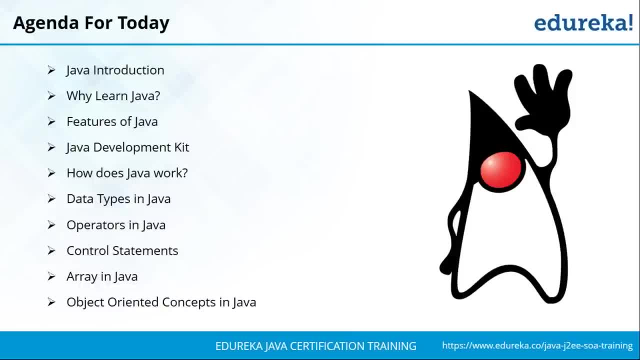 does Java work? Once you're clear on these concepts, we will move into the core Java and we'll understand the various data types in Java, the various operators that you can use in Java. I'll also help you understand the control statements in Java and we'll be discussing 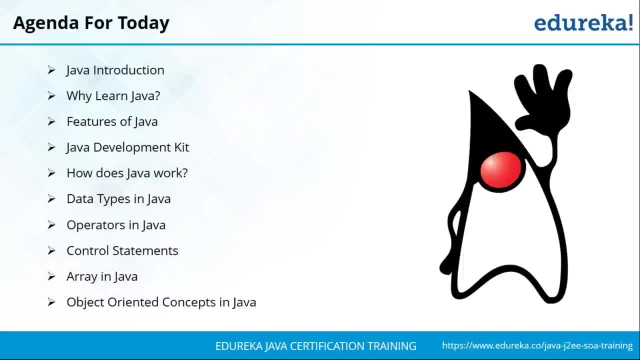 about arrays in Java. Finally, to give you a good fundamental knowledge, we'll also be discussing about the object-oriented concepts in Java. Now are we clear with today's agenda? Okay, Prashant says yes, I've got a confirmation from Aaron Ann Henry, Divya Bharat Deepti. 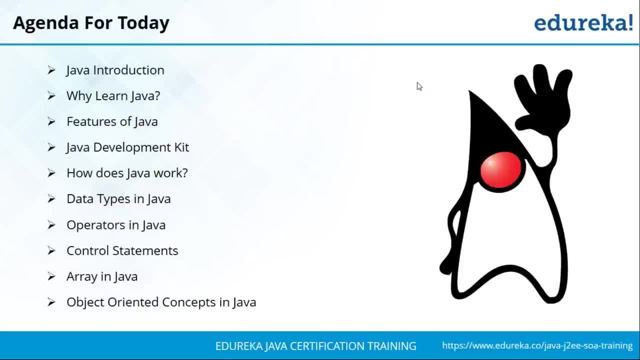 That's great to see guys. So one thing I'd like to clarify right in the start itself is: at any point, if you're not clear, if you have any doubts or any questions, please put it across in the chat window so that I can clarify it then and there itself. 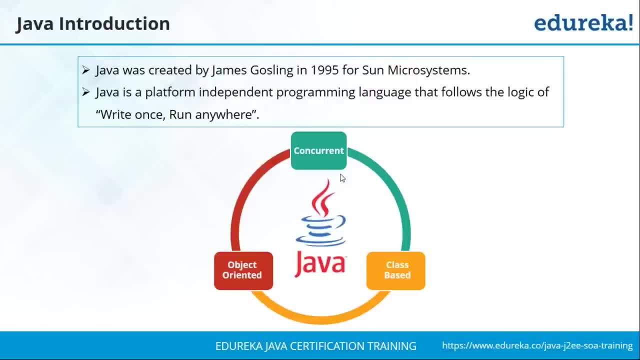 Now let's move forward and have an introduction to Java. So Java was created by James Gosselin in 1995 for Sun Microsystems. So Java was originally planned to be named as Oak, but that name was taken. So they went after and named it after their favorite coffee, which was Java. 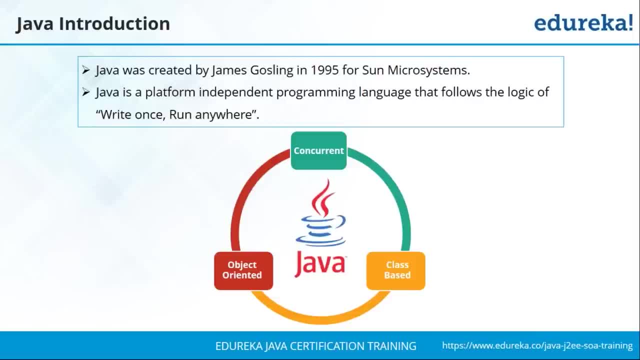 Now, Java is a platform-independent programming language. Now, when I say platform-independent programming language, what they basically mean is that once you've written your code, you can run it anywhere as such, So there's not going to be any specific dependencies or any changes that you need. 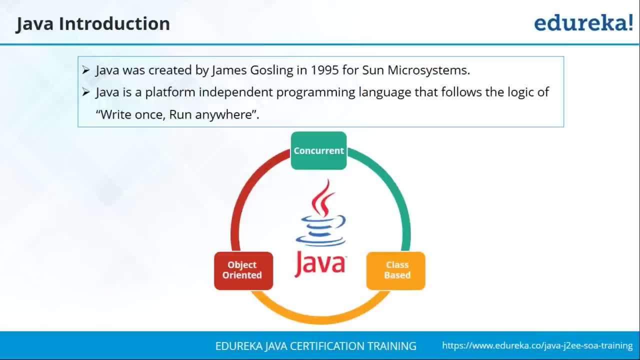 to perform on that code once you've brought it to a different system as such. Now there are mainly three key features of Java, So Java follows a concurrent approach. Now, when I talk about concurrency, it basically means that when you have a lot of statements that need to be executed, 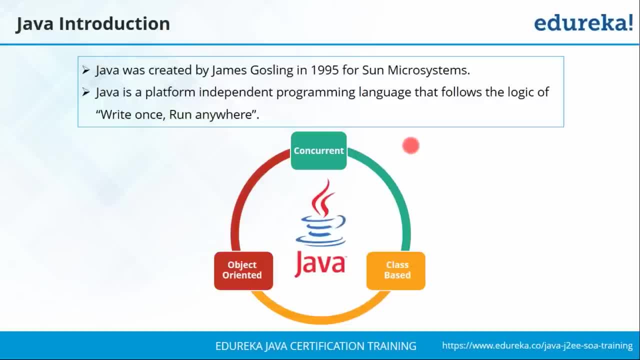 rather than executing them one after the other, you can concurrently execute them and thereby increase the overall efficiency as well, So this saves you a lot of time as such, And this can be achieved using Java. After that, Java follows a class-based approach. Now here. 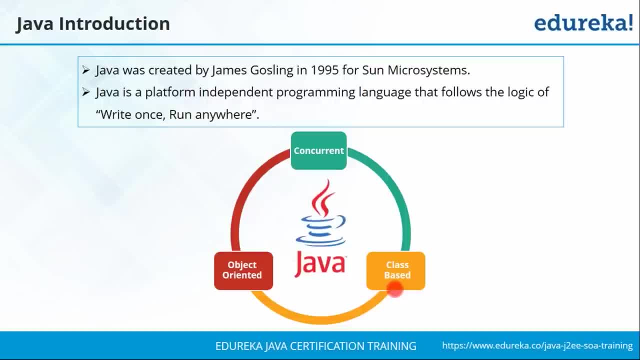 when I say class-based approach, it basically means that everything that you're going to be writing as part of your Java code, it is going to be present inside a class. Now don't worry too much about what a class is or how it is going to help us. We'll be talking that towards the later. 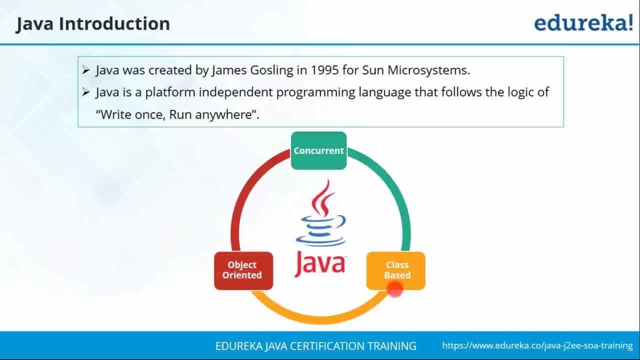 half of the session. but just understand that every code that you're going to be writing is going to be written inside a class as such. After that, Java follows an object-oriented style. So, to those of you who are not familiar with the different styles of programming, there are mainly 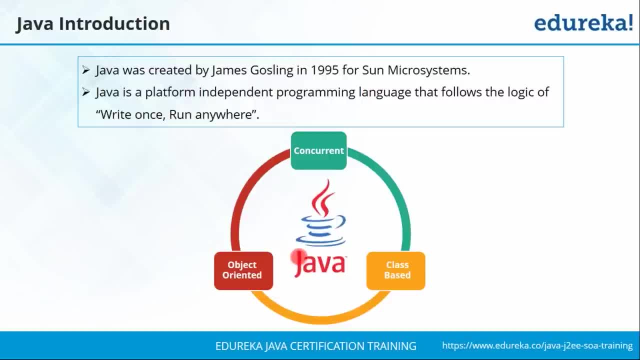 two styles that programming languages follow. One is the procedural style and the second is an object-oriented style. So Java actually follows an object-oriented style where everything is considered to be an object. So the variables that you're going to be using, the functions that 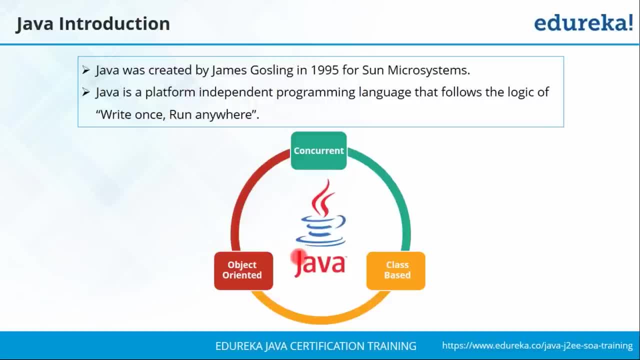 you're going to be using the operations that you're going to be performing. everything is going to be done using objects as such. So are we clear with respect to the first slide? Okay, So I have my first question here from 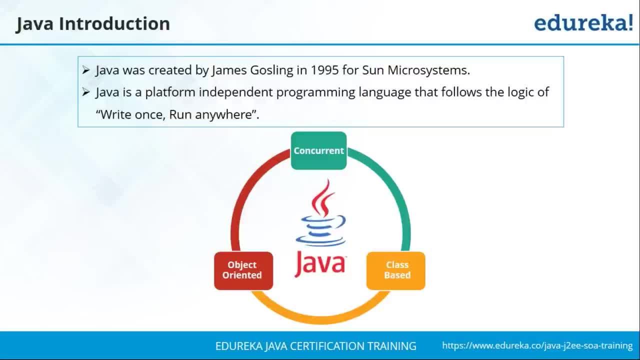 Prashant. Prashant is asking me: why is object-oriented style so important? Now, Prashant, to help you understand this, I'll just give you a comparison of object-oriented style to the procedural style that I had just talked about. Now, basically, in procedural style, what you do? 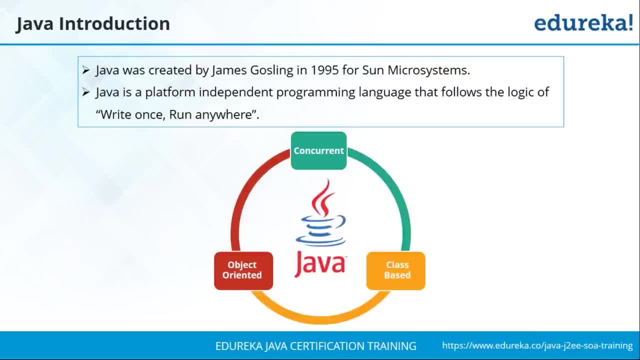 is that you follow a top-down approach, That is, all the statements that you wish to execute are written in a sequential order, one after the other, and then you go on executing one by one. So here, when you look at object-oriented style, firstly it follows a bottom-up approach. 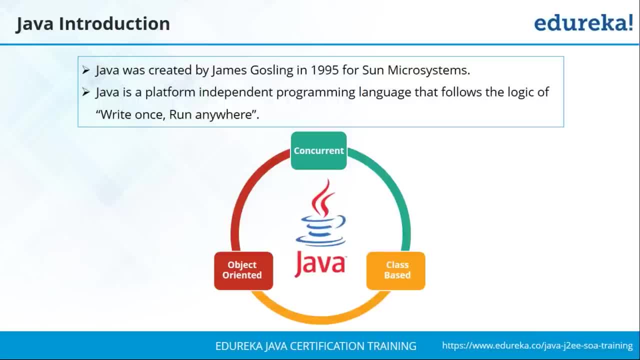 and then you go on executing a bottom-up approach. So basically, the top-down approach is that you follow a bottom-up approach. So when you look at object-oriented style- I have already mentioned you- everything here is considered to be an object. So when object, basically 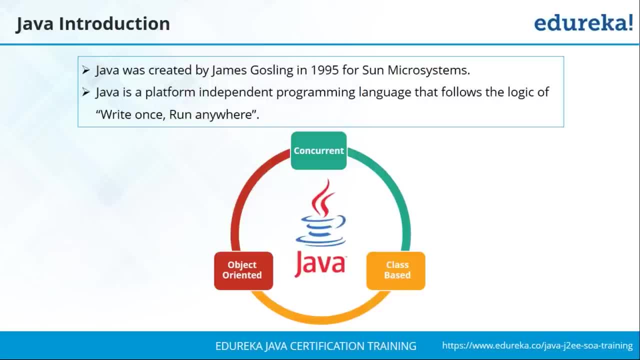 means that everything can be related into the real-world instance. So when we talk about an object, definitely it can be related to a real-world instance. Let's say you have an animal, So you would be having an object for animal present in your programming language. 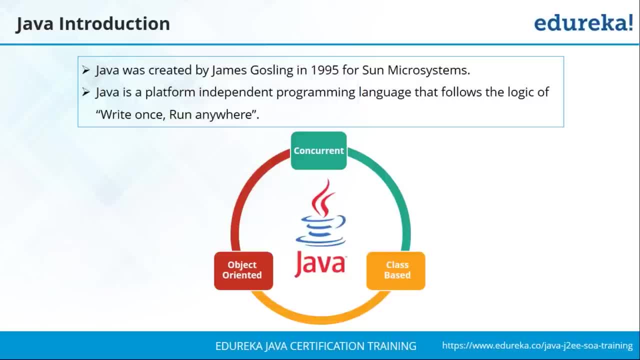 that Java also makes sure that through object-oriented programming style, your code and your data is highly secure as well. So the feature of security is highly improvised in object-oriented programming style. So I hope with that you're clear with respect to why object-oriented 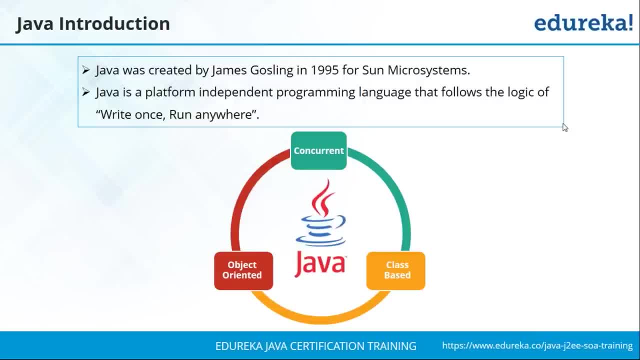 programming style is important. Okay, so Prashant wants to know some other programming languages that follow object-oriented approach. So, Prashant, the other programming languages that follow object-oriented approach is C++, then you have visualbasicnet, then you have chashnet. 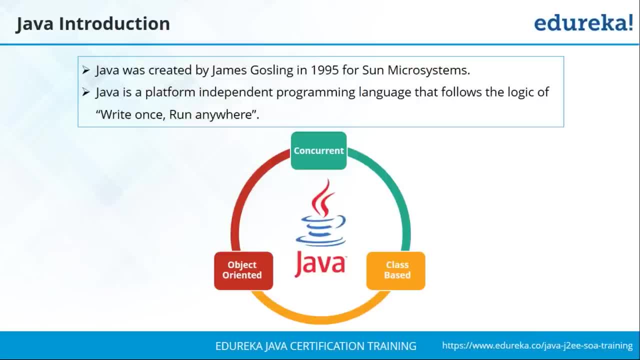 Now, chash is a good competitor for Java, So these are other programming languages that make use of object-oriented style. Are you clear, Prashant? So now that we've got an introduction to Java, let's go and answer the elephant in the room why we need to learn. 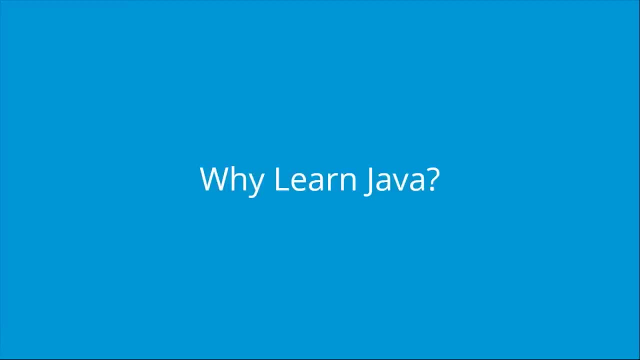 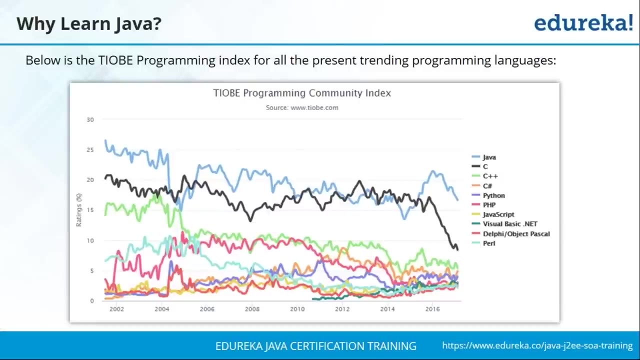 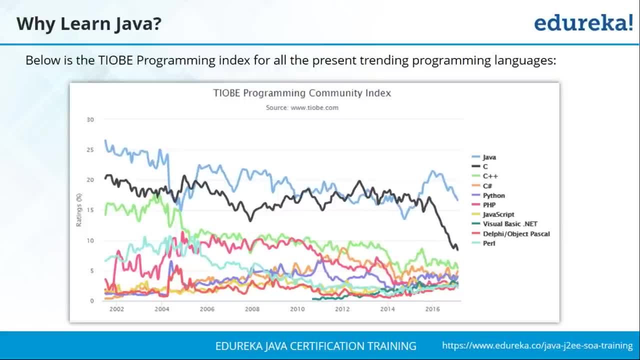 So, So, So every day. So what they have done is that they had conducted a survey based on the usage of different programming languages in the industry, as well, as they had also considered the searches for these codes across multiple domains. as such, 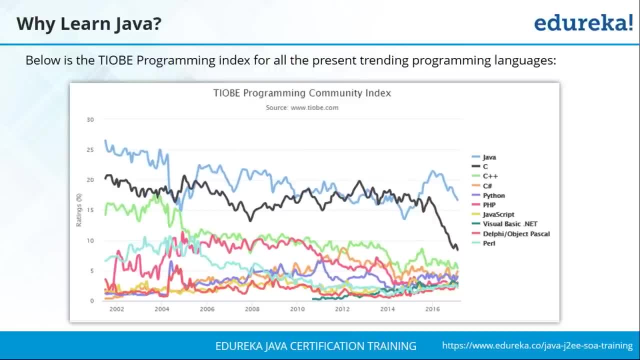 So the keyword search for these programs were taken from Google, they were taken from Yahoo, YouTube, and then this index was generated. So this index is something that is released every year and you can see here the popularity of each of the programming language. So here you can see how Java 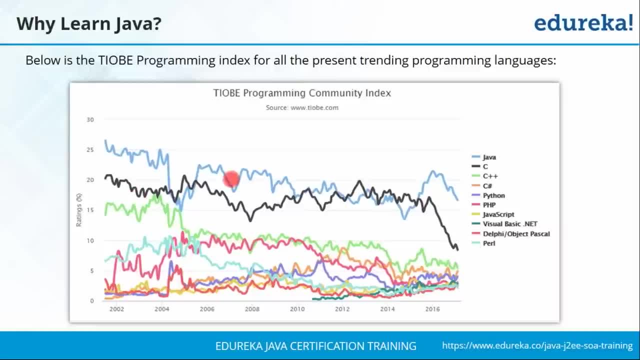 has dominated this field from early 2000s till the present 2017. as such, You can see there is no close competitor to Java as well. This in itself should give you an idea of how popular Java is and how widely it is being used in the 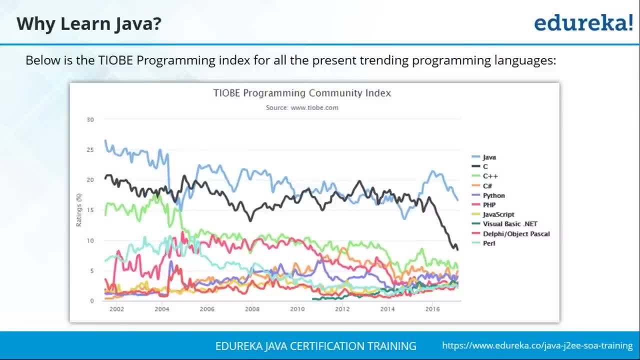 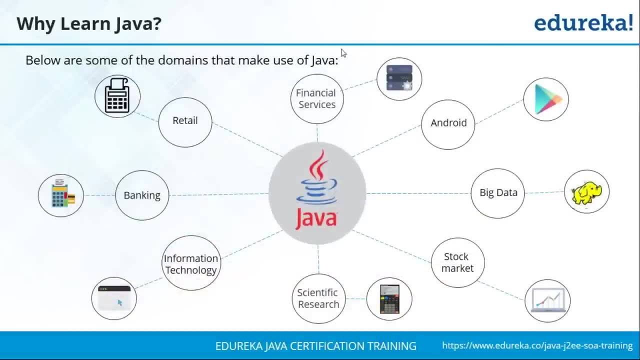 industry. Now, apart from this, let me give you a better understanding of how Java is used in different industries. So here I have just picked eight of the popular domains as such. Now, in eight of these domains, let me give you an understanding of how Java is being used in them. So when we talk about the financial service, 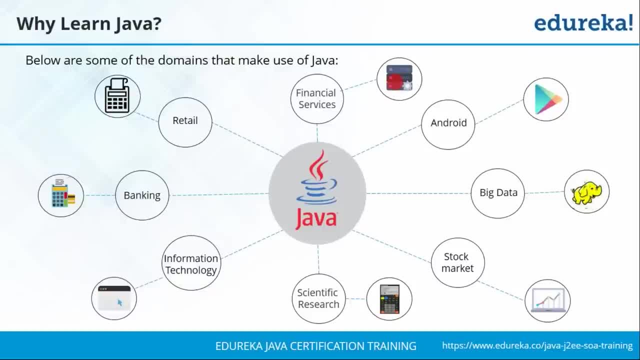 here your server-side applications will be written in Java. Now, Java is a highly preferred language to write server-side applications, and financial service domain is something that mainly uses the server-side applications. Apart from that, when you say even the retail domain, Now the billing applications that you see- 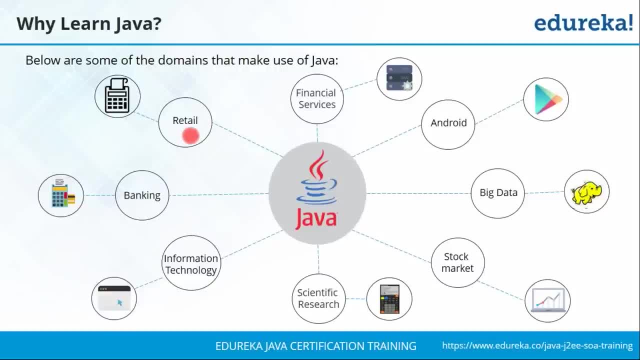 when you go to a store. this could be a normal store, it could be a supermarket, it could even be a popular outlet as well. So their retail applications billing system is completely written in Java. Apart from that, in your banking domain, 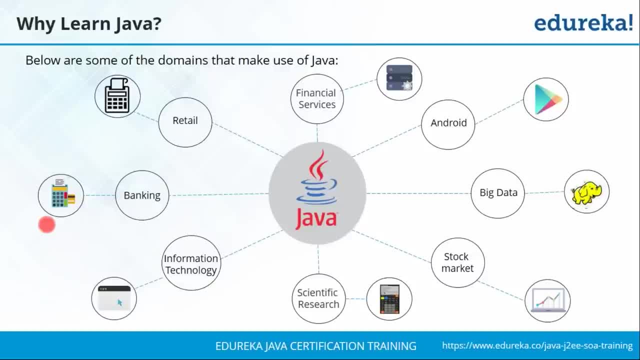 your transaction management, as well as your transactional programs, are written in Java. When you look at the IT industry, definitely you can understand. Java is a program language, So you have a lot of applications that are developed using Java, and Java is again one of the most preferred. 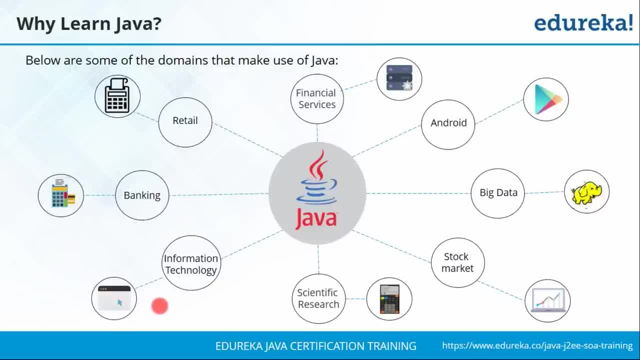 as well as the most used program language in the industry today. So a lot of applications either are written in Java or make use of some features present in Java using the Java APIs. Then, when you look at the scientific and research community there, your calculative as well as your operational programs- 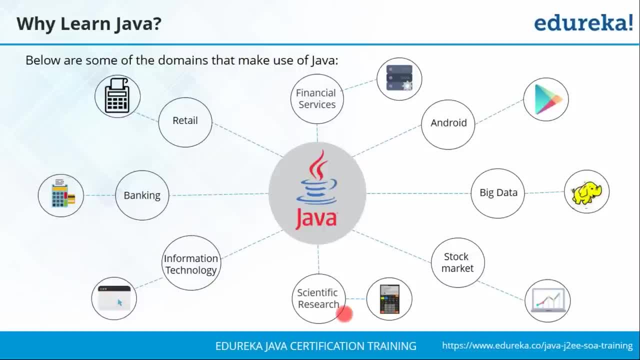 are written in Java, So, using Java, they are able to process as well as manage huge amount of data. Now again, when we say huge amount of data, we are all familiar with how scientific community deals, So they'd be using numbers that are way too big. 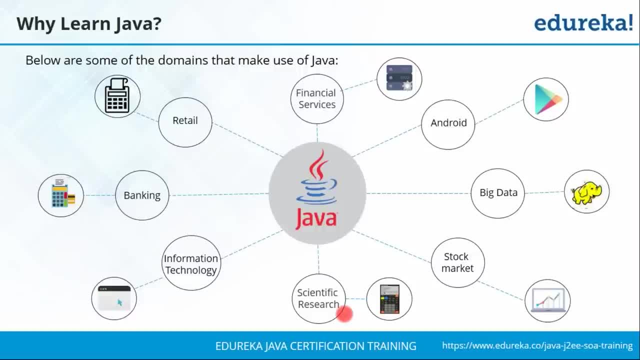 for normal applications to handle itself. So all those numbers, all those data is gonna be handled by Java quite easily. When we look at the stock market now, this is something that is quite useful. So in the stock market there are a lot of algorithms. 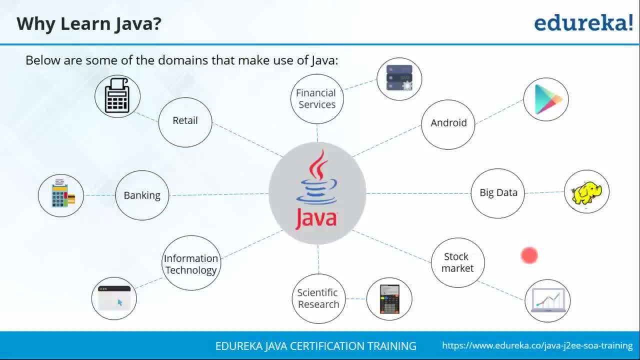 that are written in Java, which help organizations to understand better as to which company they need to make their investments as well. And when you look at the most popular domains today, it is the big data, as well as the Android domain. So here, your Android programs make use of Java. 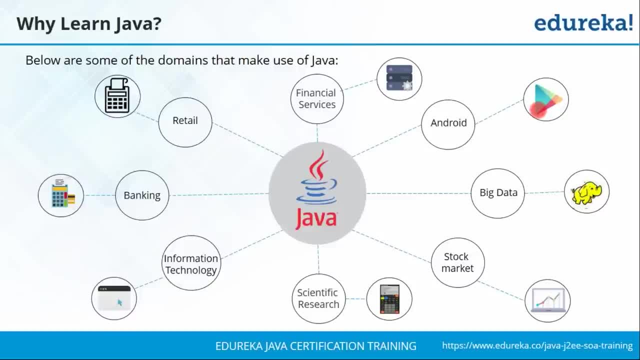 and your Android operating system itself highly makes use of Java and various Java APIs as such. When we look at the big data domain, your Hadoop mainly uses Java, and you even have a concept of MapReduce which involves Java as such. So I hope with this you've got an idea. 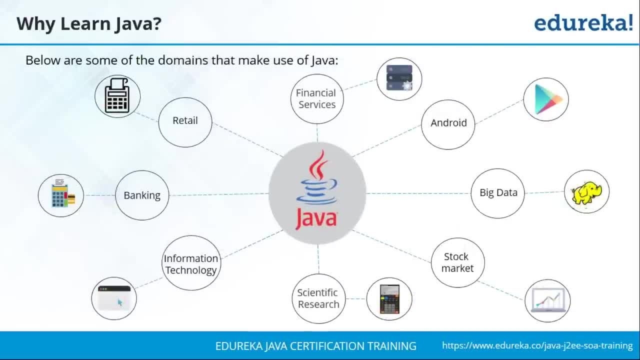 of the various domains where Java is being used, And these are not the only domains where Java is being used. I've just selected some of the few domains, But you need to understand that Java is a very big ocean, So it's not something that is just restricted. 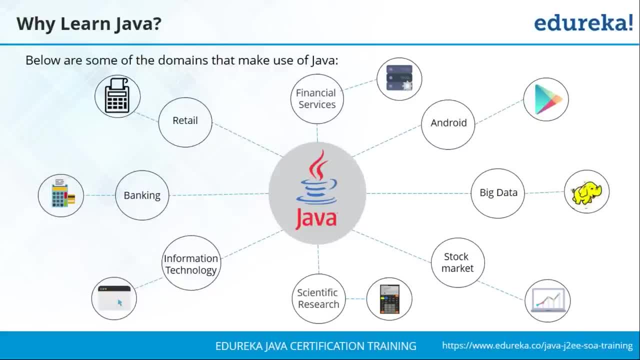 to certain domains. Java is being used across different platforms in different domains, Everywhere. you see, you can find some amount of Java present there. But when you look at it in a positive way, Java is also an ocean of opportunity When it's being used across so many domains. 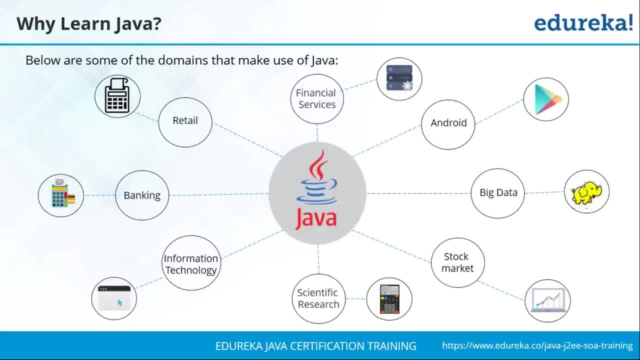 it's being. when you're generating multiple applications daily on Java, then it also brings in a good amount of job opportunities for you as well, And this is something that you all need to concentrate on. Here are some of the technologies that make use of Java extensively. 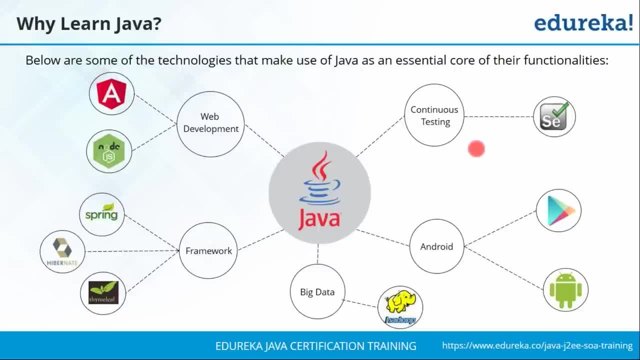 So let's start off with the continuous testing field. So when we talk about the continuous testing field, this basically means your automation testing. Now, this is something that you would have heard quite often, and in the automation testing field, Selenium is presently one of the most widely used. 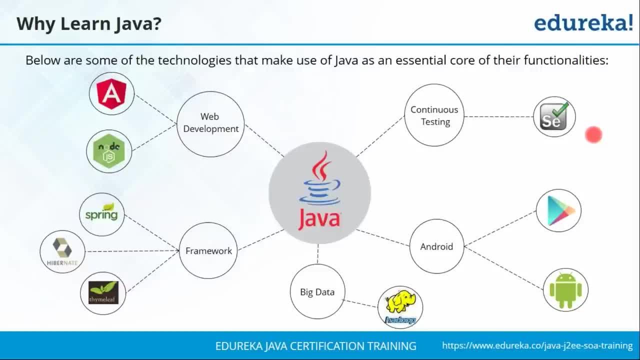 So Selenium extensively makes use of Java as part of their core programs. So you've gotta be writing a lot of codes in Java as part of your Selenium. Then again, we've discussed about Android. Here you are Android applications that you're finding. 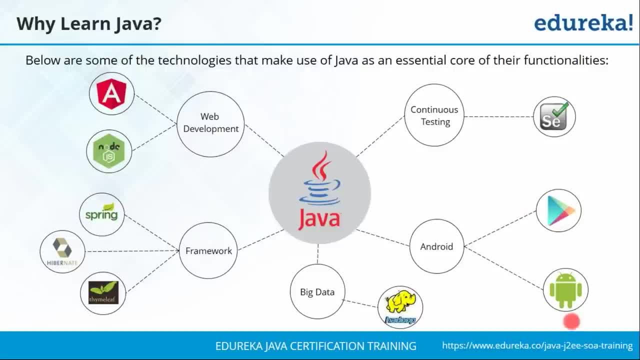 in Google Play store as well as your Android operating system, makes use of Java and various Java APIs. as such, We've also discussed about how Big Data and the Hadoop field makes use of Java as part of their core features. Then, when you look at different frameworks, 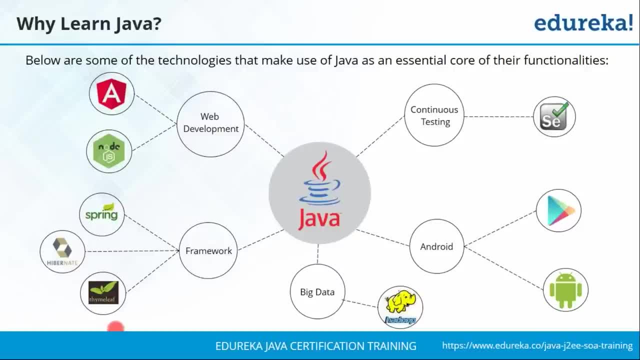 now you have Spring Hibernate Time Lives. These are some of the popular frameworks Now they also extensively used for other players like Linux or Premiere extensively use Java as part of their course. Now, Spring and Hibernate is something that we'll be discussing more in our upcoming sessions. 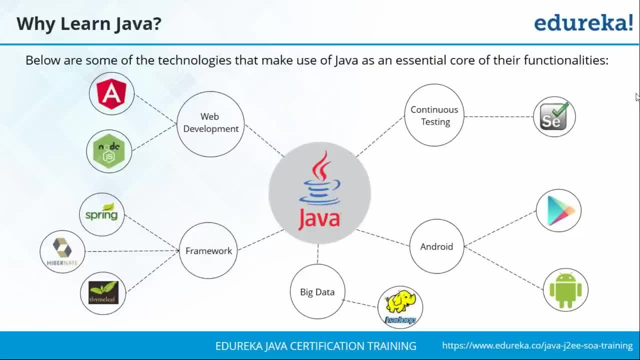 where we'll be extensively deep-diving into these two frameworks. Now again, when we look at web development field here, when you talk about these two- Angular as well as Nodejs- so these are basically scripting languages Here. what you're gonna be doing. 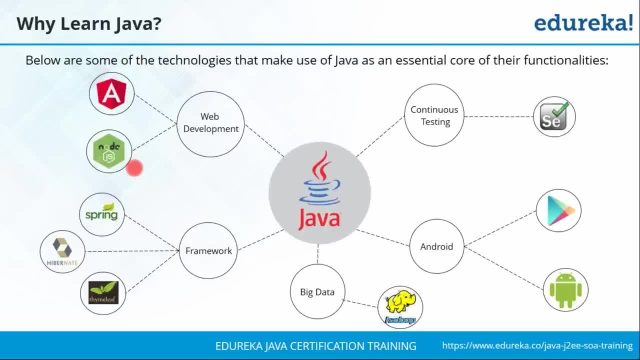 is that you're gonna be using JavaScript extensively as part of their core as such. Okay, so any questions still here. So I have a question here from Barath Barath is asking me: what is a framework? So, Barath, a framework basically is a structure. 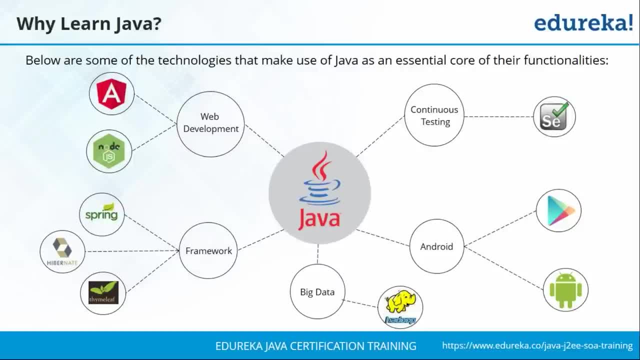 that you'll be following for developing your applications. So once you have a structure, you get an idea of how the application should be developed. And again, Spring Hibernate are some of the most popularly used application frameworks across the industry. 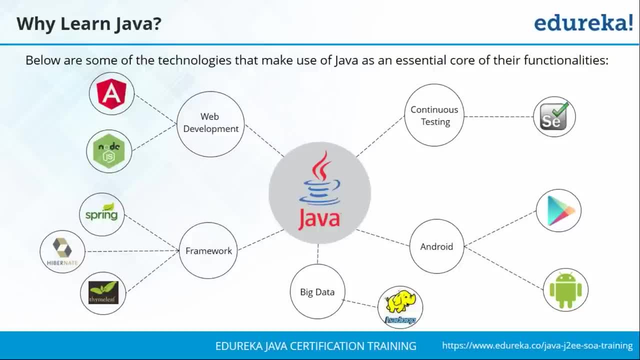 So when you have to develop an application, you will be following these frameworks to have a standardized structure for your application. So are you clear, Barath? Okay, so Barath is clear. So any other questions? Okay, so Divya says no. 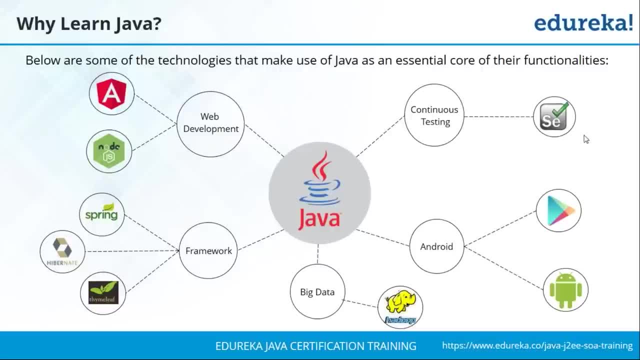 Arun says: no, Anna is clear. That's great to see guys. So again, I'd like to remind you at any point. if you're not clear, if you do have any questions, you can put it across in the chat window. 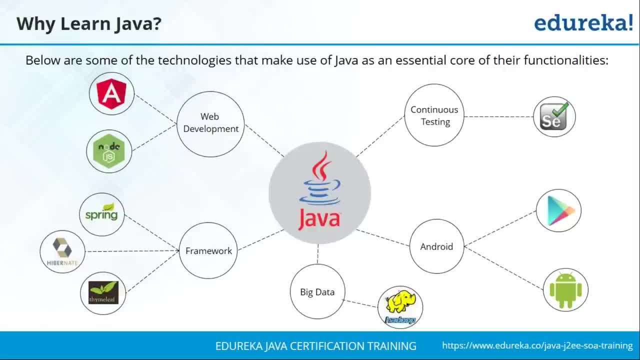 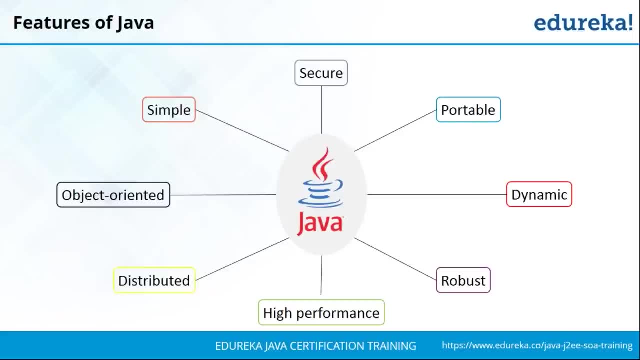 so I can help you clarify it then. and there itself. So let's move forward and talk about the various features that Java has to offer. Now, when we talk about the features of Java, this basically is also called as the buzzwords of Java. 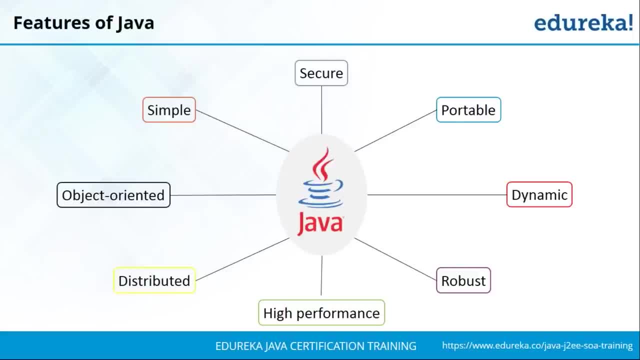 So these are the most essential features which have made Java the most popular programming language of the industry today. So we'll be talking about each of them one by one. Let's move forward and discuss that. So the first feature that you'll be discussing: 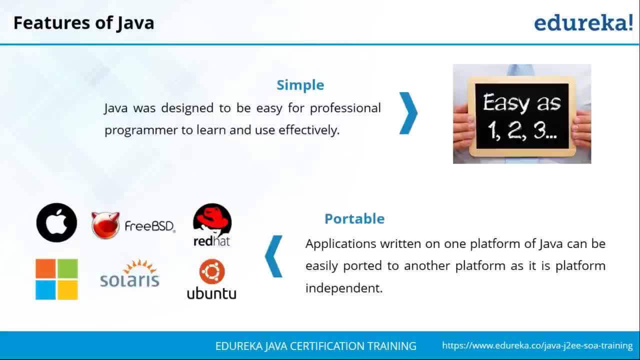 is Java is simple. So when we say Java is simple, it basically means that anyone can learn Java and it is very easy for programmers to use it and make their code highly efficient as compared to other programming languages. Now, after that, we have the portability. 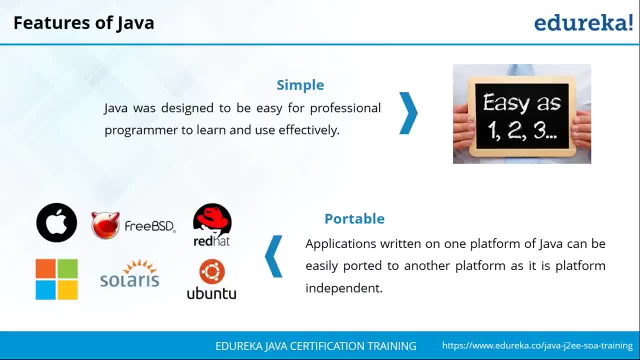 So I've already discussed the same with you in the start. Your Java application, once it is written, can be executed anywhere. It can be across multiple platforms. it could be across multiple operating systems. they could have separate configurations, but again your Java program would not have any problem. 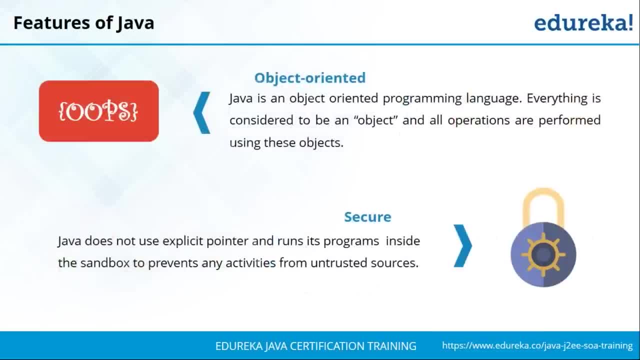 in executing across these platforms. After that, Java follows an object-oriented approach. We've already discussed: everything in Java is considered to be an object and every operation that you're going to be performing is through these objects itself. Now, when we talk about the security feature of Java, 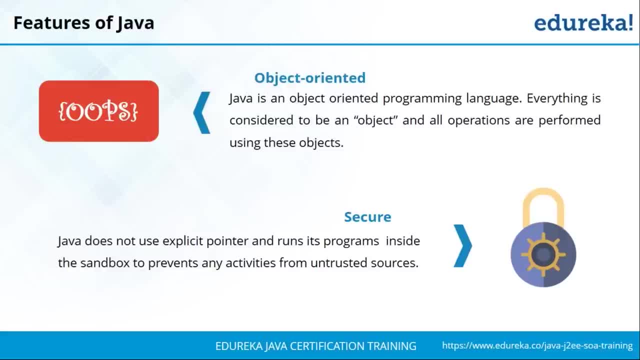 Java does not use the concept of pointers as well, So if some of you are familiar with C++, there's this concept of pointers, which basically means you're pointing to a specific memory location. So this is something a lot of programmers face hassle in. 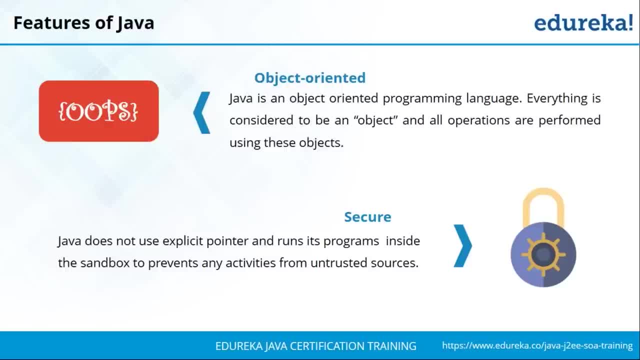 So that concept is completely removed from Java as well. Now, apart from that, your Java virtual machine- that is the environment in which you'll be running your Java- also checks the code whether there's any threat present or if there's any error present in it. 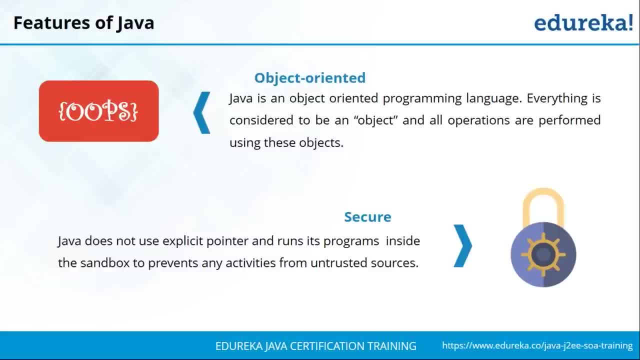 before it goes on to execute your code. Again, when you look at the web development side of Java as well, you have this concept of applet, which ensures that the security of the code is met as such. So once you've written your code, 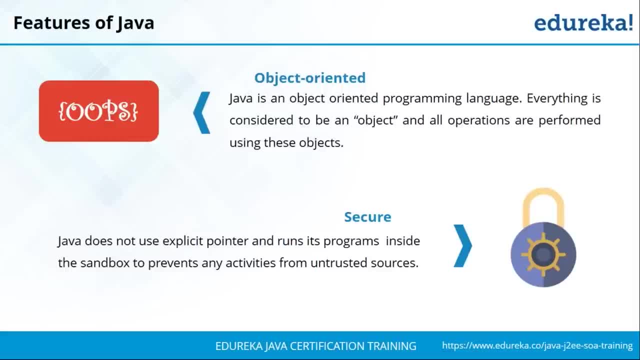 it cannot be read by any other person. What you'll be doing is you'll be giving them an intermediate file that is known as bytecode. So this bytecode is not a directly readable file. So you'll be giving them an intermediate file that is known as bytecode. So this bytecode is not a directly readable file. 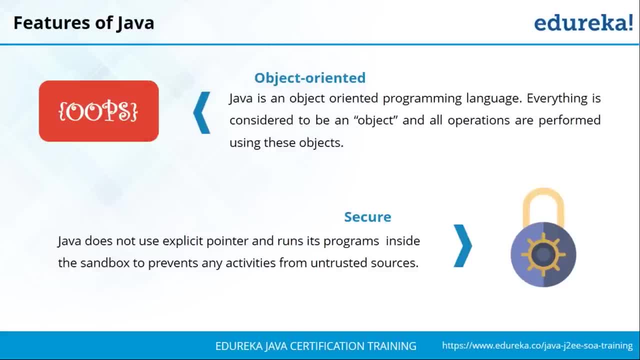 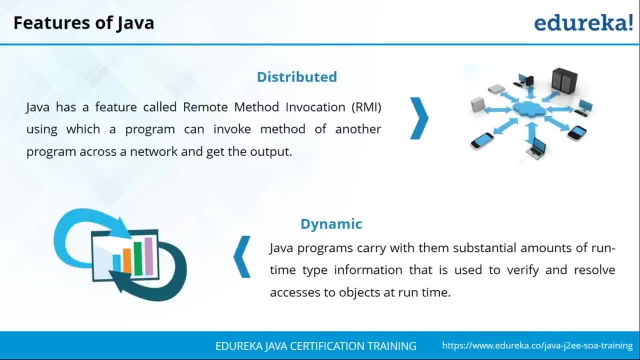 So with that, your code is also completely secure, So no one can actually directly read your source code. Okay, so when we talk about the distributed feature of Java, this basically refers to the remote method invocation. Now you don't have to worry too much about this. 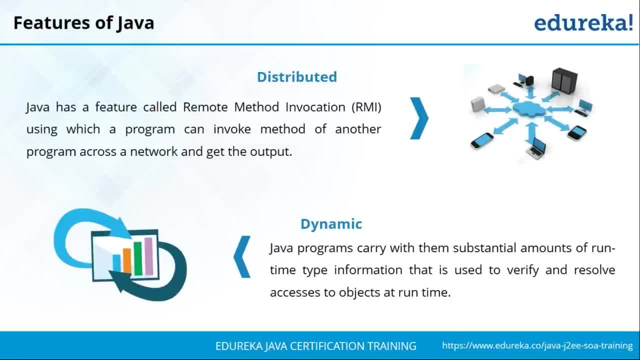 We'll be talking about this in our upcoming sessions, but I'll just give you an overview here. So you're gonna be writing a lot of programs, but they're gonna be linked to each other and not everything may be present on the same system. 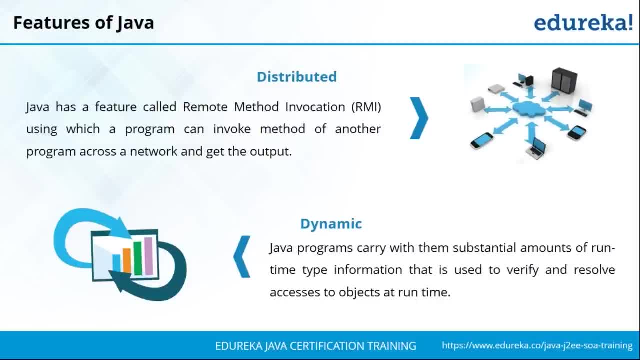 that you're executing your program. So, through the remote method invocation, what you can do is, if their dependencies are directly accessible over a network, your Java program will be able to access this. take all the necessary information that it wants, and then it'll be able to execute it. 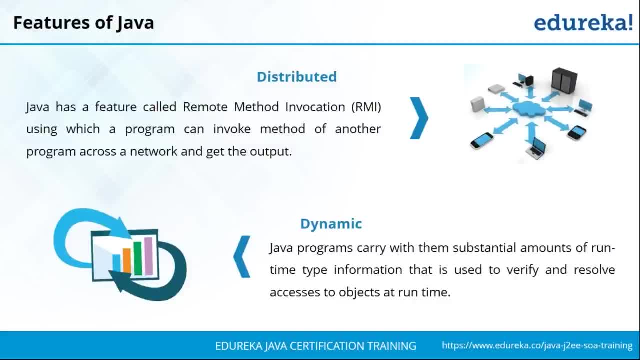 And this will seem like an easy process. Java will make it look like all the programs and dependencies are present in your same system, but it's a quite complex operation, But through Java's distributed feature, it becomes quite easy for you to achieve this. 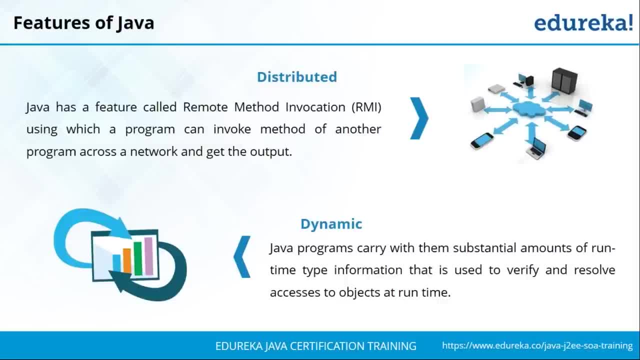 After that you have the dynamics feature of Java. So when we say dynamic, it basically refers to you know. So when we say dynamic, it basically refers to you know, it refers to the information gathering as well as the dependency association at runtime. 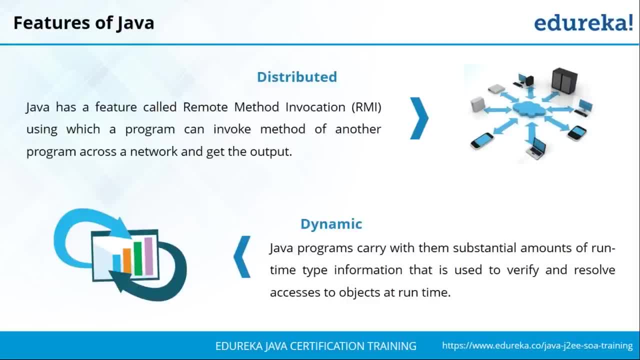 So a lot of information that your program requires, a lot of dependencies, classes or packages that your program requires is only associated to your code just before it's going to be executed as such. So there's a lot of runtime features. 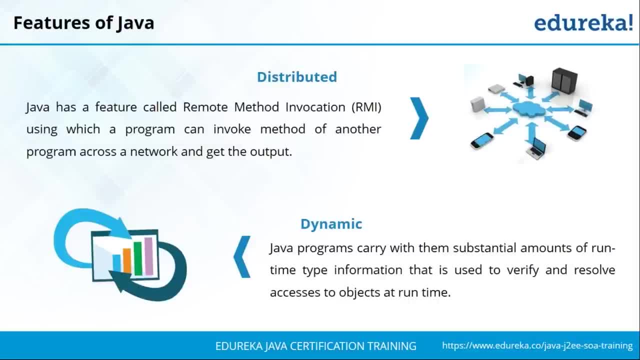 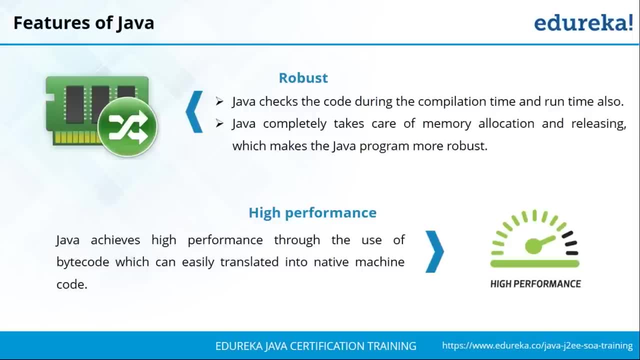 that comes into picture when you're gonna be executing a Java program. After that you have the robust feature, So this basically refers to how your Java program can be suitable across multiple environments as such. So your Java code is basically checked both at compile time as well as runtime. 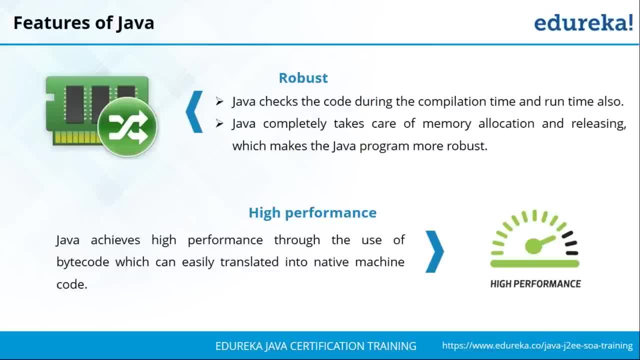 After that, your Java memory allocation. So this is something that is quite important: Memory allocation and memory releasing is done by Java in turn itself, So you don't have to worry about the hassle for allocating memory for your variable. then, once you're done with the variable, 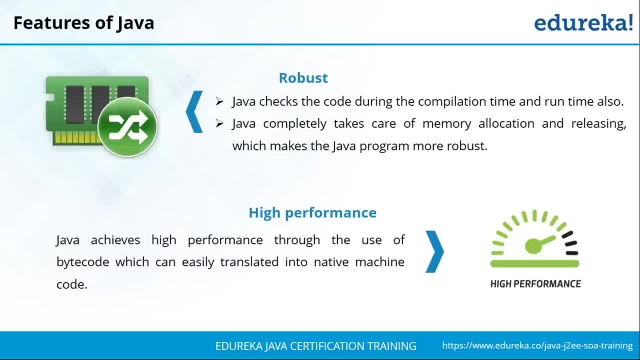 you need to release that memory. Here Java does everything for you so that completely relieves your burden of memory management. Then you have the high performance feature. now Java achieves its high performance feature through the creation of bytecode. Now the bytecode basically is an intermediate language. 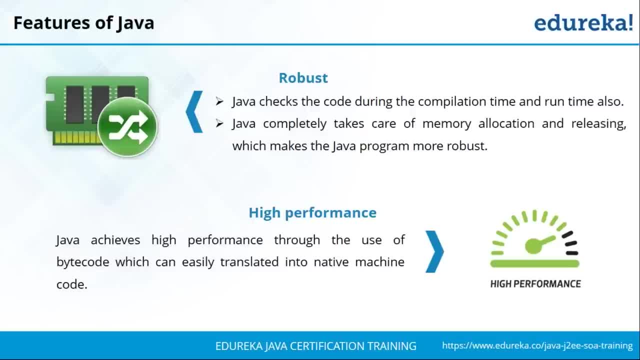 that is present between your high level language, that is, your English, and your assembly language, which is your machine language, that'll be consisting of ones and zeros. So once you've actually converted your high level language to bytecode, it becomes very easy to translate it. 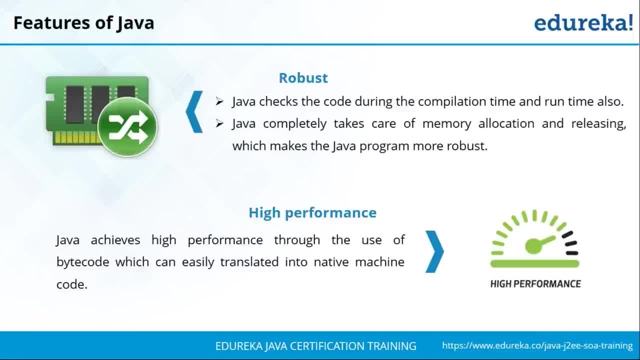 to machine level language. So once you have the bytecode, it'll be very easy for you to run it across multiple environments and it'll be very easy for you to achieve high performance as well. So any questions with respect to the features of Java. 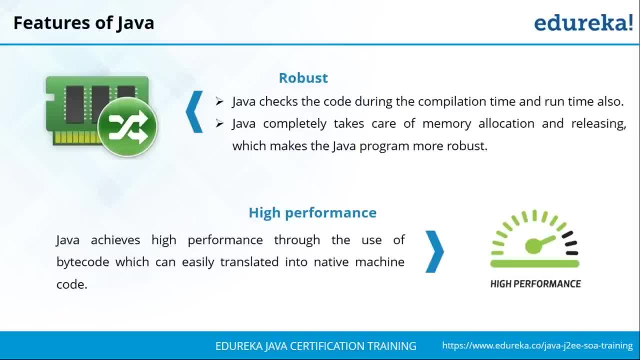 Is there any feature that you're not clear with that you want me to re-explain? Okay, Prashant says clear. Anna is clear, Bharat Divya: everyone's clear. that's great to see guys. So, moving forward, let's talk about the Java Development Kit. 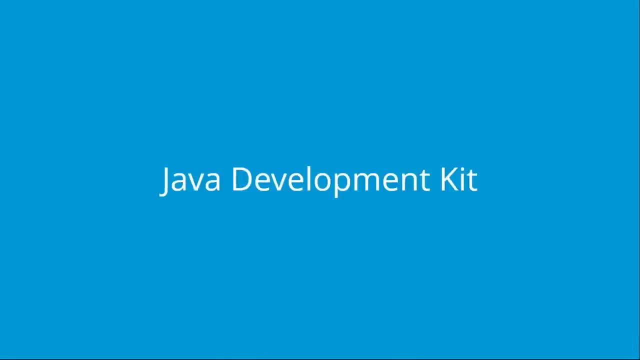 So here there are mainly three components that you need to understand with respect to the Java environment as a programmer. So Java Development Kit, you have your Java Runtime environment and you have your Java Virtual Machine. So these are three essential components. 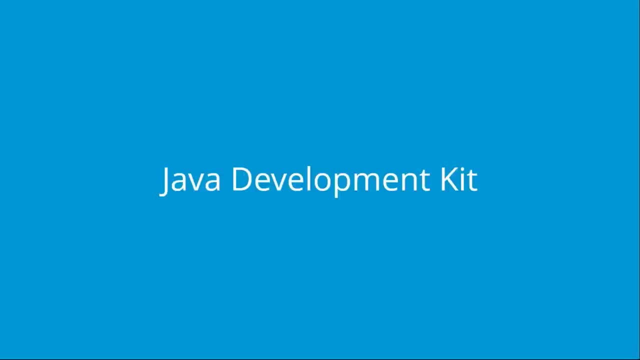 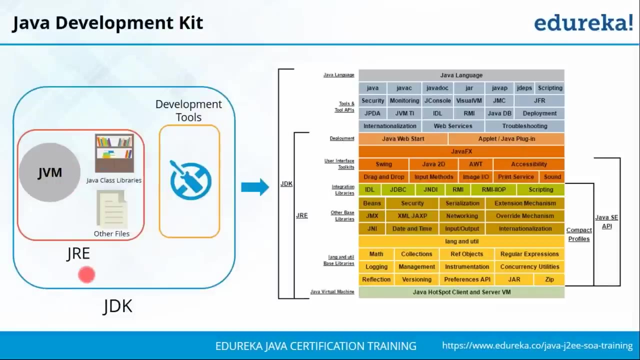 I'll just show you how these are related to each other and give you a good understanding with respect to them as well. So here are the three components that I had just mentioned. You have your Java Virtual Machine, your Java Runtime environment. 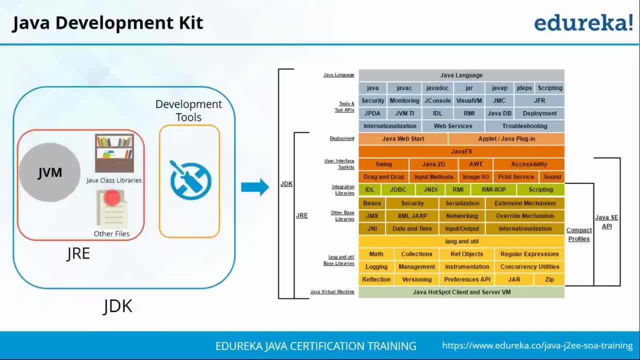 and your Java Development Kit, So your Java Virtual Machine. So, basically, this is one of the components of Java in which you're gonna be executing your bytecode. So, whichever machine has your Java Virtual Machine and you're gonna be executing your bytecode, 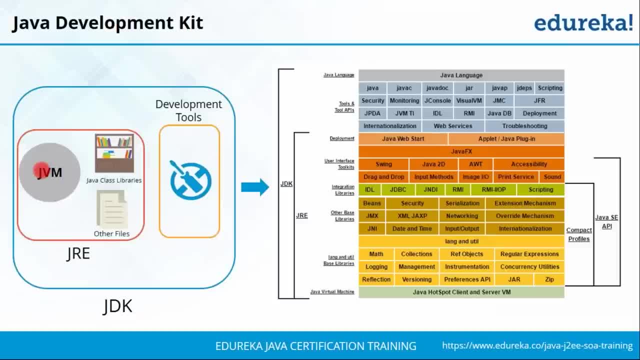 then that machine can directly execute your Java code. All you need to do for executing a Java code is that you need to have your Java Virtual Machine present there. So let's say you wanna give a program which you've developed in Java, then all they need to do is that they need to have 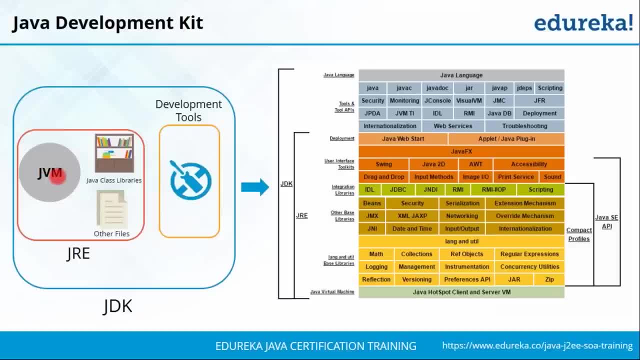 their Java Virtual Machine present in the system and then they can directly go ahead and execute that program. But then you have your Java Runtime environment. That is the environment in which you're gonna be running your Java programs. So there you're gonna be having your Java class files. 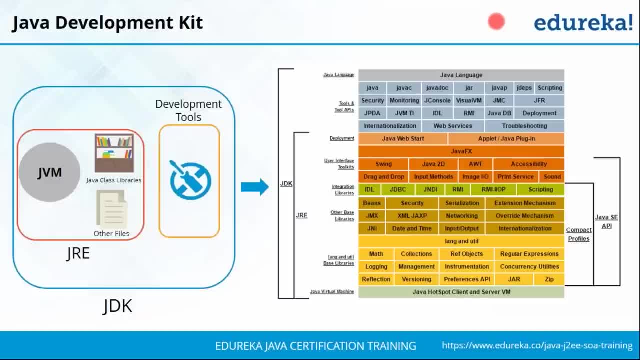 as well as your other files as such. Now, to give you a better understanding of the other files, you can look at the image here. So, basically, these are the other files that you're gonna be having as part of your Java Runtime environment. 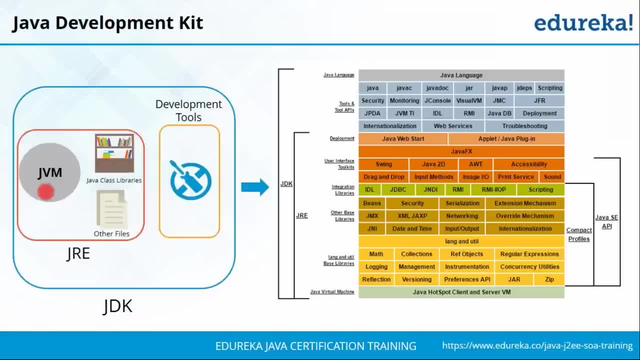 Whichever of these files are required, the JRE will directly link it to the JVM as required. So all these will be present in your JRE, and after that you have your JDK. JDK basically refers to your Java Development Environment, So this is something all developers require to have. 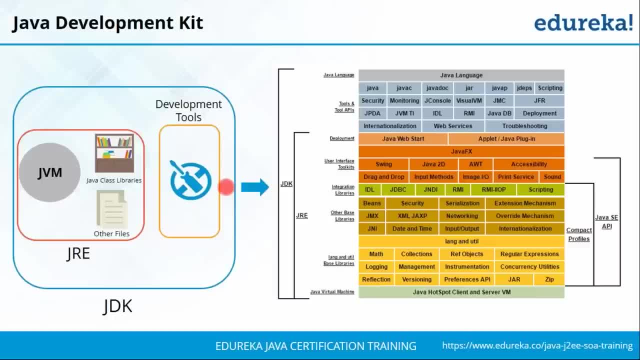 So, in case, if you wanna write your program as such or you wanna create various programs, then you need to have your Java Development Kit present on your system. So again, when you talk about your Java Development Kit, it basically has these following development tools: 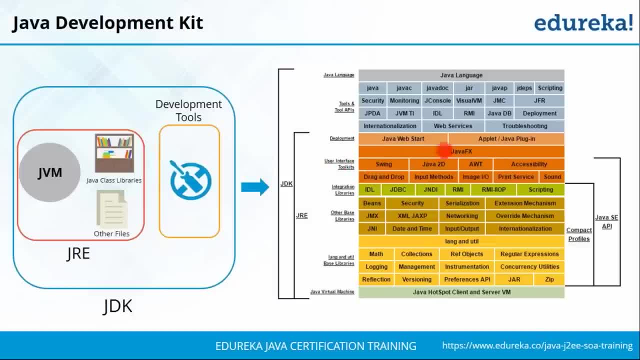 So, as you require, you can use either of these tools as part of your code. So are you clear with respect to the Java Virtual Machine, the Java Runtime Environment and Java Development Kit. Okay, so Divya is asking me. 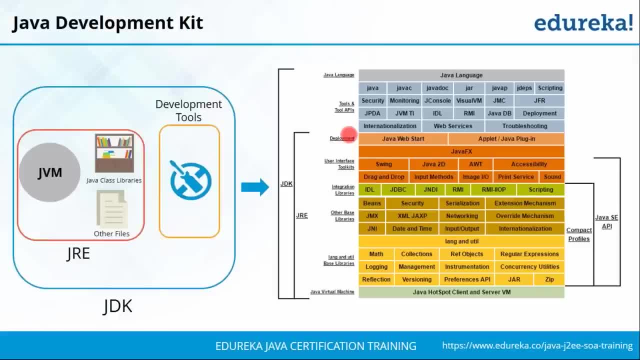 I already have Java installed in my system. Do I need to reinstall it Now? Divya, unless you have specifically downloaded and installed the Java Development Kit, I believe you'll be having the Java Virtual Machine installed in your system, So this is basically used to run the Java codes. 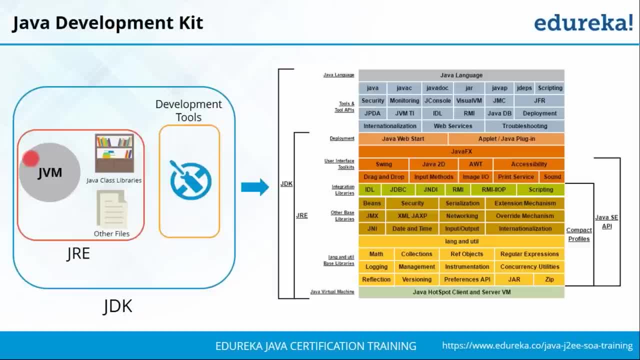 present on different browsers. So I think that is what you're referring to. Yeah, so that is your Java Virtual Machine that is installed in your system. So what we're gonna be doing is that we're gonna be downloading the Java Development Kit. 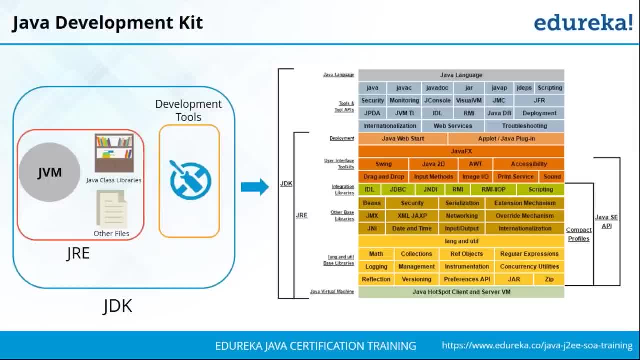 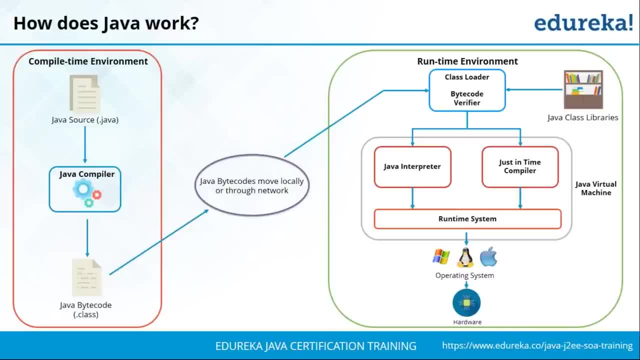 and installing it on your system. But before we go ahead and do that, let's try to understand how Java works. Now let's consider the two main environments. First is the compile time environment, that is the environment where you're going to be. 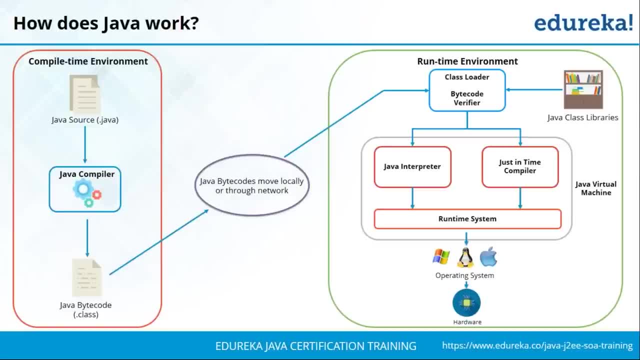 developing your Java code and then you have the runtime environment where you're gonna be executing your program as such. So we're gonna start off with our Java source code that is going to be of a java extension, So every code that you're going to be writing and saving. 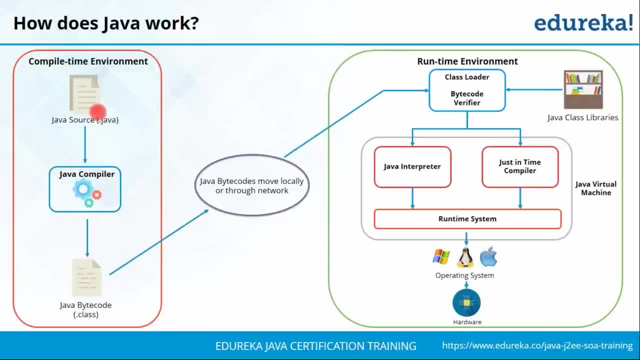 should be saved with an extension java. So this basically helps you to understand that this is a Java source code file. So once you've completed your code, then you can go ahead and use the Java compiler to compile your source code. 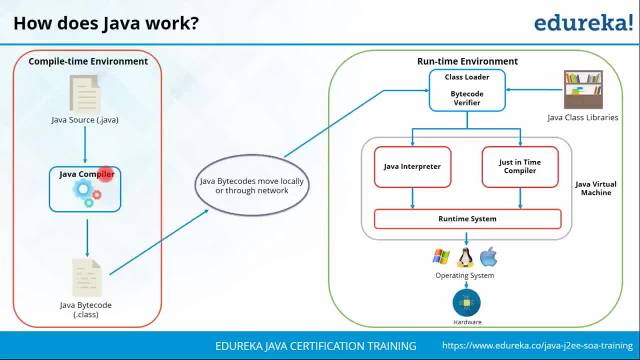 check if there are any errors present in your code and then create a bytecode. So once you've completed the coding of your application, then you've translated to the bytecode, then what you're gonna be doing is that you're gonna be moving it. 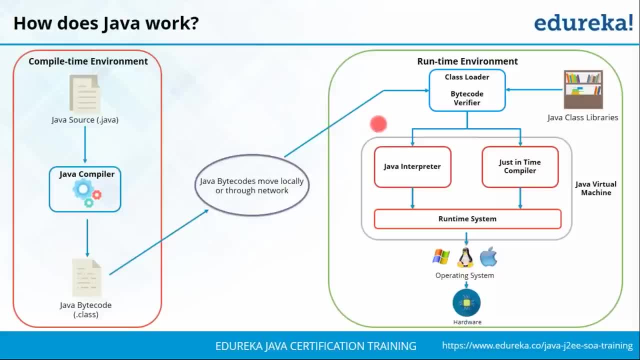 either locally or through a network, That is, you're gonna be distributing it through the internet. So once that is done, basically whoever has to run it- will follow the following process to execute it. So what happens is first is that a class loader is called. 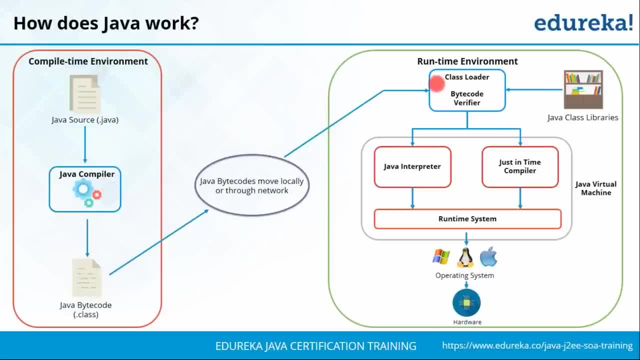 Your application may use objects from different places, So they're corresponding. details are loaded from the Java class library. After that, the bytecode is verified. So here again, when we say bytecode verification, now you're transferring your bytecode across a network. 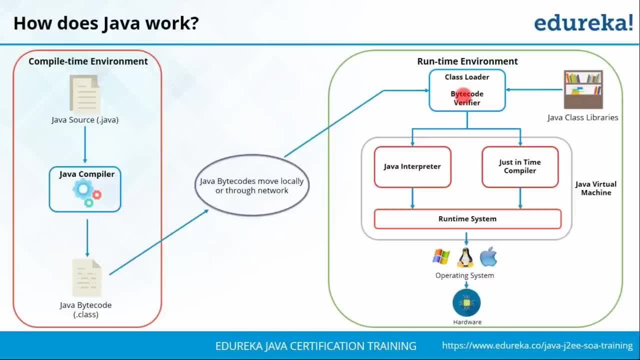 So there is a slight chance that your code may get corrupted or some virus or some changes may have happened through that transition. So your Java bytecode verifier checks if your code integrity is met and if there are any errors present in that code. So once that is done, basically, 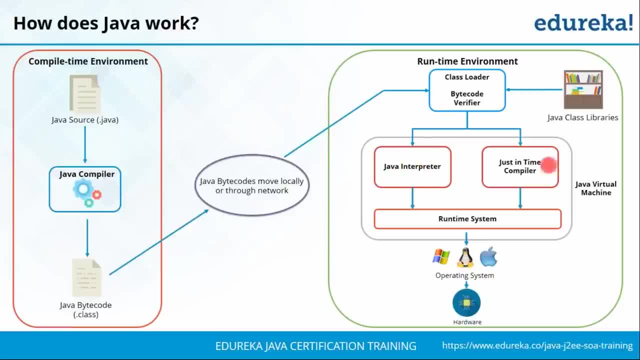 what happens is that you're gonna first send it to the Java interpreter as well as a compiler as such, So this again ensures your code has no errors. It makes it easier for your execution of the code because you're running it through an interpreter. 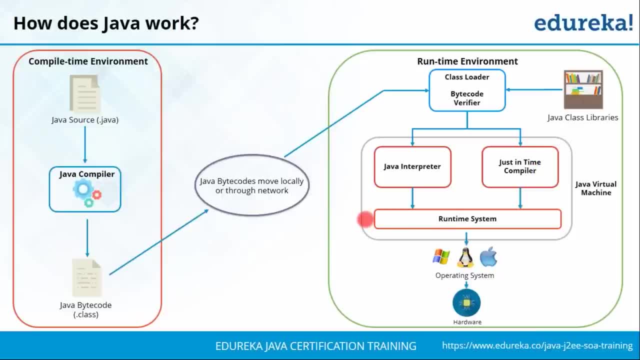 if it required, or a compiler as well, and then you're gonna execute it on your runtime system. So once you've brought it to your runtime system, then it interacts with the operating system, which in turn interacts with your hardware, where your memory allocation, data, storage. 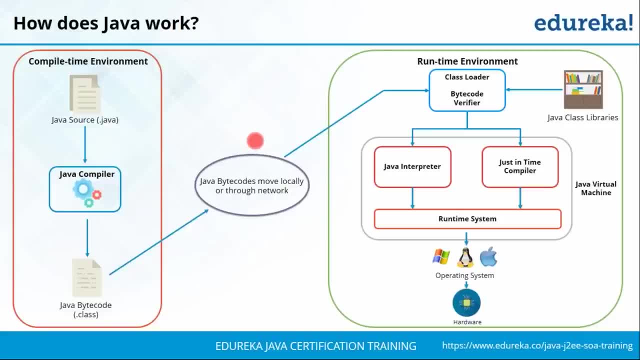 everything happens as such. So are you clear with respect to how Java works? Okay, so Divya is clear. I've got a confirmation from Anna. Bharat is also understood, Deepti Prashant. that's great to see, guys. 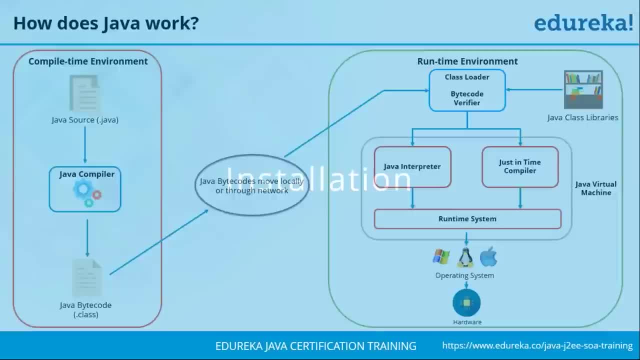 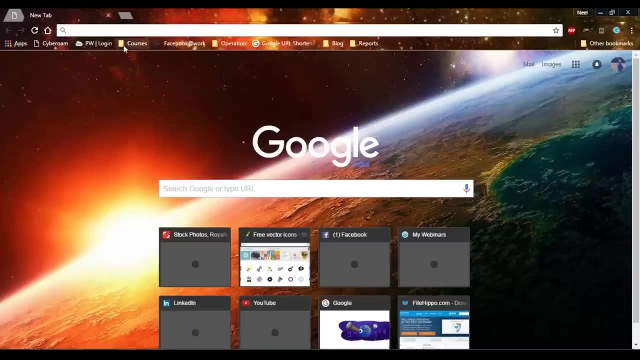 So enough with the theory part. Let's move ahead and install Java Development Kit on your system. Now to download the Java Development Kit, what you need to do is just go to your browser Here, just search for JDK download, So this will directly lead you to Oracle. 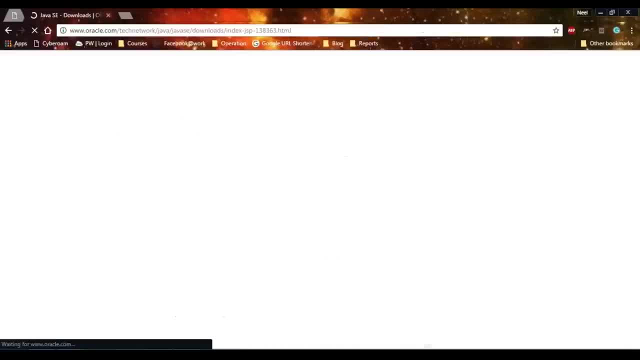 So this will directly lead you to Oracle. So this will directly lead you to Oracle. So this will directly lead you to Oracle's page where you can download the Java Development Environment, where you can download the Java Development Environment. So here you have your option. 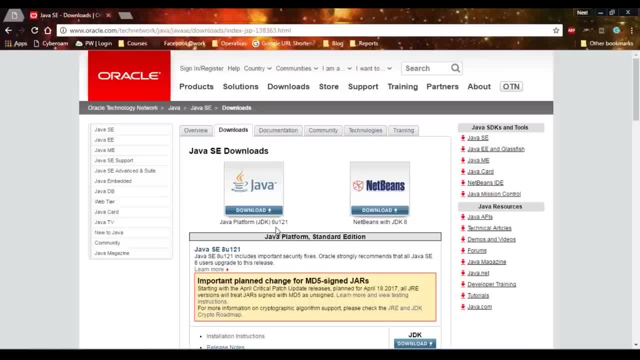 to download Java Development Kit, that is, JDK version 8u 1.2.1.. So this basically means you're gonna be downloading Java 8.. Now again to give you an idea: in the industry presently most organizations are working on Java Environment 7,. but I again recommend that you start off with Java 8 itself, because most organizations have already started migrating to Java 8.. So all you need to do is click on download here. Then you need to specify which operating system is your choice. Before that, just accept their license and then you can choose the corresponding operating. 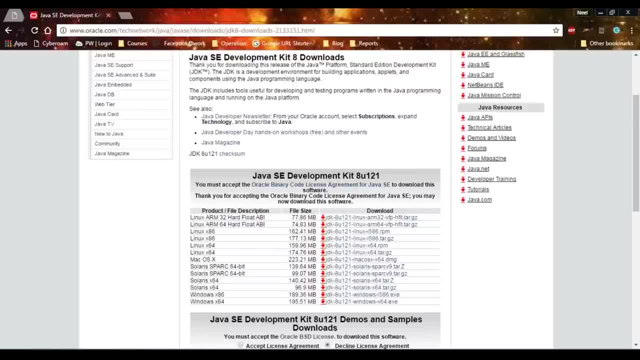 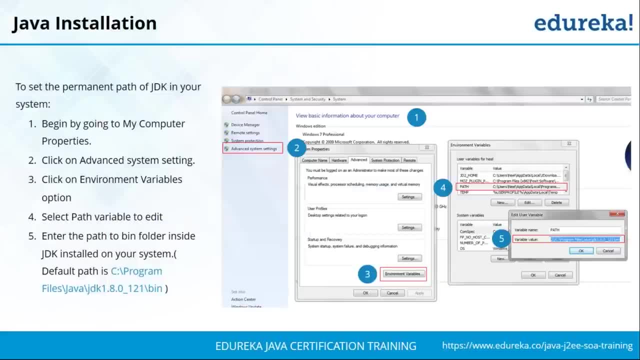 system. Now the installation of Java is very easy. All you need to do is just click next, next, next, until you're done with it. After that comes an essential process where you need to specify your Java development kits path. So go ahead and install Java on your system, and then I'll help you understand how to set. 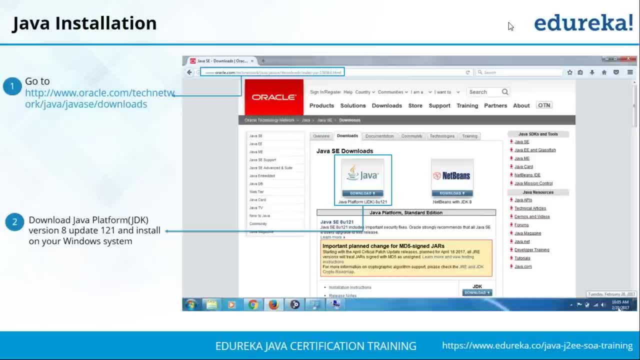 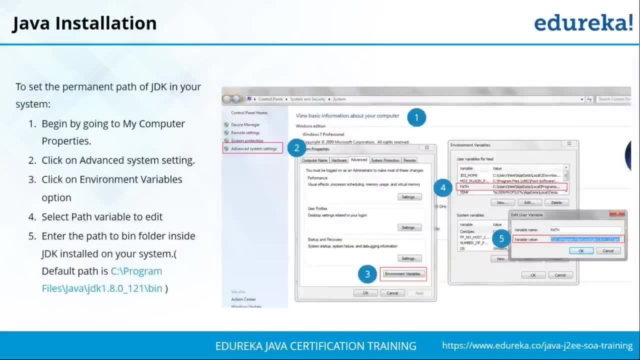 the path variable. So now that you have installed the Java JDK on your system, it's time we go ahead and configure the path of Java on your system Now. to do that, all you need to do is go to your my computer here, just right click and. 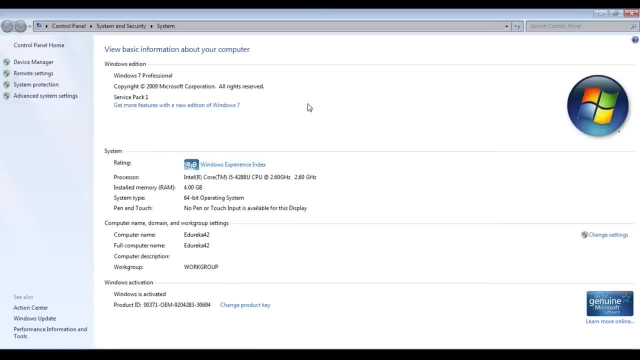 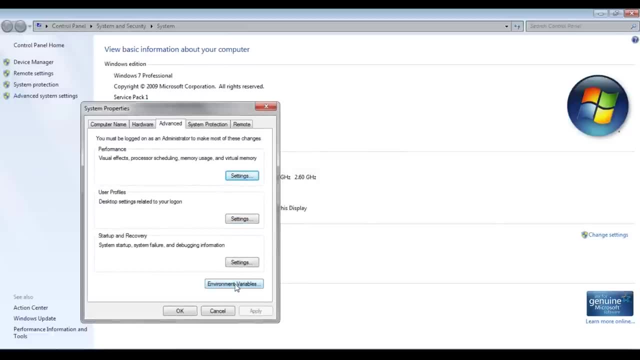 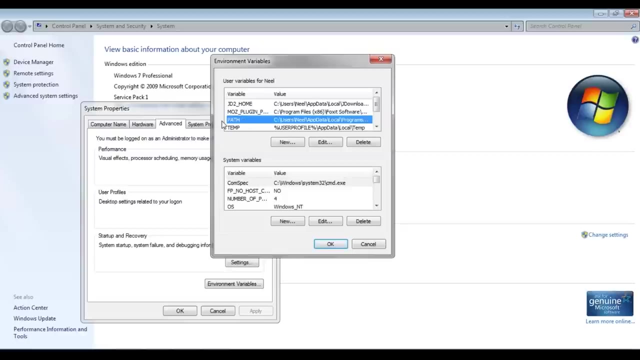 select properties option. So here you'll be getting system properties. now all you need to do is click on advanced system settings and here you have the option of environment variables. Just click on that and you will get this option for setting environment variable Now, if you do not have. 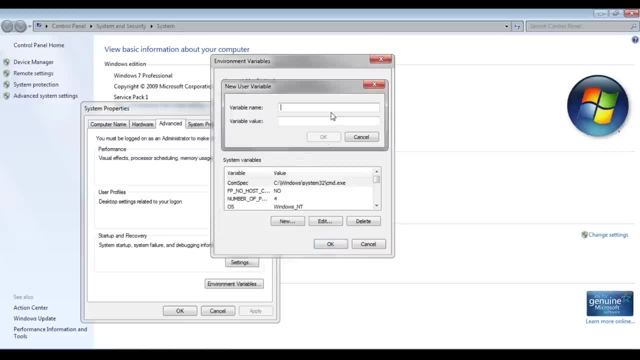 a path variable already set, just click on new and create a path variable. But if you do have an existing path value, So I already have multiple programming languages set on my system, so that path is already set. But in case if you do not have the path variable, just click on new and create. 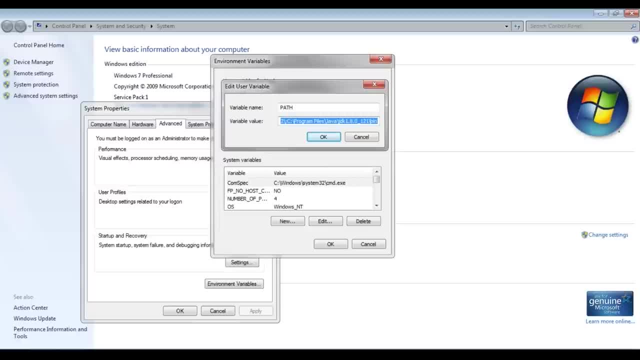 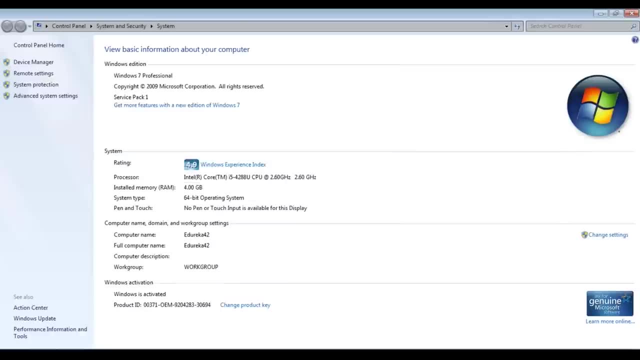 So then comes the question: what do you need to specify in this path? So here, what you need to do is that you need to give the location for your Java bin, That is, the JDK bin. So go back to my computers, to the location where you have. 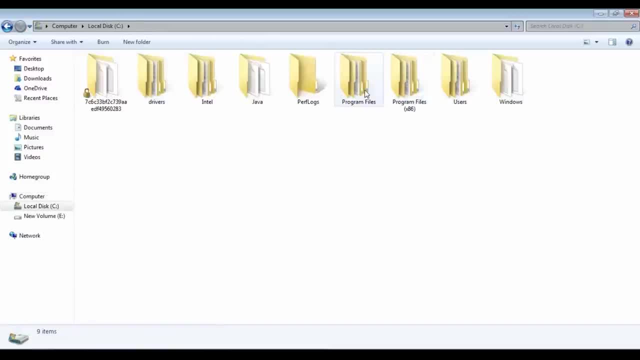 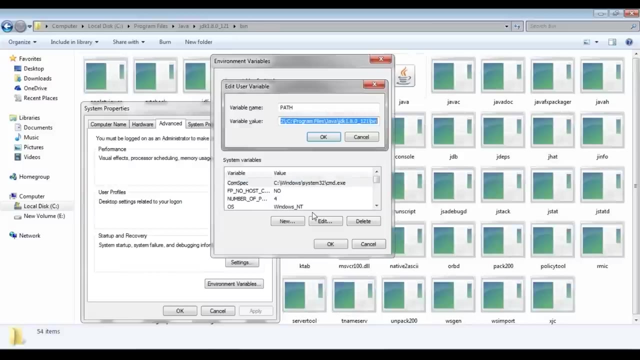 installed Java. Now in case, if you have not changed the path, it will be present in C programs, Java. and then here you have two options. you have JDK and JRE. So go inside JDK and then inside bin. So take this complete location, copy it. come back to your environment variable and specify: 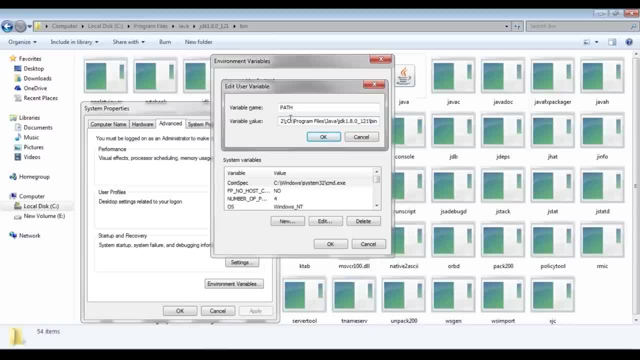 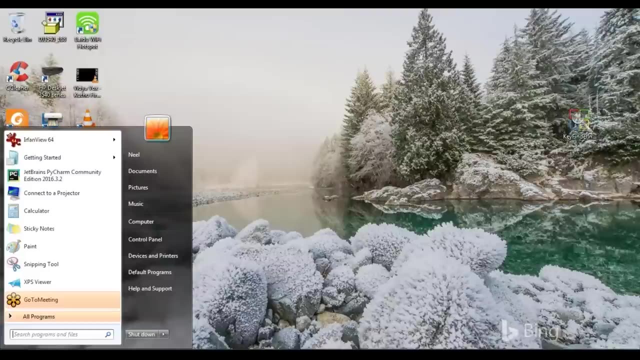 it here. So in case there is any other value, just put a colon and then put the new value. But if there is nothing set, you are creating a new variable. then just directly specify this path length, Just click on OK And then to check out if your Java path has been set, just run your command prompt. 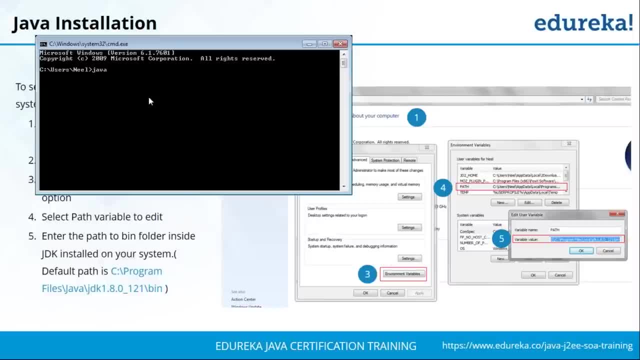 That is here. just type javac. So by this what you are doing is that you are basically checking if your Java compiler has been set. Just press on enter and, in case, if you get these values as such, then the path has been set correctly. 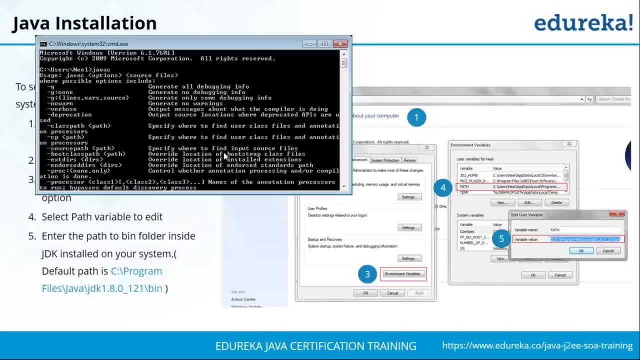 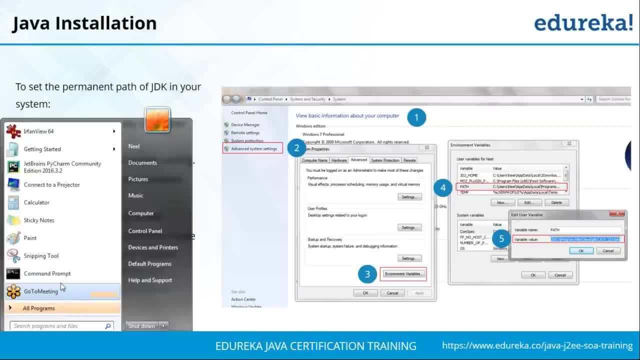 But in case if you are getting Java not found, then let me know I will be able to assist you accordingly. Okay, So now that you have all the values set, you can go back to your computer. Okay, Once you have all set your path, let me just show you how to run and compile a Java code. 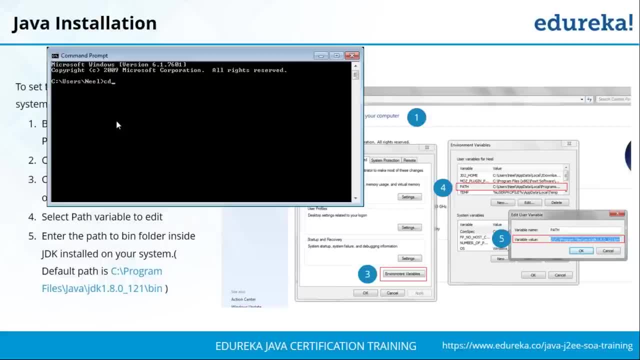 So to compile a Java code, first go to the directory where you have specified your Java. Now it's time. I'll show you how to run a Java code. So all you need to do is cd. go to the directory where your Java code is present. 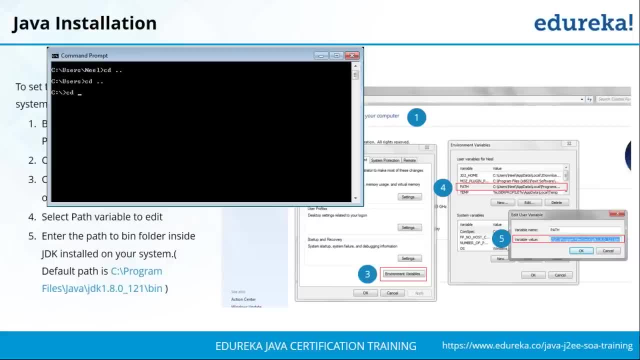 I'll run the hello world program that I had shown you earlier. So cd java. it was present inside java. Now, to compile your code, you need to specify javac, followed by the class file in which you have stored your code. So I had stored it inside hellojava and once you type this you can see a class file. 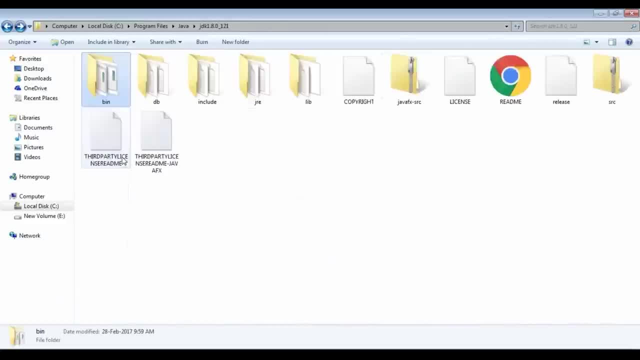 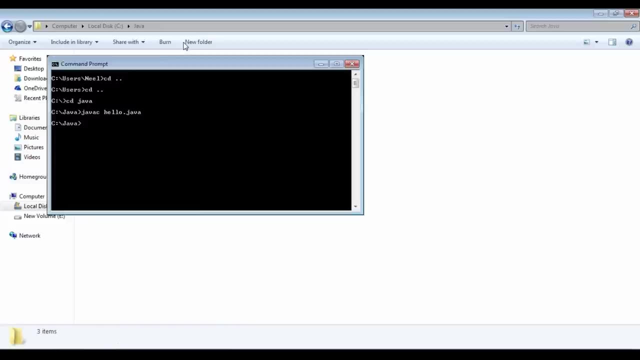 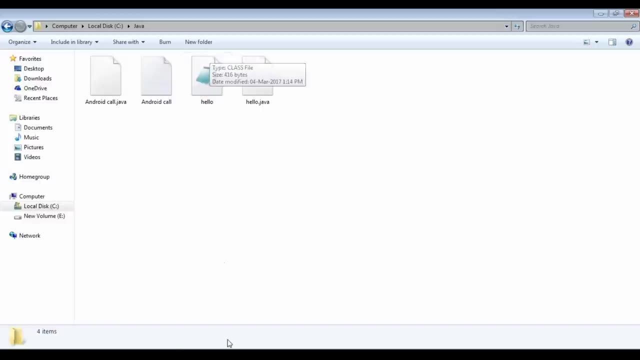 would be created there. So I already had it created. let me just remove that and show it to you again. So let me just remove this and let me just re-execute this command. So if you see here a bytecode gets created with the compiler command. 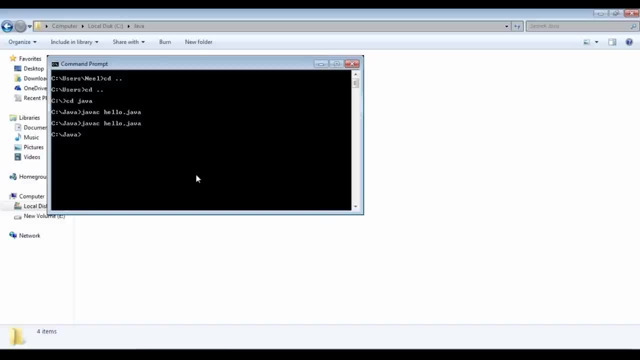 So once you've done that, it's time we execute this program. So to do that, all you need to do is specify java And then your helloexe. So once you've compiled your code, let's execute it. So just specify java and the file name. 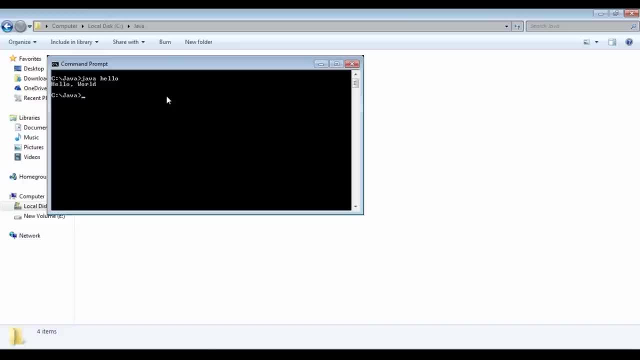 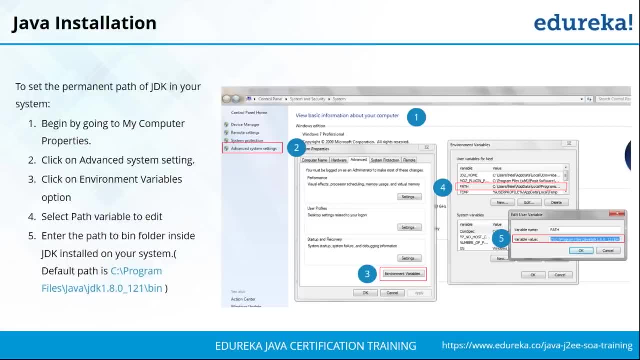 So you can see the code has been executed. But this becomes a tedious process when you have huge amount of programs that you want to execute. So, to overcome this challenge, what we're going to be doing is that we're going to be installing an IDE. 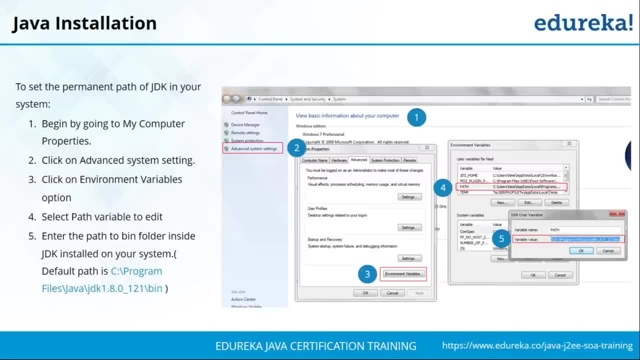 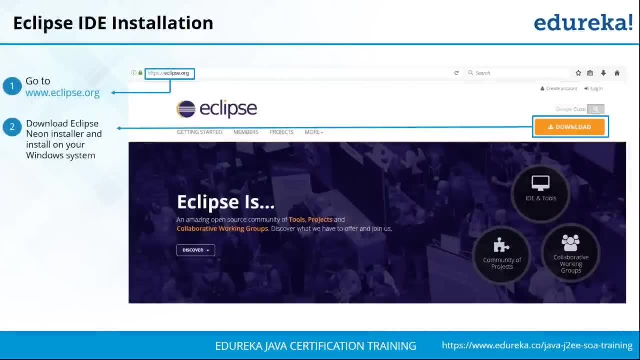 IDE basically refers to an integrated development engine, An environment where you can basically compile as well as see your code. Now the most popular IDE is Eclipse, So let's go ahead and download and use Eclipse, because this is a standard development tool that you're going to be using as part of your industry. 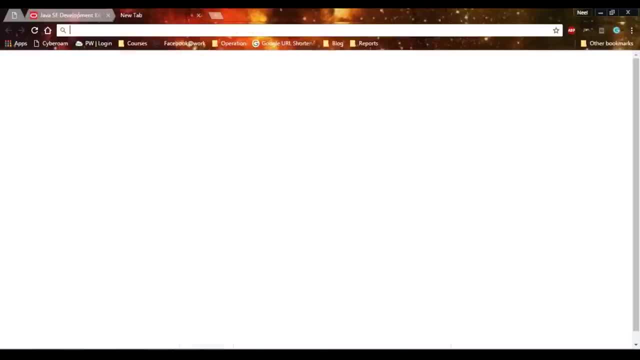 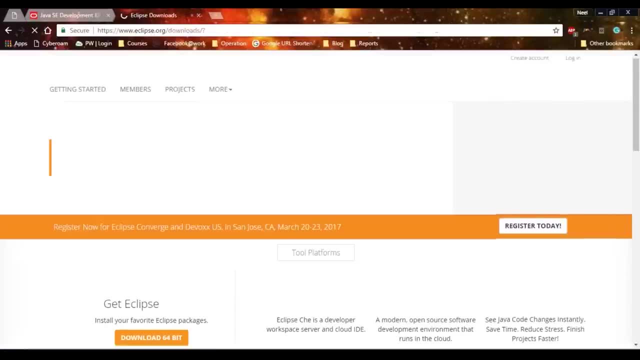 Now to download Eclipse. all you need to do is go back to your browser, search for Eclipse download, So go to the Eclipse download option, And here I recommend that you download Eclipse Neon itself. Now let's go to Eclipse Neon. Let's go to Eclipse Neon. 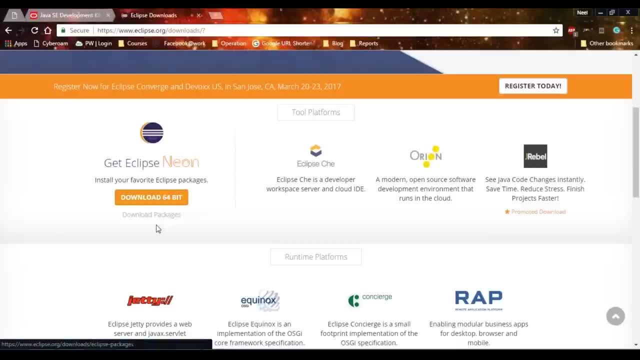 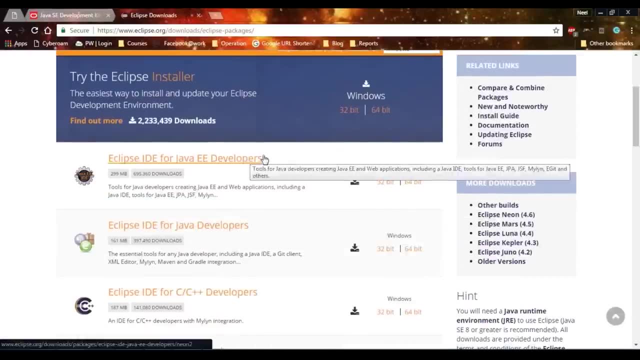 Now there's a direct option to download the 64-bit for Windows. But let's say, if you're using a 32-bit, you can go to the packages option And here you can choose the corresponding package. Now there are multiple versions of Eclipse for Java developers. 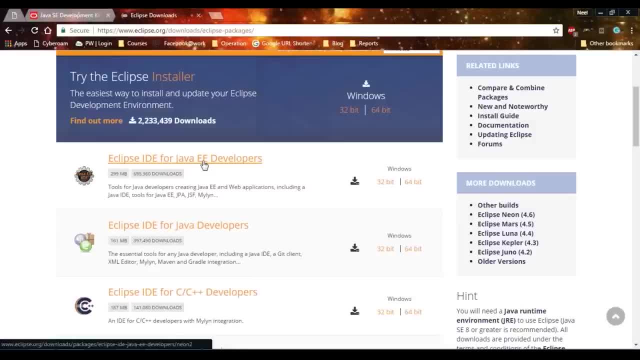 So I recommend that you download the Java Eclipse IDE for Java J2E development. So this is a complete package and it'll be very easy for you to use this as well in our upcoming sessions. So specify your system and download it. It'll directly give you a zip file. 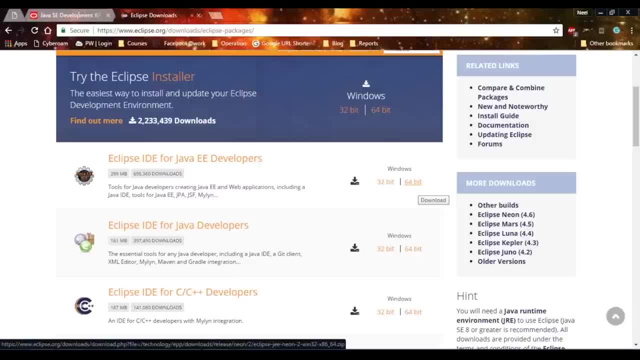 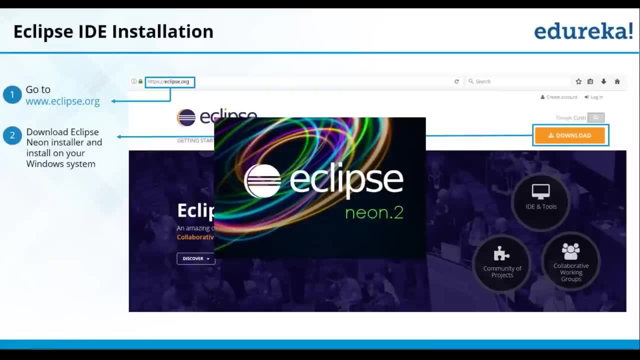 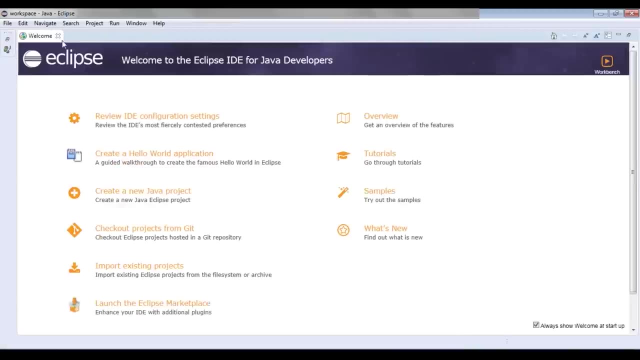 Now inside that zip file. Once you've extracted it, you'll directly have your Eclipse, which you can launch from there immediately. Let me show you how the Eclipse looks like. So this is your Eclipse IDE. So to your left, you have all your Java projects. 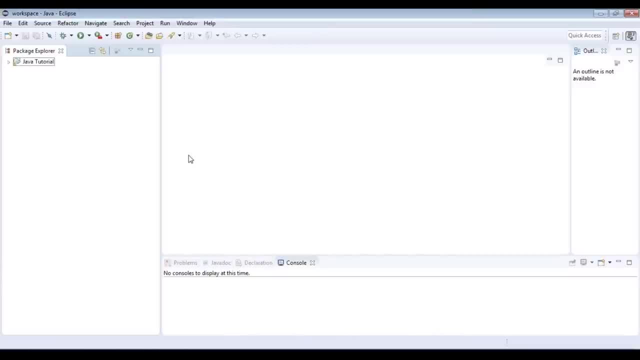 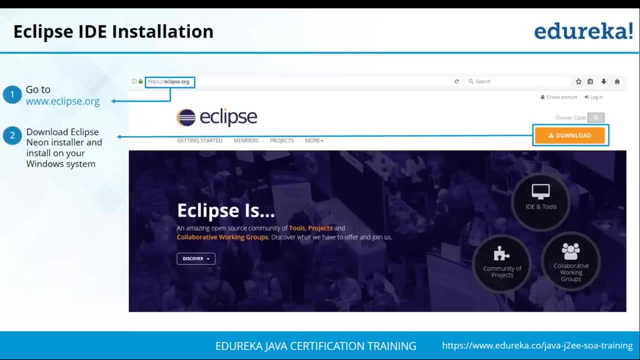 Then you'll have your code present here and this is your output feed. So, don't worry, we'll be using the Eclipse IDE in our next slide, So just hold on to that. Any questions with respect to the installation or any problems that you have faced? 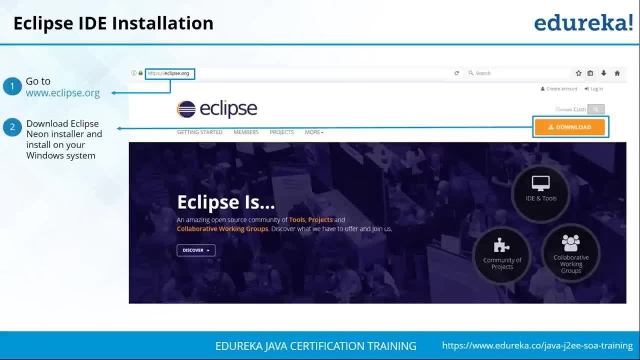 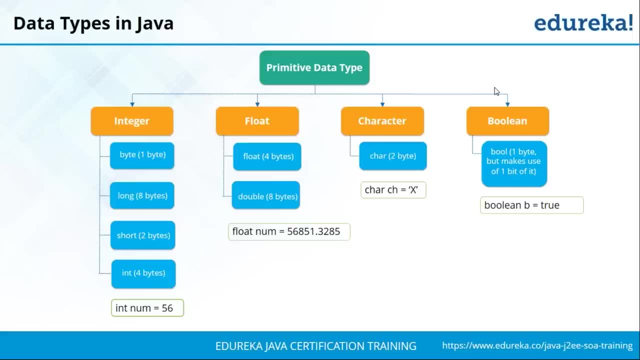 All right. So now that all of you also installed Eclipse in your system, it's time we move ahead. So we'll be discussing the various data types present in Java. So these are some of the primitive data types that are present in Java. 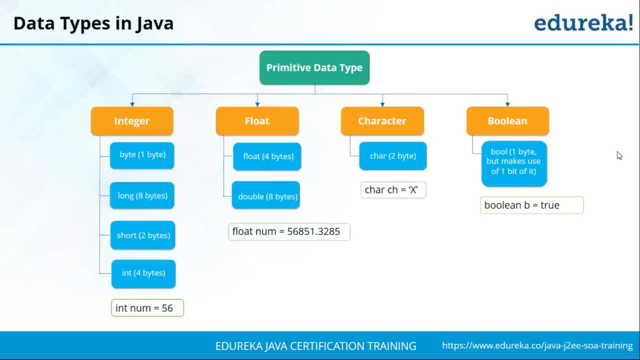 They can be mainly classified into four different aspects. So first you have your integer, then you have your float character and boolean. Now integer, basically, is used to store a numerical value. Okay, Numerical value, again, when I say cannot have decimal points. 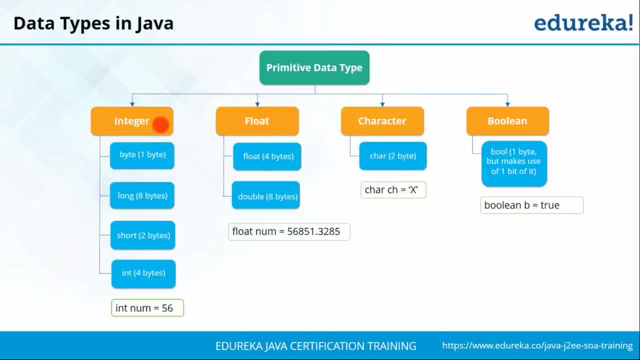 For decimal points you have float, So any numerical value that does not have a decimal point value can be used to store int. So, again with an integer type itself, you have four different types: You have byte, you have long, you have short and you have int. 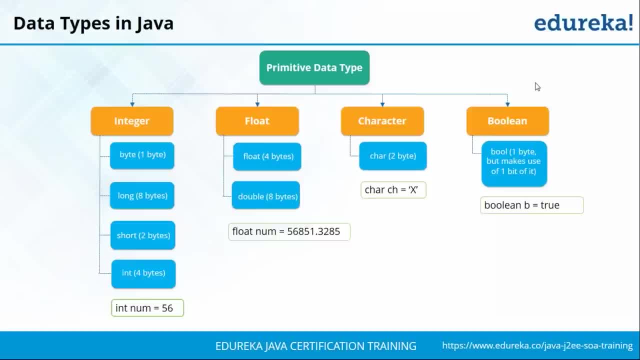 So, based on the numerical value which you're going to be storing, you can use either of these. So, to give you a better understanding, in a byte you can store a number that is between either minus 128 to plus 127.. 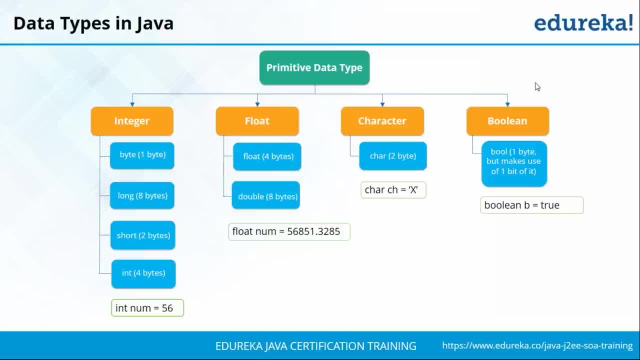 But at the same time, when you look at int occupies four bytes. So within an integer you can store a numerical value that is between 2100 crows to plus 2100 crows. So it's a huge number itself. So mostly we stick to integer itself, but again, based on your need, you can even use 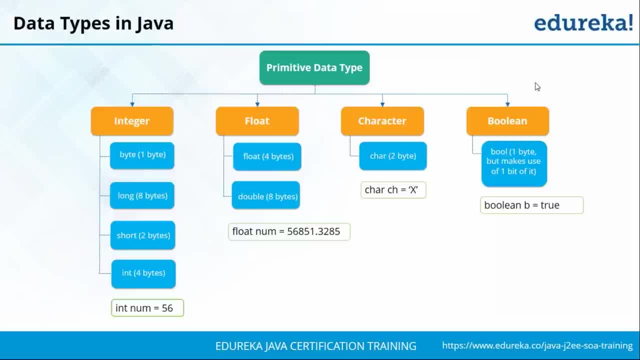 long as well. So if you have a number that is going beyond that as well, you can use long. So, based on your need, you can use a corresponding value. So here you can see how you initialized int num is equal to 56.. 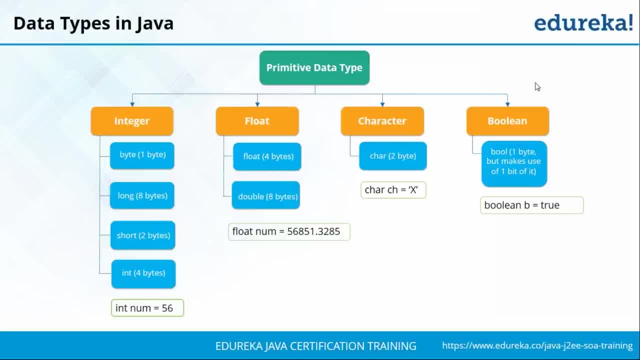 Okay. Okay, So you have a numerical value of integer type that is going to store a value- 56. Now, after that, you have the float type. Again, float type can be used to store decimal pointed numerical value. So in case, if you do have any value that is taking decimal point value, then you're going. 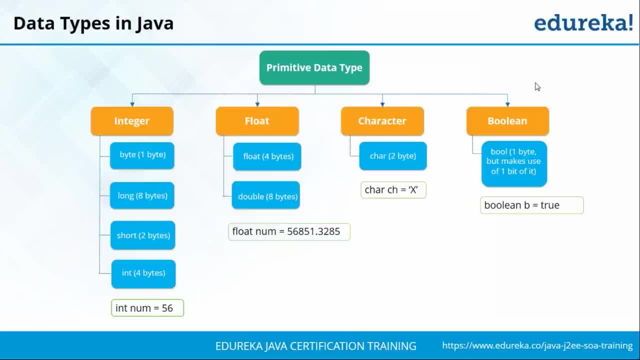 to be using a float variable. So, again, based on your need of storing the number, you can use float or double, and you can see how I've initialized. a floating number is equal to 568151.3285.. With respect to integer and float: okay, so Divya is asking me what will happen if I store. 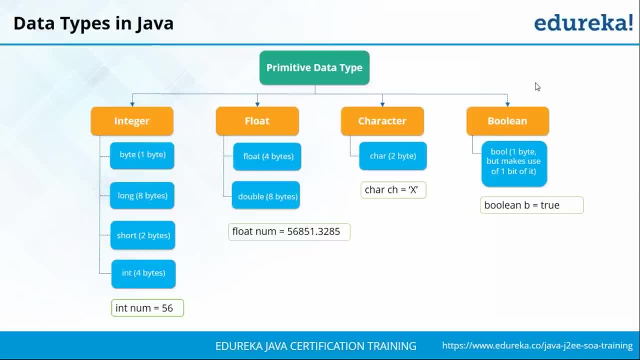 a decimal value inside integer. So good question, Divya. So what happens is that if you initialize a number to be integer and you're going to be storing a decimal value inside that, Let me tell you this. So if, let's say, int num is equal to this value, that is, 56851.3285, then the decimal point. 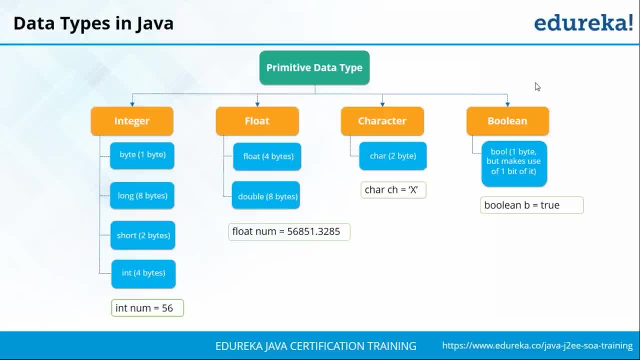 value will be discarded and only 56851 will be stored inside that number. Are you clear, Divya? Alright, Okay, Now, apart from numerical values, let's say, if you wish to store a character, then you have the char type. 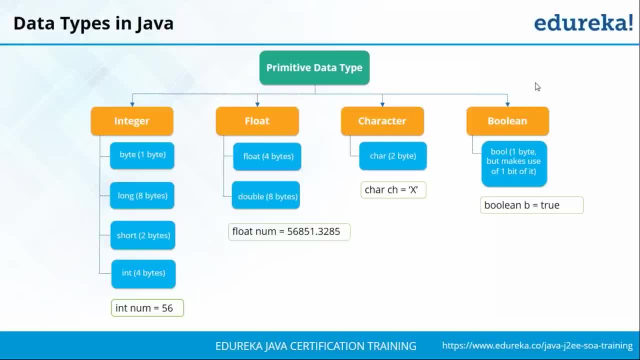 So you can see how you've used character to store a single character. So any of the alphabetical characters, you can store it in part of this. Apart from that, you can even store special characters and numerical values also in this, but they'll be considered to be a character value. 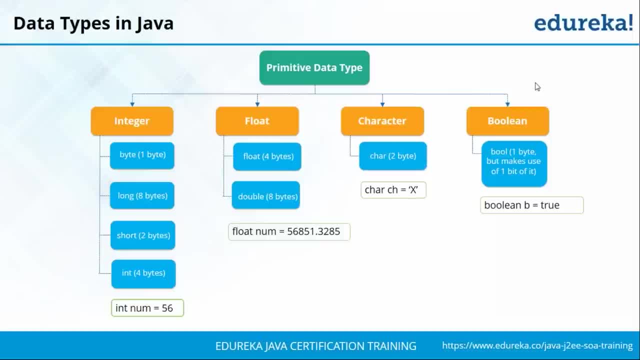 Then you have the Boolean type. Again, Boolean is very straightforward: It can store either true or false value accordingly. So any questions with respect to that, Any questions with respect to the primitive data types present in Java. Okay, Prashant is asking me: can we convert a number stored inside character to an integer? 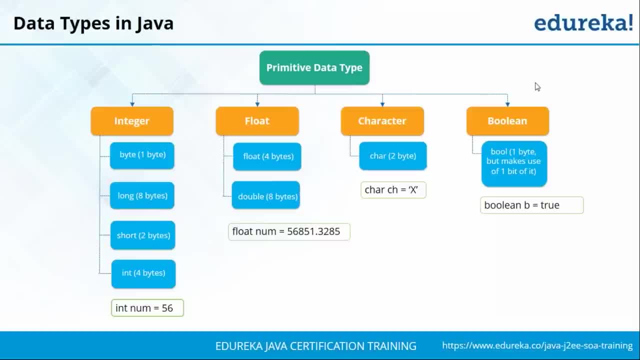 Definitely So. you can convert accordingly, Prashant, but that's a process called typecasting, But for now don't worry about it, You can convert it accordingly. Okay, So Henry is asking me: can I store a word inside a character? 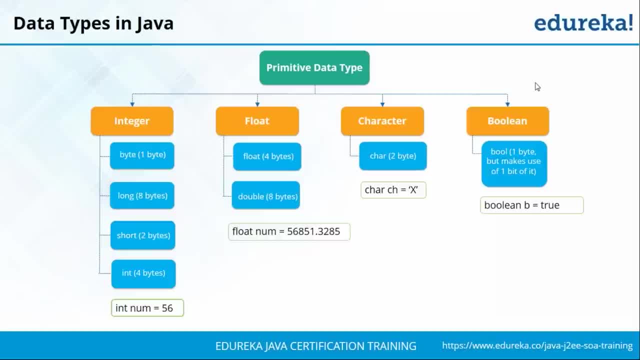 No, Henry, you cannot store a complete word inside a character, But for that we have another type that is called strings. But we'll discuss that later. We'll discuss that in an upcoming slide, so don't worry about it, All right. 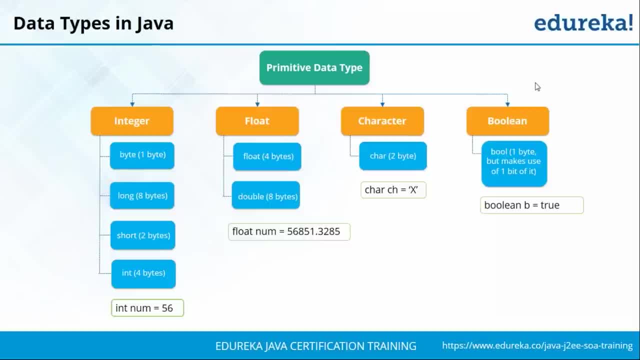 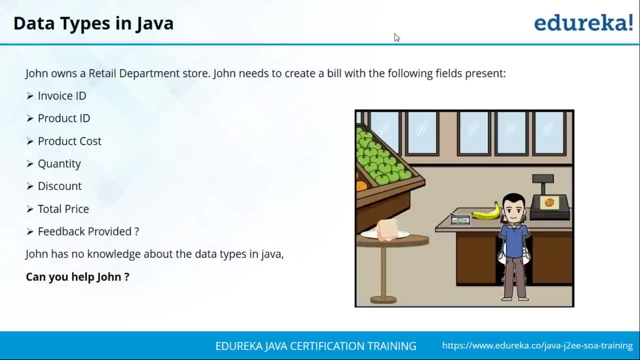 So, moving forward, let's see a use case where you're going to be using the different data types. So now let's look at a use case. So John owns a department store, So he wants to create a bill which has to have the following fields. but John does not. 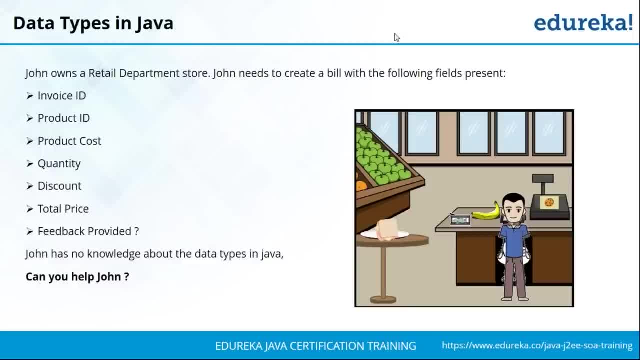 know Java, So he wants you to help him out and create the corresponding fields with the correct data types. So you're going to have an invoice ID. you're going to have a product ID, you're going to have a product cost, You're going to have a quantity, a discount. 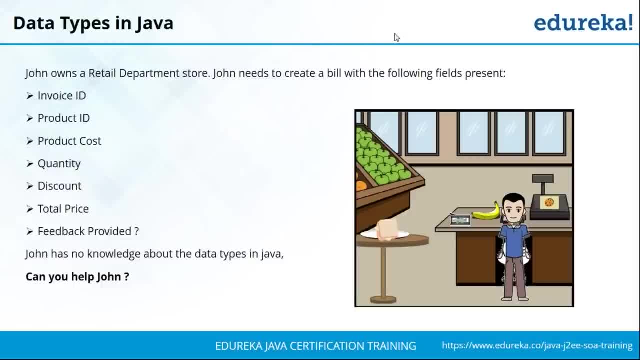 Total price and whether the customer has provided feedback. So can you guys guess which data type is going to be associated to which field? All right, So most of you made your guesses. Let's see how many of you are correct. Your invoice ID is going to be integer. 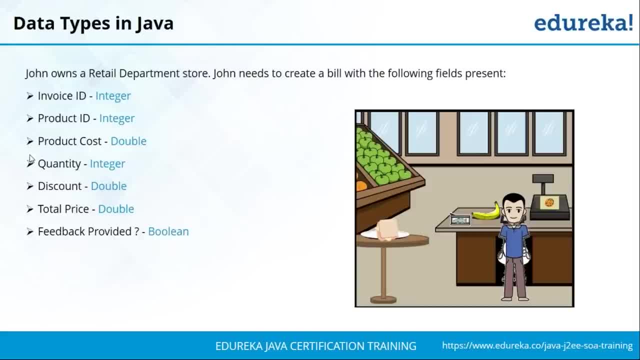 Your product ID is going to be integer. After that, your product cost is going to be double. Now, some of you guessed it to be float, but again, we prefer using double over float because it is more precise. After that, your quantity is going to be again integer. 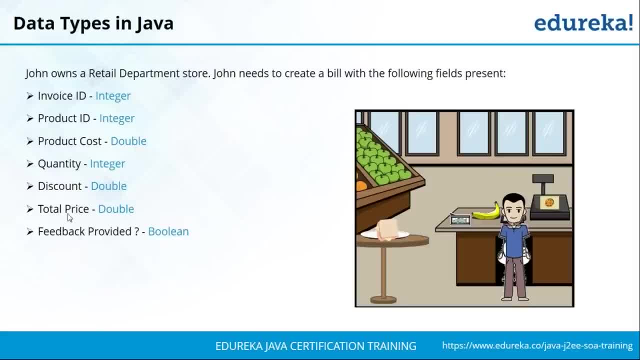 So that's going to be double, Discount is going to be double, Total price is going to be double, and whether feedback has been provided or not is going to be Boolean based on true or false value. Now let me just show you how to declare these values as such in the Eclipse. 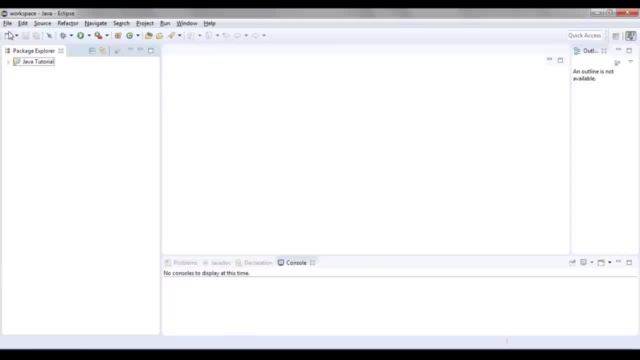 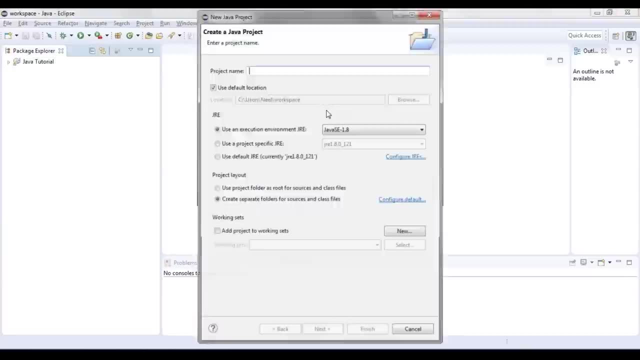 So the first thing that you need to do as part of your Eclipse is you need to create a new project. So on the left- most I can present here- you can select the Java project option. So here you need to specify the name of the project. 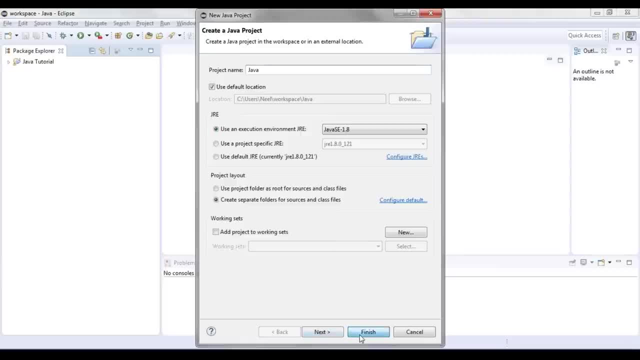 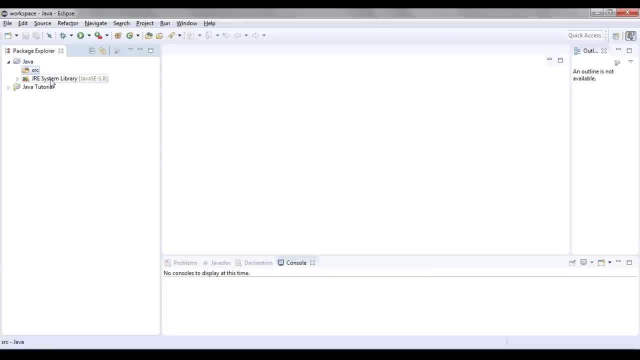 So I'll call it Java, and then you can directly click on finish And automatically a new project is created. Now inside that project you can see you have source as well as the Java system library. This is basically all the libraries to which you can access to as part of your Java environment. 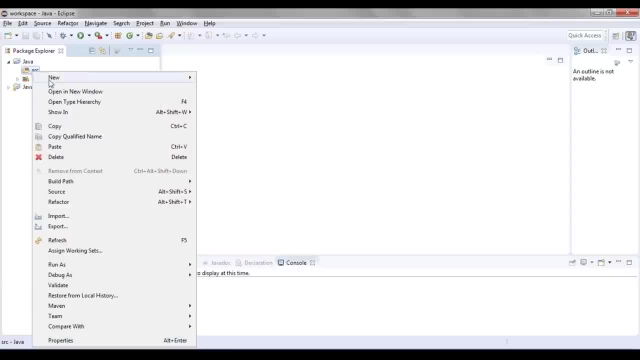 So now I need to create a new class file. So right click and then go to the option and click class file. So I had mentioned to you earlier as well: everything that you're going to be writing is going to be part of a class. 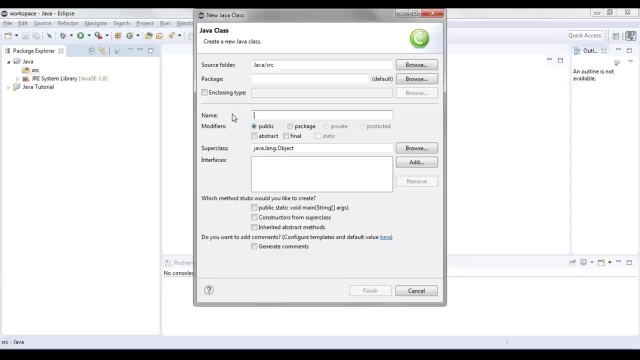 So click on class and then you need to specify the name of the class. Now, one thing that you need to do is you need to specify the name of the class. So one thing to remember is that, as part of the naming conventions for class, you cannot. 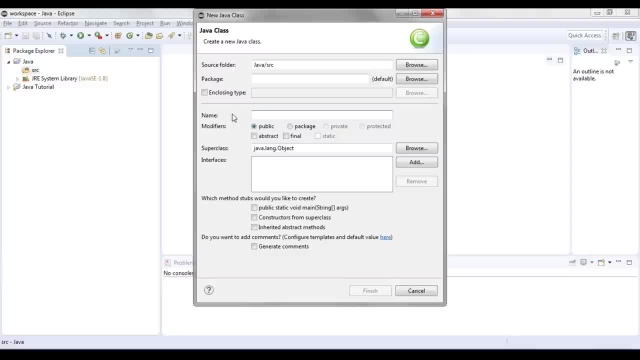 use white spaces as such. So what I'm going to do, I'm going to make it as retail shop, retail underscore shop, So don't make any changes here as such, but one thing is make sure you have checked this option. that is public static void name. 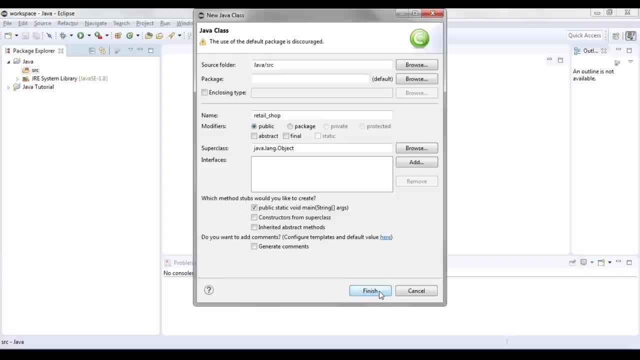 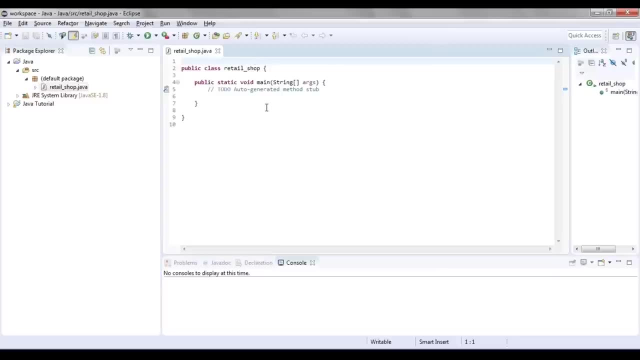 This basically means that inside your class, your main function is going to be: So just click on finish and you have your class file created here. Okay, Bharat is asking me: what does the main function do? Okay, But basically, every time that you're going to be executing your code, your code starts. 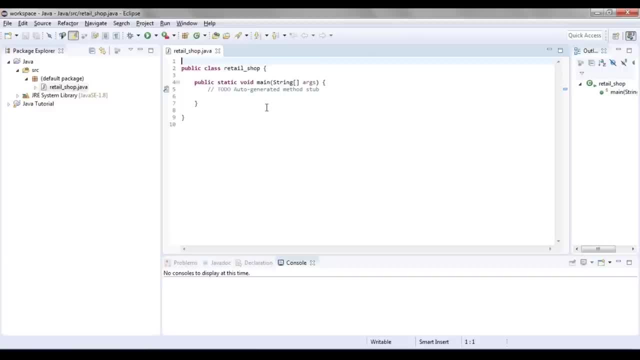 executing from that main. So wherever you're going to specify in your main, there your code starts executing. For now don't worry about these concepts. public static void main. We'll be discussing more about that in our next session about classes and objects. 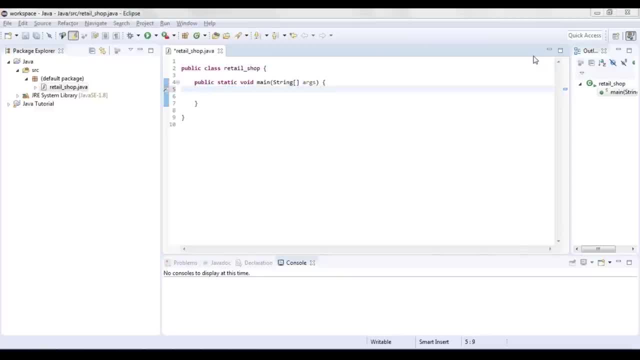 For now, all you need to do is I'll show you how to declare these variables. So first, what are you going to do is that you're going to specify integer type. Now, for integer type, All you need to do You need to specify int. 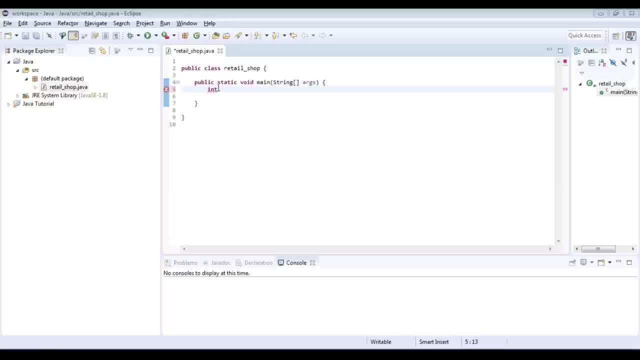 So just type int and system will consider to be integer. So you can see it's been highlighted separately because these are reserved keywords. That is, when you're using these keywords, Java in turn understands that this refers to integer. Now, in my integer I had my invoice number. 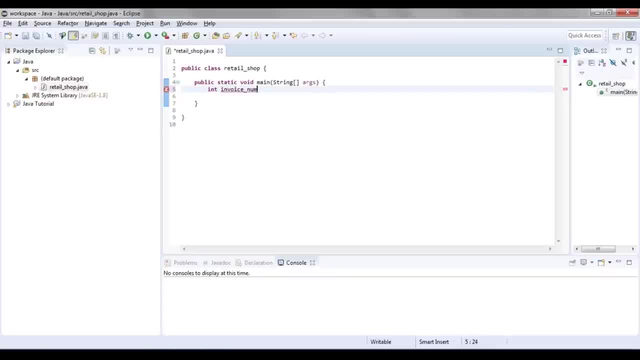 So I'm going to say invoice underscore num, So this is a variable name. So whenever I'm going to use invoice number as part of my code, it basically means that this is a variable that is of integer type. So if you have multiple variables of the same type rather than declaring them individually, 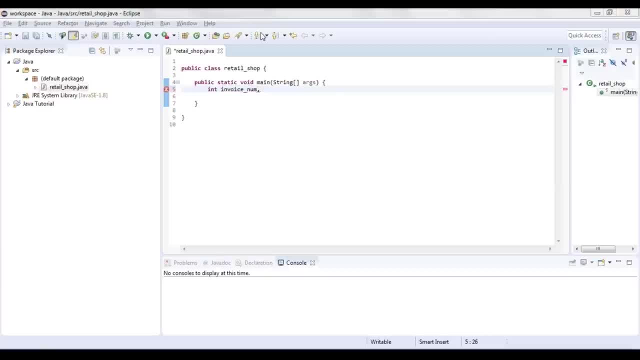 all you can do is put a comma and then start specifying the next variable name. So after the invoice ID we had the product ID, So that is product underscore ID. And then the third integer value that we had was quantity, So I'm going to call it quant. 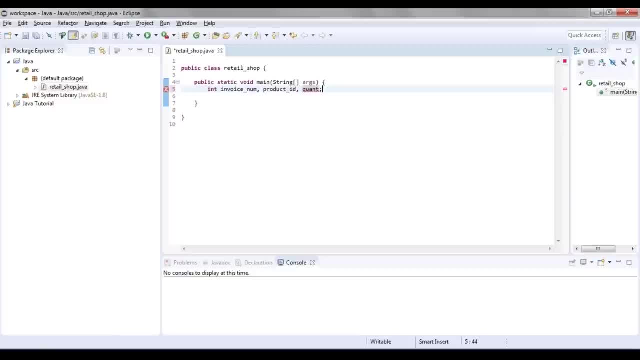 And after every statement make sure you put a colon here. So this basically Basically tells that this is an end of a statement. So in Java it is very important that you make use of semicolon at the end of every statement. So this is a challenge most programmers face initially, where they forget to put semicolon. 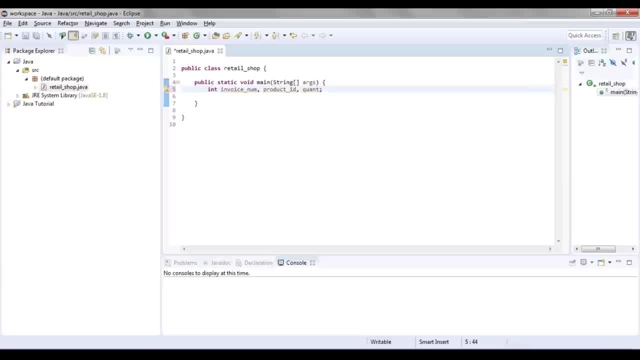 at the end of their statement And they end up having a lot of errors corresponding to that. So every statement has to end with a semicolon. After that we had double values. So for double, what you're going to do is you're going to go next line and you're. 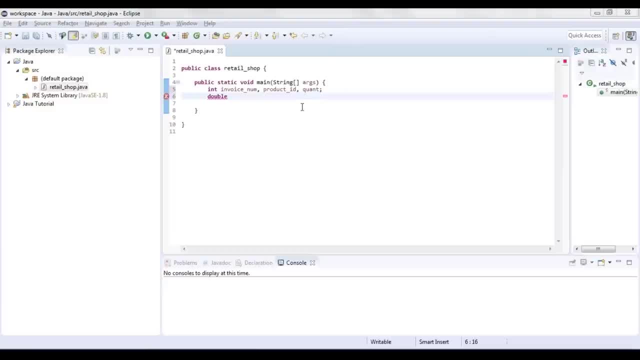 going to call it double. Now I had my cost, That was, so I'll just call it cost. Then I had discount And then I had my final price, So I'll just call it price. So these were doubles. Now, to specify a Boolean type, you have to completely type Boolean B. That would be Boolean. 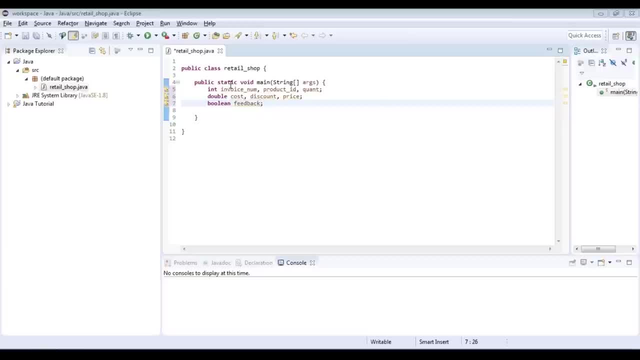 And then you had feedback. So this is how you define different data types in Java. So by default, all the integers would be assigned zero, The doubles would be again 0.0. And your feedback would be set as true. So are you clear on how to declare variables in Java. 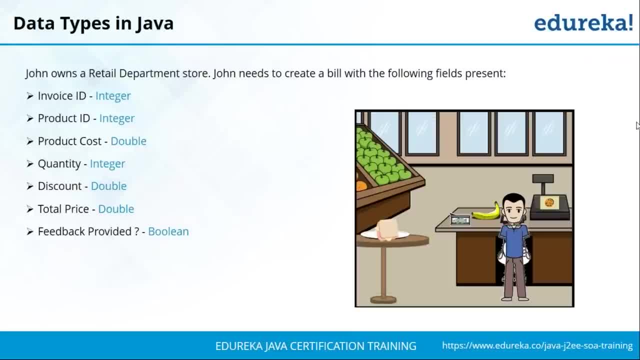 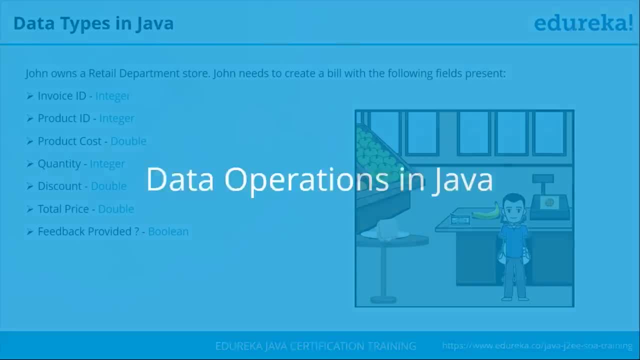 Okay, Divya is clear. so is Sandeep Arun. Anna, That's great to see guys. So now that we've seen the various data types in Java, let's move forward and look at the various data operations that you can perform in Java. 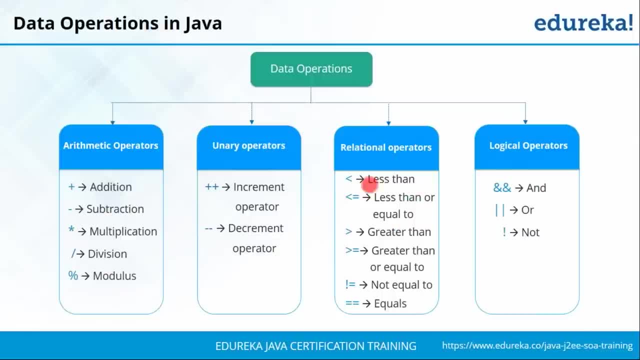 So you have mainly four different types of operators in Java. So you have your arithmetic operators, that is, to perform arithmetic operation, you have abstraction division and finally you have modulus. So this is something that you may not be familiar with if you're not from a programming background. 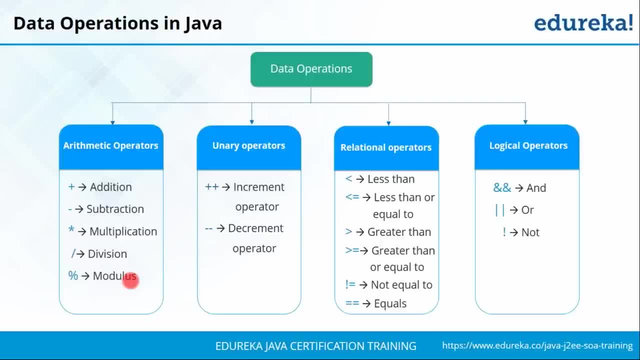 Basically, what modulus does is that it performs division, but rather than giving you the quotient, what it gives you is the remainder of that division. So let's say you want to perform 5 divided by 3, rather than getting 1, what you're going? 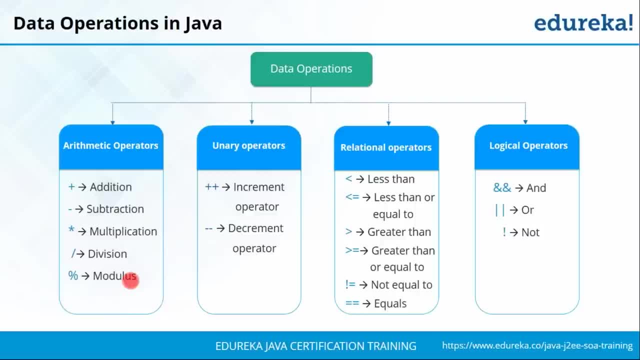 to be getting is that you're going to be getting 2 as the remainder value, And then you have the unary operator. Now the unary operators basically are increment and decrement value. So let's say there is a specific value that you have initialized. 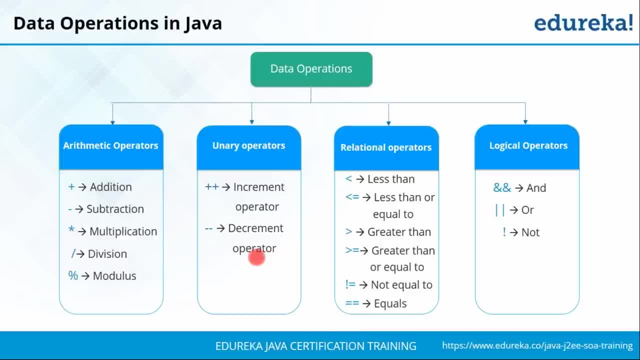 So let's say you have an a that is equal to 10.. And somewhere in your program you want to increment it after a certain set of operations. So what you're going to do is that you want to increment the value of a with the increment. 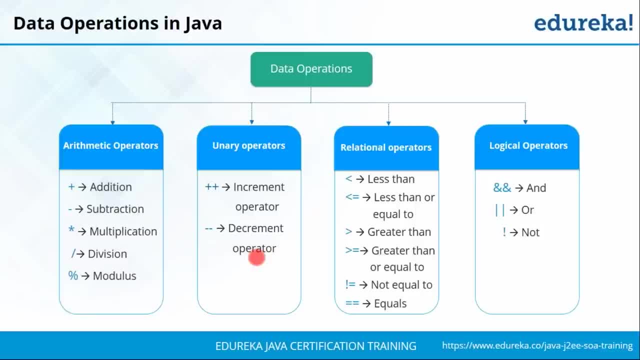 operation. Now, don't worry too much on this. We'll be using the increment operator in the loop statements and I'll show you how it plays an essential role as part of control statements. Then you have the relational statements. Now, this is something that you may be familiar with. 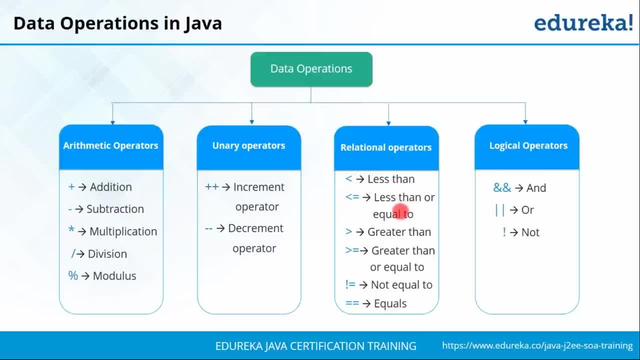 You have lesser than, you have greater than or equal to. You have lesser than equal to, you have greater than you have not equal to. Again, not equal to is represented with an exclamation mark and equal to sign. So when you do that, it basically means it's a not equal to. 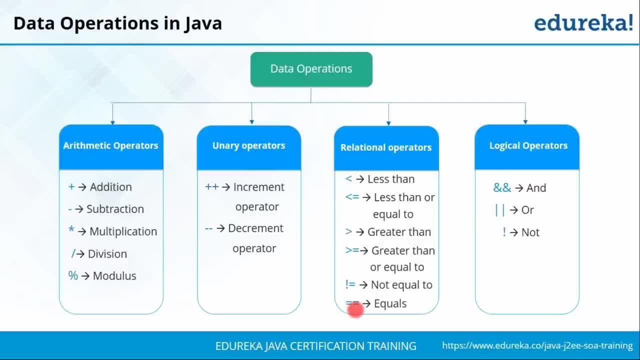 And for equal to, it is double equal to, Because if you put a single equal to, it will consider to be an assignment operation. So finally, we have the logical operators. Now, in the logical operators you have three main operators. You have AND, OR and NOT. 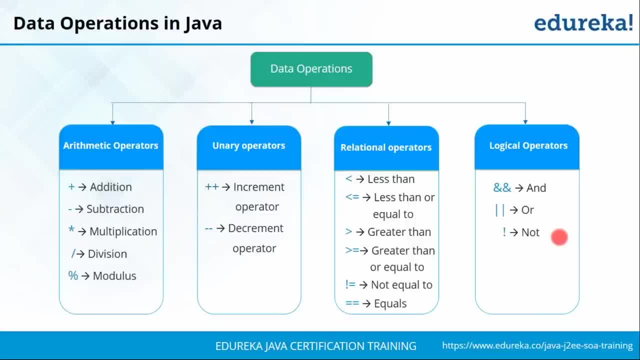 So, basically, the NOT condition is used to negate the corresponding value. So let's say there's a variable, There's a condition that is true, Then if you want to negate it, you're going to be using a NOT value. Now, the two operators that you need to emphasize on is the AND and OR operators. 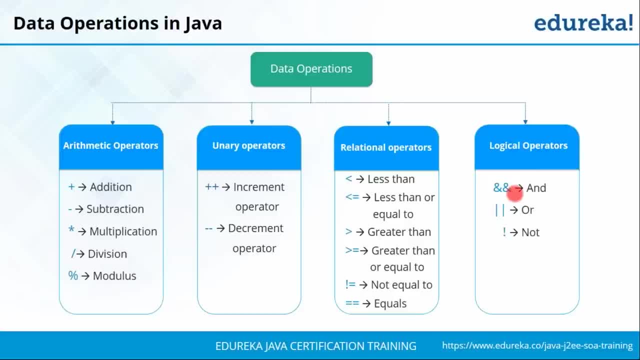 So here you're going to be working with different conditions as such, That is, you're going to be using the AND and OR operator on different conditions. Now let's say both my conditions are true, So in that case both of these operators will give me the output to be true. 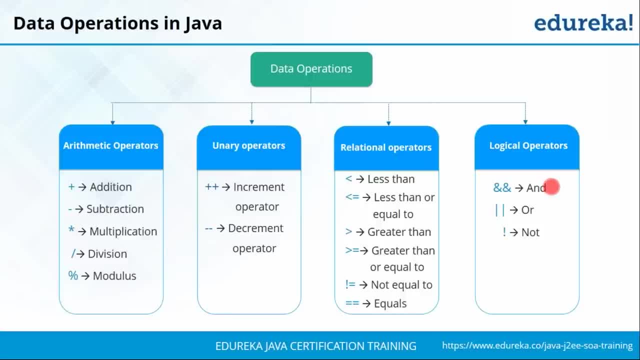 But in case if one of your condition is true and the other is false? Now, in that case, Your OR operator will give you the output value to be true And your AND operator will give it to be false. So, unless and until all your conditions are true, 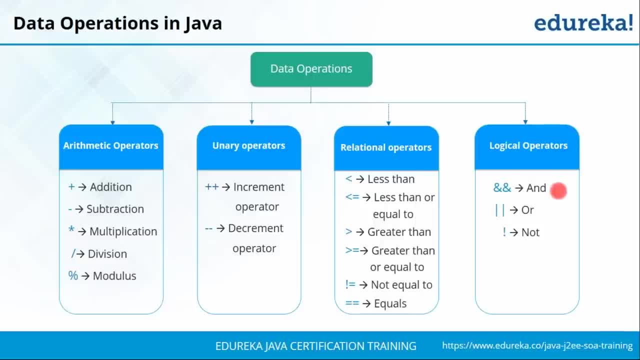 You will not get a true value to be output in case of an AND operator, But in case of an OR operator, as long as there's at least one true statement, Then you can get the output to be true. Now these will be used in control statements again. 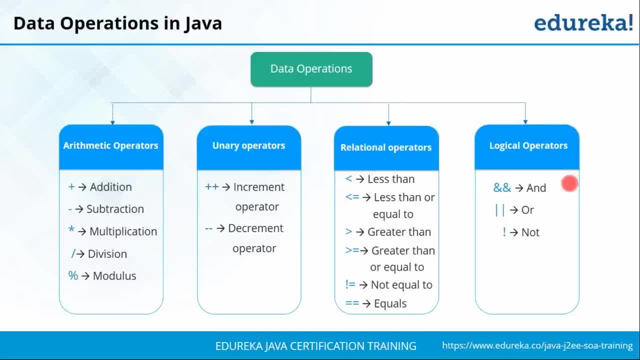 Now, don't worry, you'll be seeing that in the upcoming sessions, But I hope you've got a complete overview with respect to the different data operators. Okay, Divya is clear. So is Bharat, Okay, So let me give you an example here. 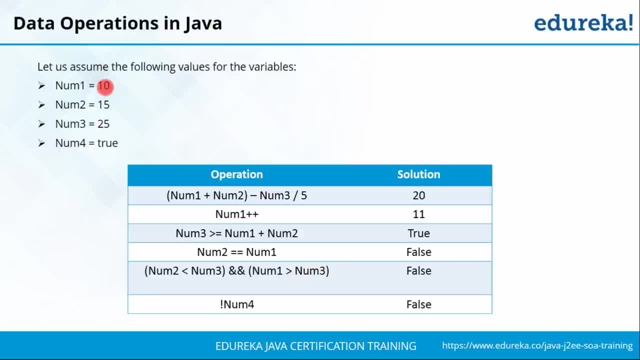 So basically what you're doing is that you're taking four different values And then you're correspondingly assigning them an operation. So I had told you earlier, equal to is used to assign a specific value to that variable. So this is an assignment operation. 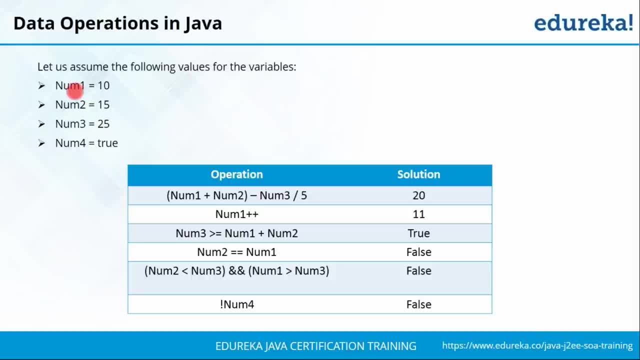 So this is also another operation that you're performing in Java. So what I'm doing is that I'm assigning num1 to be 10,, num2 to be 15, and num3 to be 25.. So here I'm taking the value. 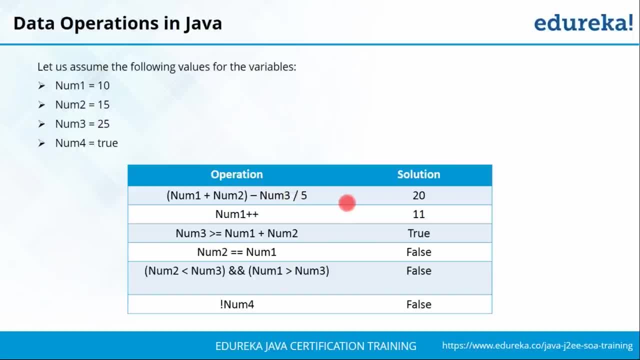 What happens is that there is a board mass rule that you follow. Now this is something that you have again in maths that you may be familiar with. First the bracket value is computed, Then you're going to be seeing the proofs and proofs. So you have division first, multiplication, addition then subtraction. 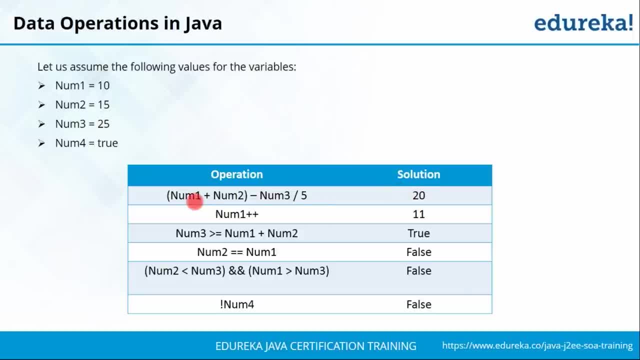 So let's look at this operation present here Now. let me help you understand how it happens here Now. before any arithmetic expression is computed, you're going to be following the board mass rule, That is, you're going to first consider the brackets, Then you're going to be checking for 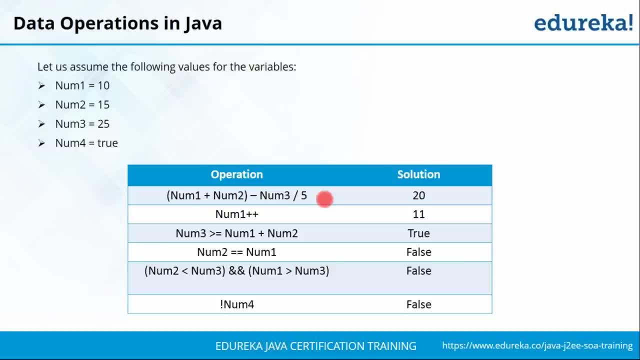 Any divisions present, then multiplications, additions and finally subtractions. So if you look at the operation present here inside the brackets, you have an addition happening. So you're going to add 10 plus 15, you're going to get 25.. 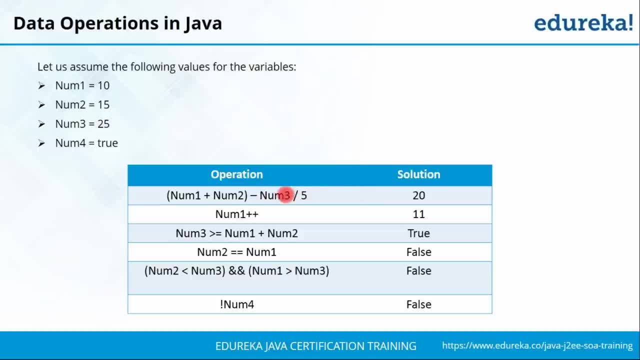 Then you're going to come out: Before you subtract 25 from 25, you're going to perform the division operation, That is, 25 is going to be divided by 5, which will give you the output to be 5.. So, from 25,, 5 is going to be subtracted and you're going to get the output to be 20.. 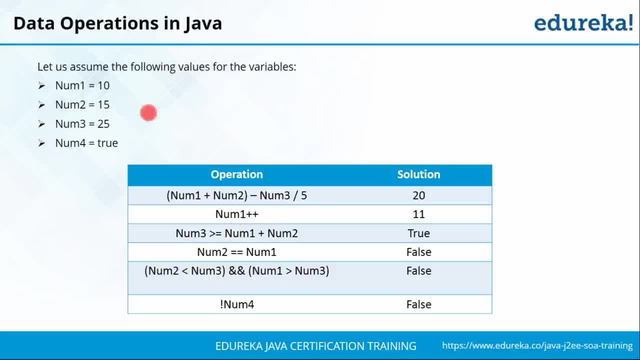 Now again, when you see you're using an increment operator. Now my original value of num1 was set to be 10, when I'm using the increment operator, then it is going to be increased to 11.. After that you're using a logical operator where you're comparing. 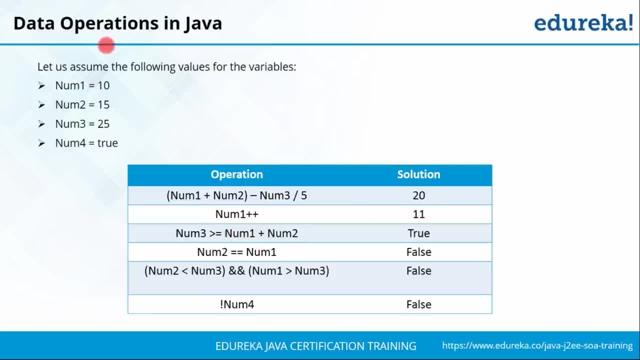 That is, is num3 greater than equal to num1 plus num2.. So 10 plus 15 is equal to 25, therefore it's going to give you an output to be true. Then you're checking: is num2 equal to num1. 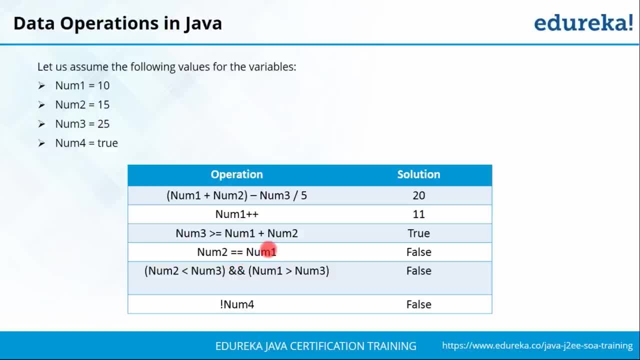 This is why you're using a double equal to. if you use a single equal to, the value of num1 will be assigned to num2.. So, in case, if you want to compare two values, you're going to use a double equal to. 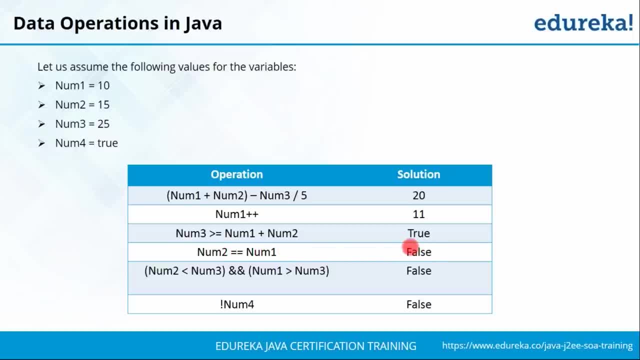 So num2 is not equal to num1, so it's going to give you an output of false. And finally, you're using a logical AND operator here. So is num2 lesser than num3? Yes, it is. 15 is less than 25.. 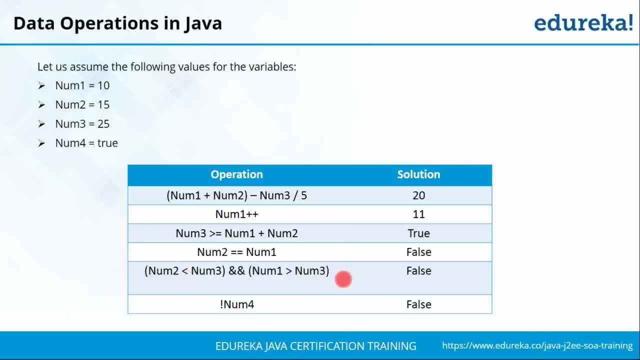 And then you're going to check. so one of my condition is true. Then, when you come to the right hand side of the operator, is num1 greater than num3? No, that is false. Therefore, I have true and I'm going to perform AND operation with false values. 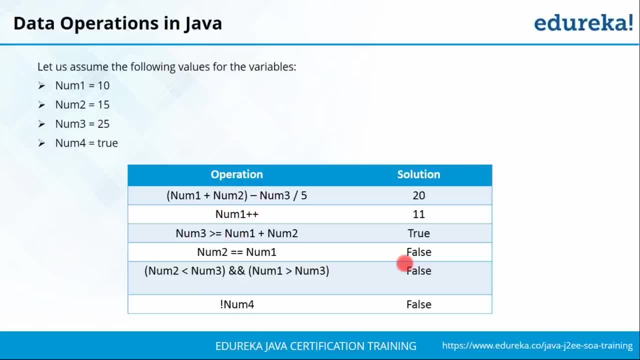 And this is going to give me a false output. So we had discussed this earlier. until and unless all my conditions are true, I will not get an output to be true in case I'm using an AND operator. Finally, I had initialized num4 to be true and I'm negating that value it is giving. 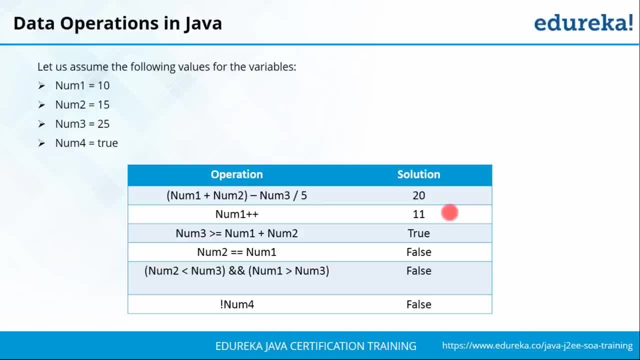 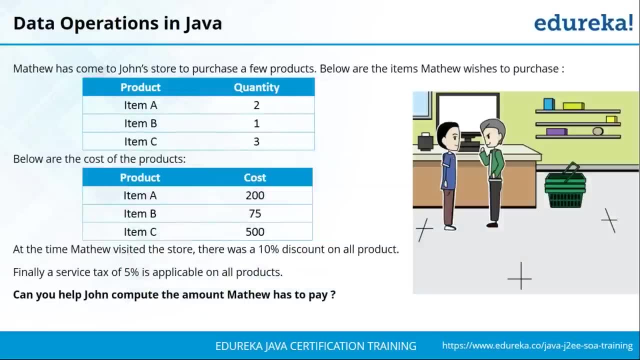 me an output of false. So I hope with this, you're clear with respect to the data operations. Okay, So moving forward, let's look at a use case where you'll be using these operators as such. So Matthew has come back. He's to John's retail store. 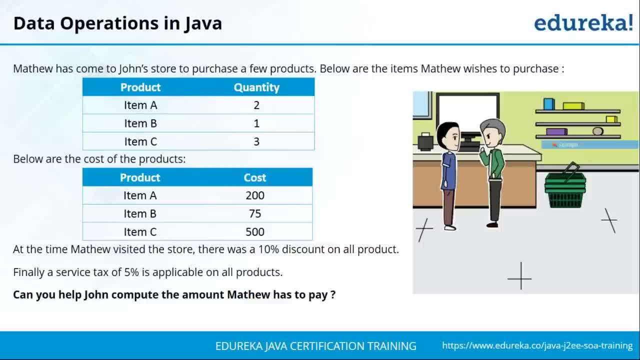 Matthew wants to purchase a few products from John's store and he's given John the list of products that he wants. So John wants two quantity of item A, he wants a single quantity of item B and he wants three quantities of item C. So already the prices of these products have been displayed. 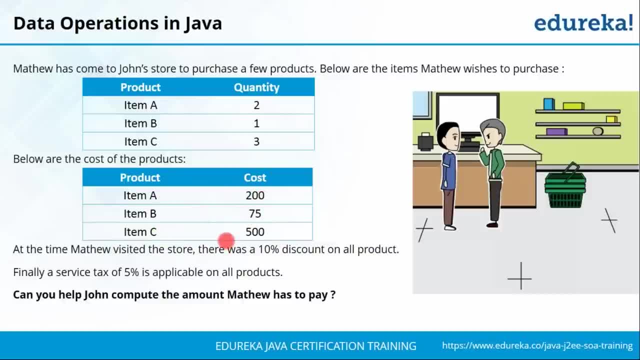 Item A cost 200, item B cost 75 and item C cost 500.. Now, at the time Matthew visited John's shop, there was a 10% on all the products as such. Now, from your total cost, you need to subtract 10%. 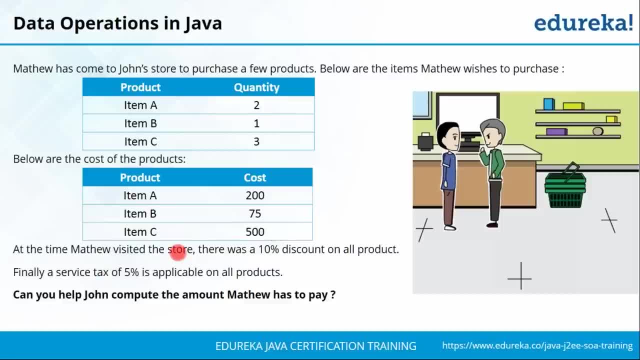 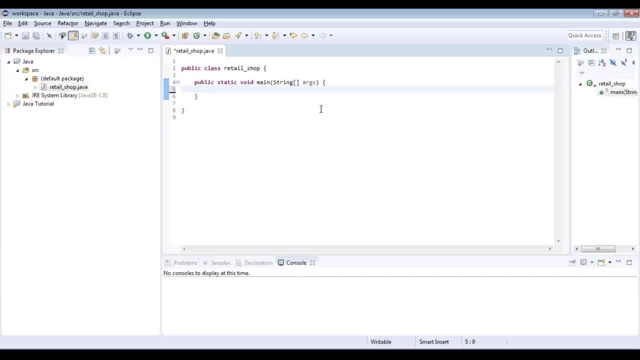 Apart from that, there was also a 5% service tax applicable on this, So you need to add a 5% service tax as well. So let me show you how it is done. So now let's go ahead and write a code to compute this value. 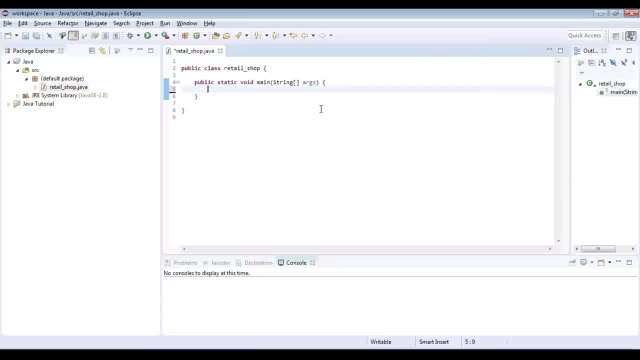 So I have three items which have a corresponding value. So what I'm going to do is that I'm going to call them to be my variable. Since they don't have a decimal value, I'm going to make them integer. so int item A. 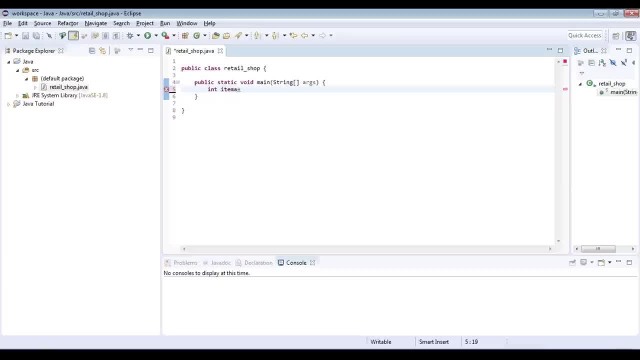 and then I'm going to initialize it. I'm going to initialize it with the corresponding value. So item A cost 200, so I have given the corresponding value. Then I had item B, which is equal to 75, and then we had item C, which was equal to 500. 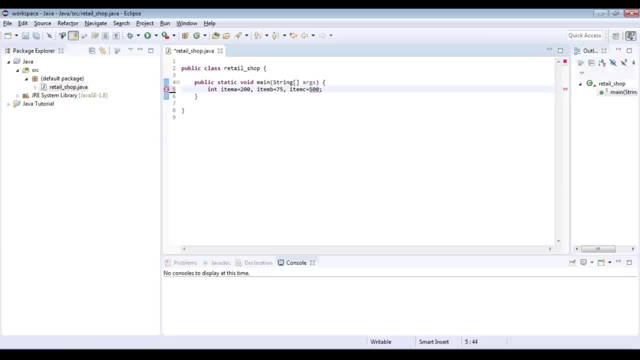 So again, once you're done in declaring these variables, put a colon, and then we need another variable which will store the total price. So I'm going to call it double price. So you can see, here we are not only declaring variables, We are also initializing them with the corresponding values. 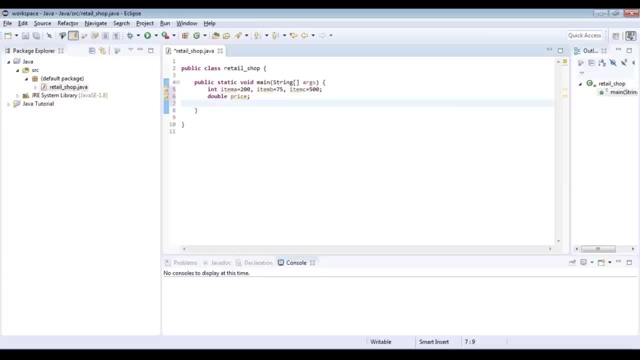 In the case, if you want to set a corresponding value for a variable before you go ahead and use it, you can initialize it at the time of declaration itself. So that's exactly what we have done here. So now, finally, let's go ahead and compute our price. 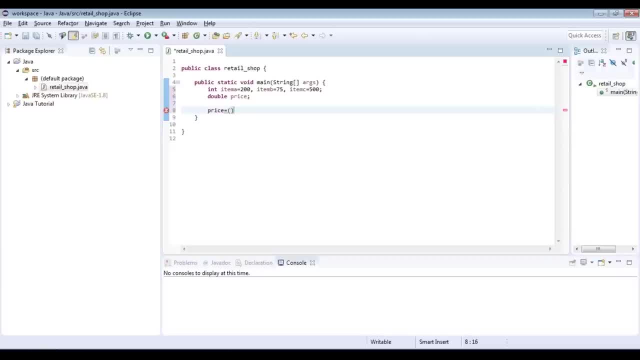 So price is equal to. now let's write the expression. So I'm going to use multiple parentheses here so that I can perform all the operations in one single code. Matthew wanted two quantities of item A, So item A cost 200.. Item A into two. 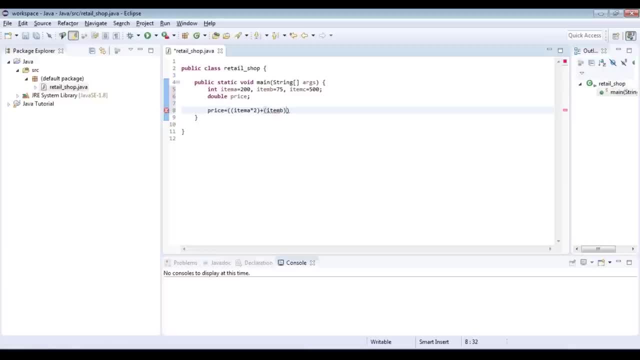 Then he wanted a single quantity of item B. Finally he wanted three quantities of item C, So item C into three. So with this we've computed the total value of these products, But we've seen that there was a 10% discount associated with these products. 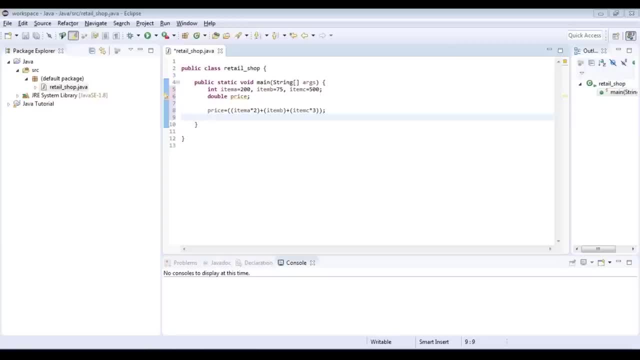 So I need to compute that value and then to that value I need to add a 5% service tax. So again, price is equal to Price, minus 0.1 into price. So here what you're doing is that the existing value of price you're going to subtract it. 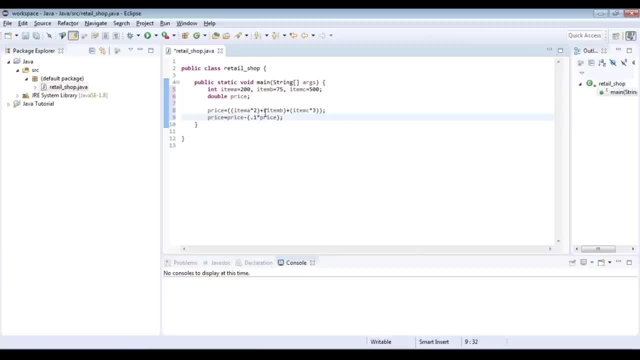 with 10% of the price value. So this value, once it's computed, will be updated and stored inside price. So always you need to remember that the expression to the right hand side of assignment is computed first and then the corresponding value is stored inside the variable to the left. 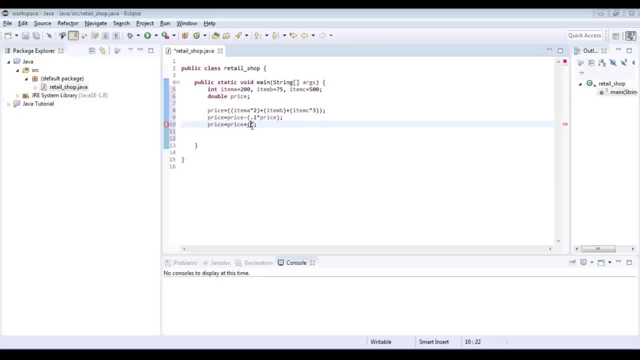 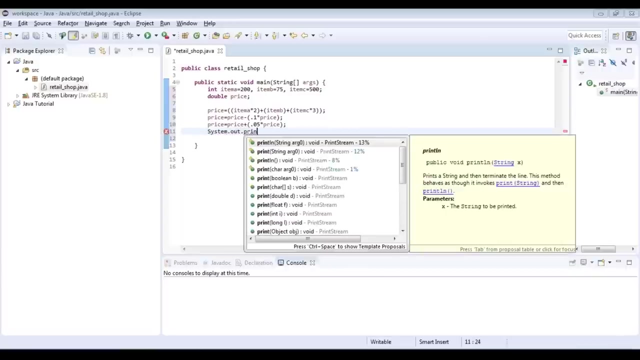 And finally, we need to add a 5% tax to this. Now, to do that is to 0.05 into price. So with this we've also added the tax. So it's time we print out this value for it. Now to print any command in Java, you're going to use the following syntax, that is, systemoutprintln. 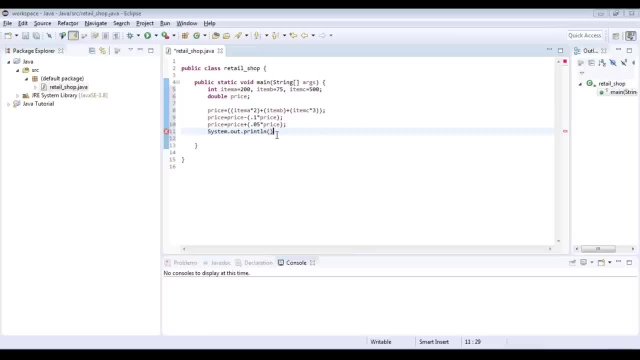 And then, inside quotes, you can specify what you want to print. Now there's another simple way of doing this. All you need to do is just type sysout and then press control plus space, So this will directly convert your sysout statement to systemoutprintln. 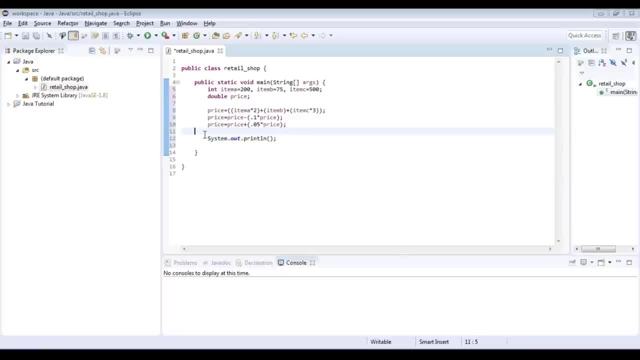 So this is basically a shortcut in Eclipse. So here I need to print my price value, So all you need to do is specify price. So with that just save the code, and then it's time we run it. Right click on the space and then you have an option here: run as. 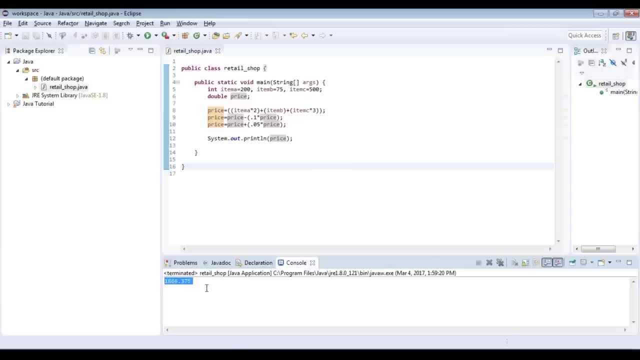 So select Java application And then you can see, finally, the output that is computed. So with this I hope you're clear on how to use the various data operators and how you can print a corresponding value out to your screen. Okay, so I've got a confirmation from everyone. 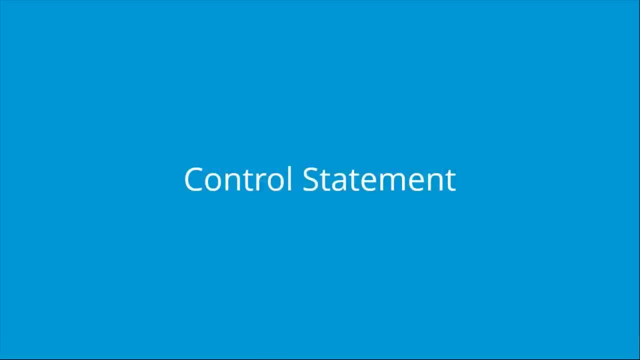 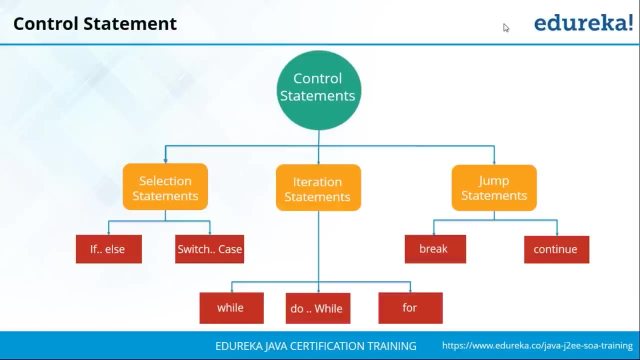 So let's move forward to the next topic, that is, the control statements. Now, the control statements are basically the statements that will define how the flow of your program code is going to go ahead. Now there are mainly three types of control statements in Java. 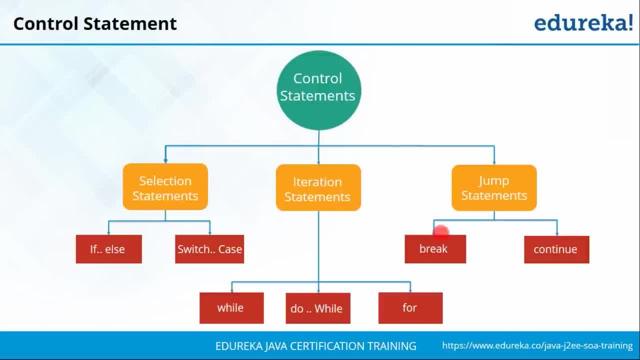 You have the selection statement, you have the iteration statement and then you have the jump statement. Now, inside the selection statement, you have if and else. then you also have switch case. Now these are two types of selection statements that you will be using, based on your requirements. 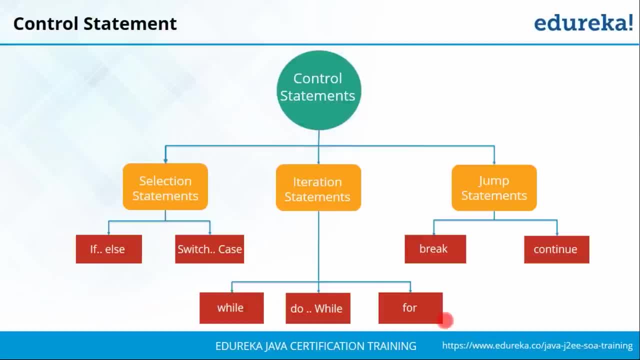 After that you have your iteration statements or, as they are better known, you have looping statements. So there are mainly three types of loops in Java. You have your while loop, you have your do while loop and you have your for loop And finally we have jump statements, that is, break and continue, which will be used. 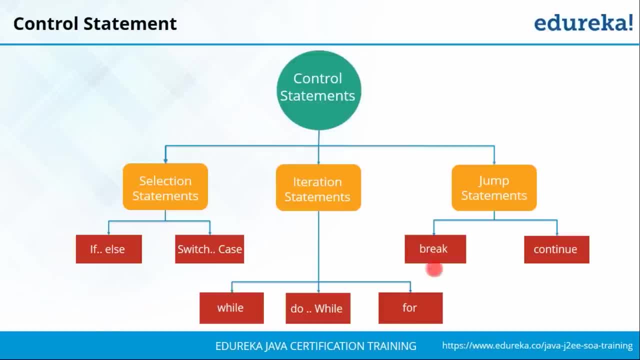 to jump to a specific point in your program. Now, don't worry, we'll be discussing about each of them, So let's get started. Okay, Let's look at each of them in detail. So now that you've got an overview of the various control statements, let's move forward. 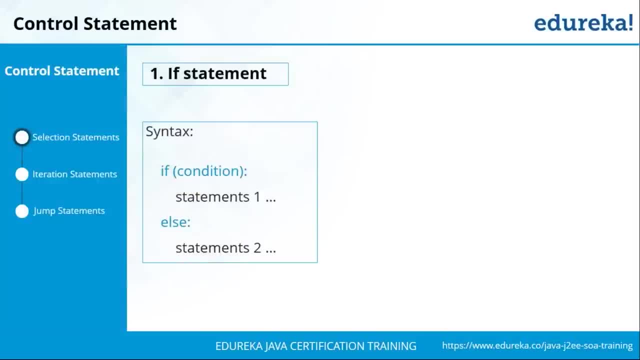 and look at each of them one by one. We'll start off with the if statement Now. the basic syntax for the if-else control statement is that you have if, followed by a condition, then, in case if the condition is true, the statements which have to be executed. 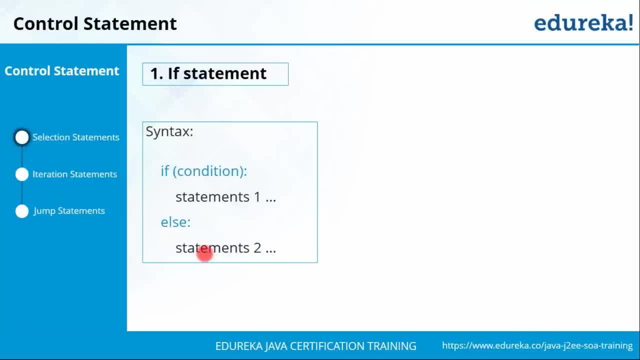 If the condition is to be false, it will go to the else block and then it will execute the statements here. So it's not restricted that you can only check one condition with if-else. You can have a multiple if-else statement. 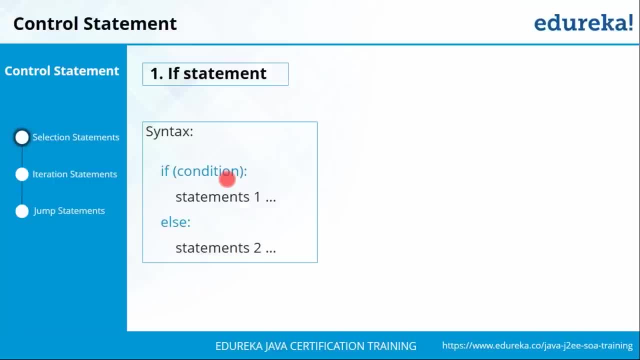 So you can check: if condition one is true, then you can execute statement one. else if you can check condition two, if condition two is true, then you can go and execute statement two again, else if condition three, and so forth. 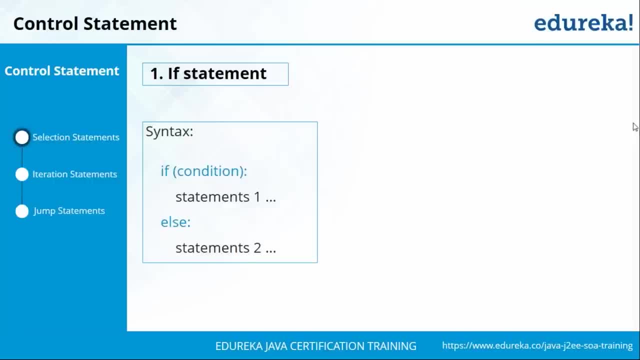 So you can have a laddered if-else. So I'll just give you an overview of how the if-else works. So you always start your program and then you check whether it is right Now, if it is found to be true, that is, if it's raining. 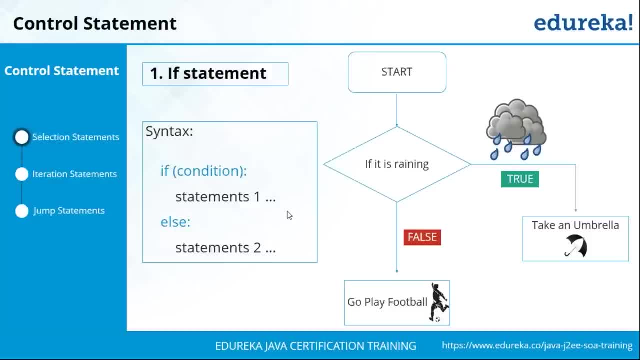 Then you need to take an umbrella, But if it's not true, then you're going to go play football. So are you clear with respect to how an if-else statement works? Okay, Prashant says yes, so does Bharat Henry is clear, Divya Arun- that's great to see. 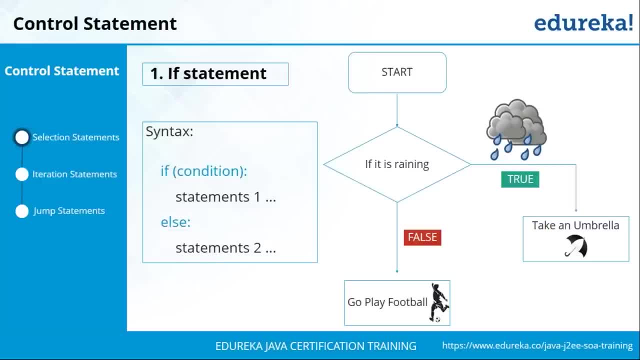 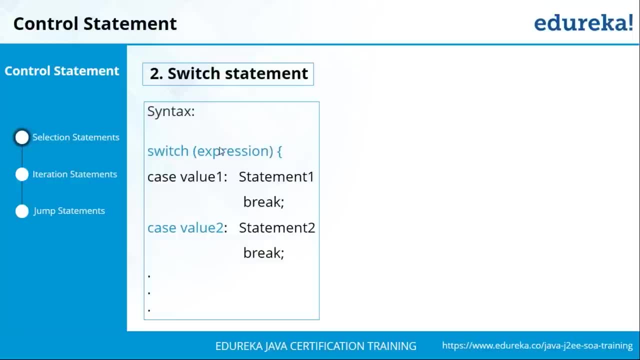 guys. Now moving on ahead, the next selection statement that you're going to be talking about is the switch case statement. Now, when compared to the if-else statement, the switch case is quite straightforward. So here, what you're going to do is that you're just going to write switch. 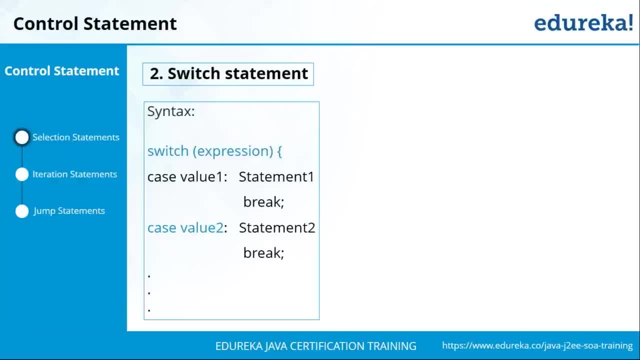 And then the expression here. So you need to understand. here, in case of a switch, putting in a condition would become problematic. Here you need to specify a direct expression as such. Now to give you a better idea, let's say: if you want to compare two numbers, then you're. 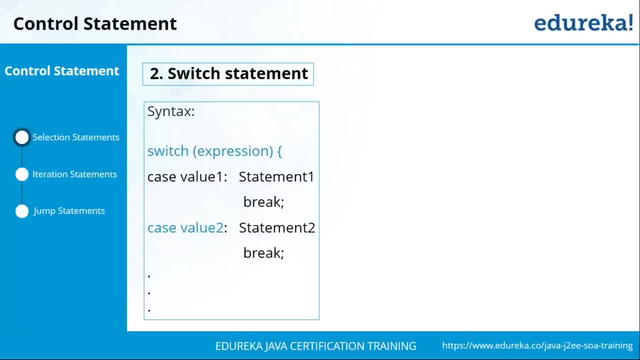 going to use an if-else statement, But let's say, if there's a specific value that you want to check against, then you're going to be using a switch case. So how switch case works is you specify switch, followed by the expression 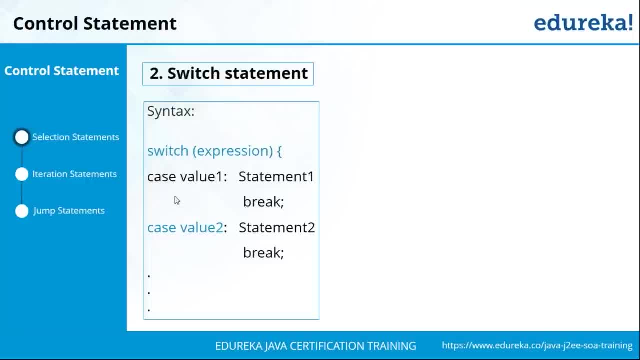 Then you come inside the loop And then you start writing the different cases. So your case one will check against the value that the expression will be taking And then, if it is true, it'll execute statement one And then it'll break from that switch case statement. 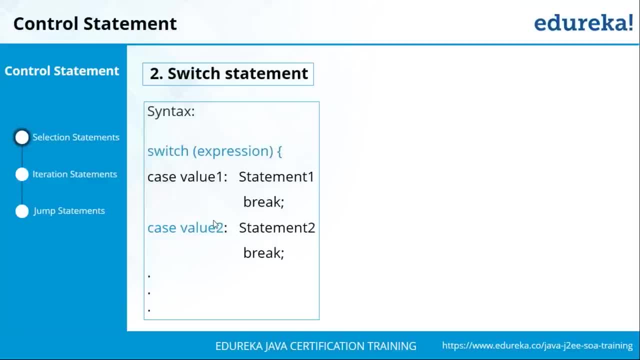 But if it is found to be false, then it'll check the next case. Now, if the next case is found to be true, it'll execute statement two And then it'll break from that. So I hope with this you've got a general idea. 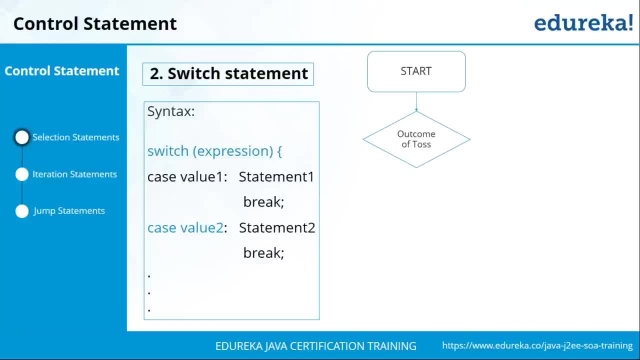 So to give you a better understanding of how the switch case works, let's look at an example here. So basically, you're tossing a coin here. So if it's heads, then Tom wins and then it's the end of the game. But if it is false and it's true, then Adam wins and the game ends. 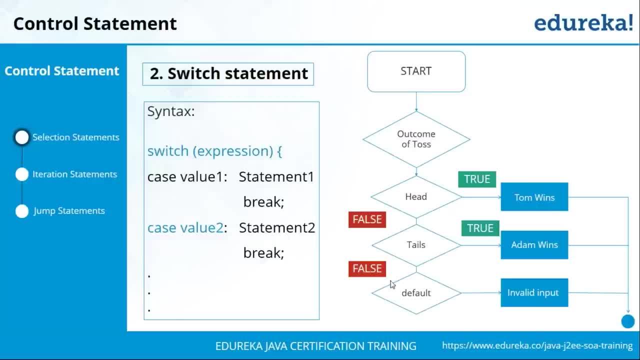 But let's say you've taken a wrong input from the user. Then you're going to go to the default statement and then print invalid input. and come Now. the default statement is the last case that is going to be executed if your expression does not meet any of the case values that you have specified. 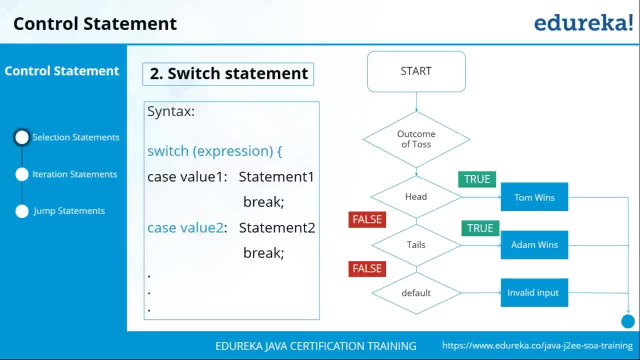 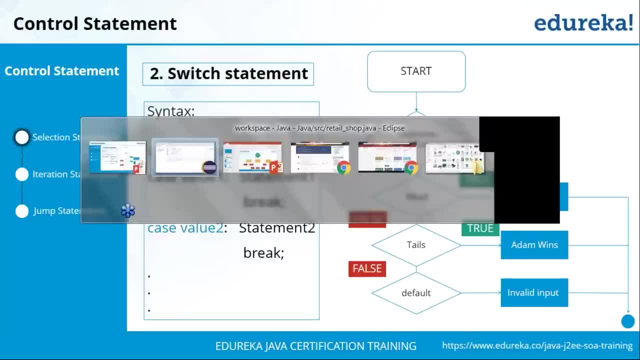 So are you clear with respect to how the if-else statement works And how the switch case works. All right, Okay, now let me give you an example with respect to the if-else and switch statement. Let's go back to our pricing system itself. 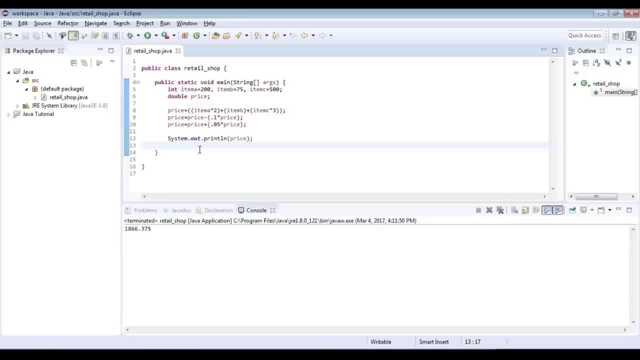 So here, let's say, you want to provide an additional discount to the customer if he's purchased over 1,500 rupees. So what you're going to do is that you're going to write an if-else statement here. So if my price is greater than 1,500, then what you're going to do is that you're going. 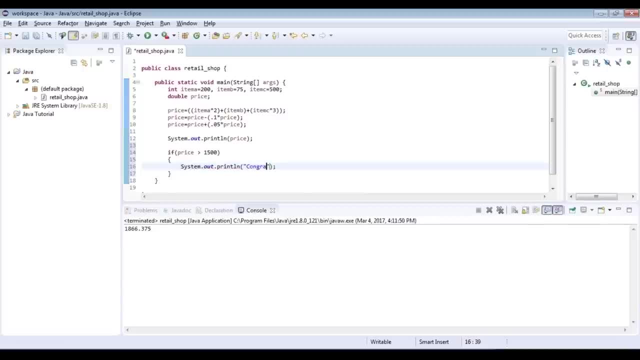 to print congrats. you have a 25% discount coupon Now in case, if it is not greater than 1,500, then what I'll do is I'll change it to else. Then here you're going to specify the else condition. 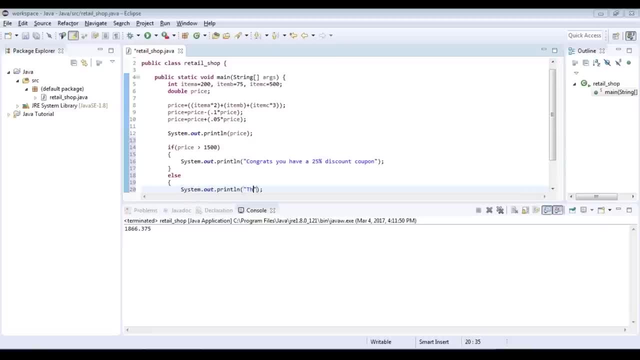 I'm just going to say thank you for shopping with us. So, basically, what we're trying to establish here is that if the customer has purchased, if he has purchased products worth more than 1,500 from John Shaw, then he's going to get. 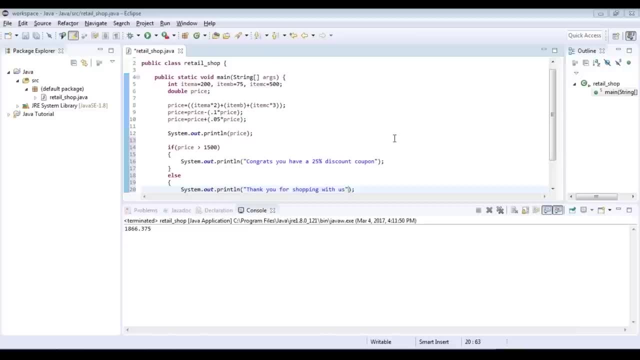 an additional 25% discount coupon that he can use next time. So again, when the next time that he comes, instead of giving him a 10% discount, he can avail a 25% discount. But in case if he's not purchased more than 1,500, then he does not- then the corresponding 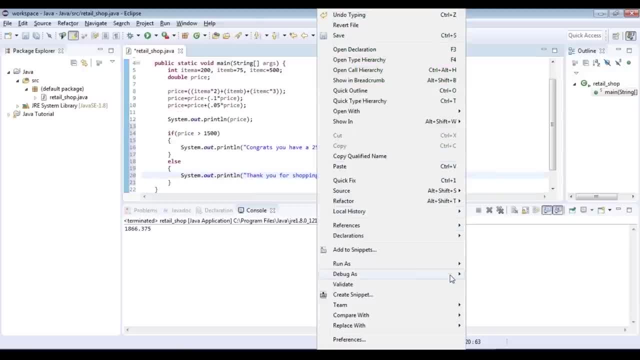 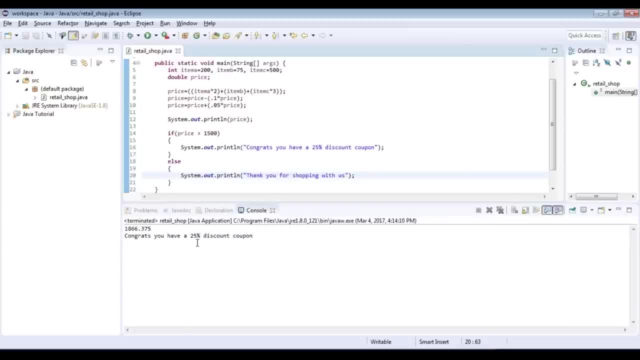 message does not get executed. So I'll just run this program again So you can see he's purchased for 1,866.. So therefore he's getting a discount of 25%. So here let's say I'm going to reduce the price that he's paid. price is equal to price. 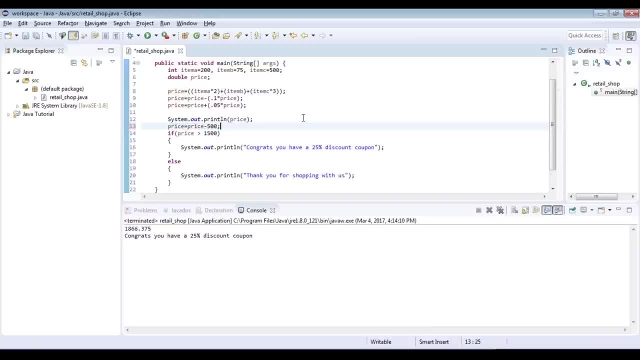 minus 500.. This is just to show you how the else statement will get executed. If I rerun this code again, then you can see: only thank you for shopping us is being printed. So originally he had purchased for 1,800, but when we are checking the condition, we 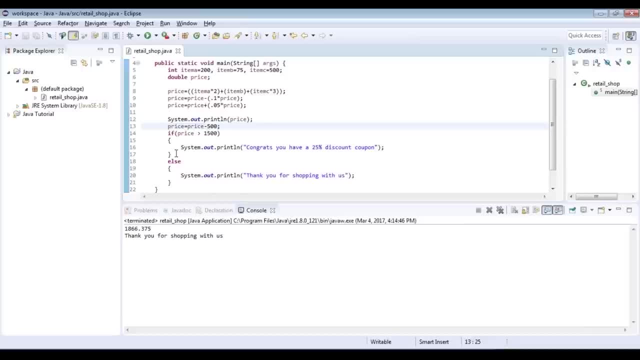 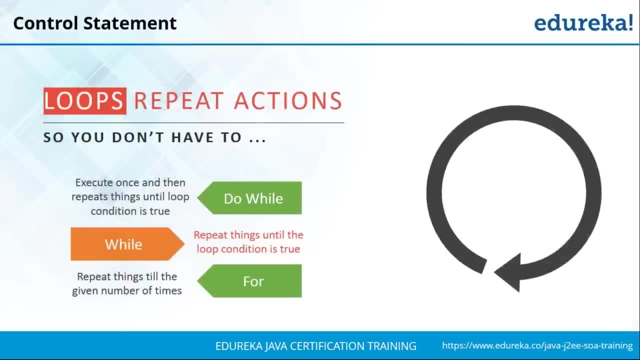 are subtracting for 500. Therefore, it is going to the else condition. So are you clear with respect to how the if else, All right, That's great. Now, moving on, we're going to talk about the various loops in Java. 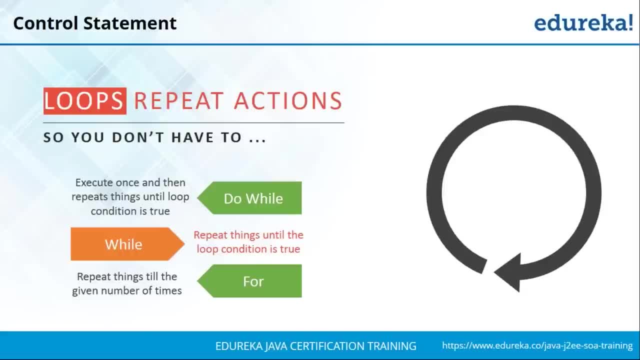 Now, the purpose of having loops in our program is to help us reduce the code redundancy. So what you want to do is, let's say, you want to perform a certain set of operations multiple number of times, then you're going to put it inside a loop state. 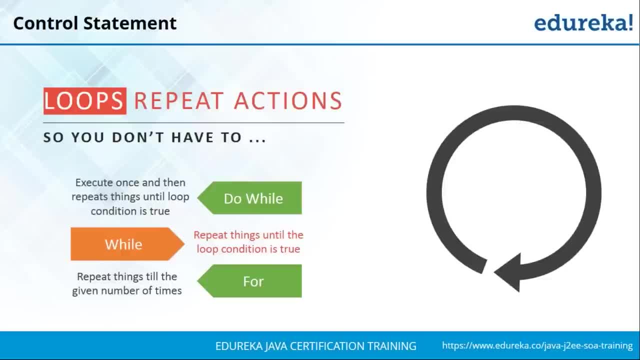 So, therefore, you don't have to write the code multiple number of times. The loop will execute it for any number of times that you wish. Now, when we talk about the various loops in Java, there are mainly three types of loops. You have the do-while, you have while and you have for. 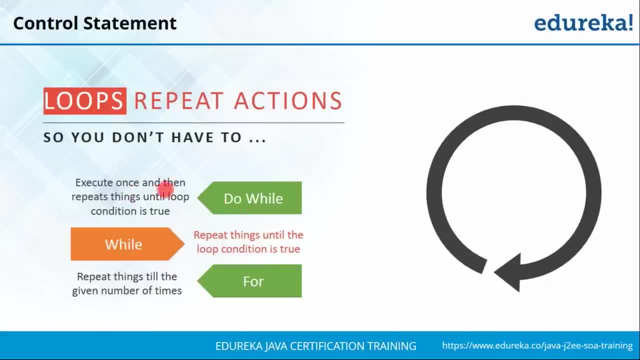 Now in the do-while loop, what happens is you execute the set of statements inside the loop once. then you check if the condition is true. If it is true, then you're going to go back and execute the condition till it becomes false. 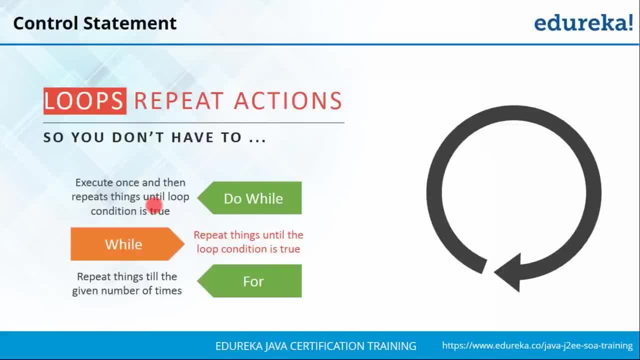 So basically, a do-while loop executes at least once and then only checks the condition. So it is an exit control loop Where you're controlling when the controller should move out from the loop state. Similarly, when you look at while loop, now while is quite similar to the do-while itself. 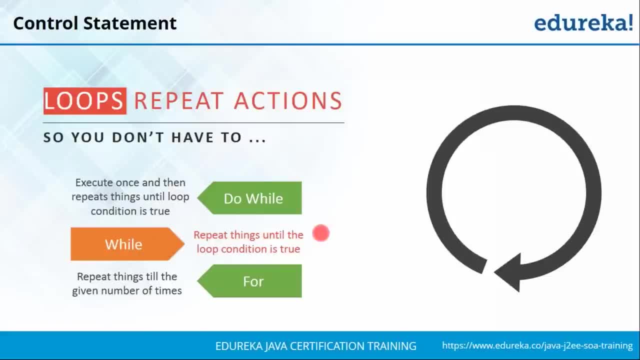 but the difference is in while the condition is first checked and then you enter loop statement directly. So you mainly use while loop when you're not sure of the number of iterations you have to perform. Now you use do-while and while loop mainly when you're not familiar with the number of. 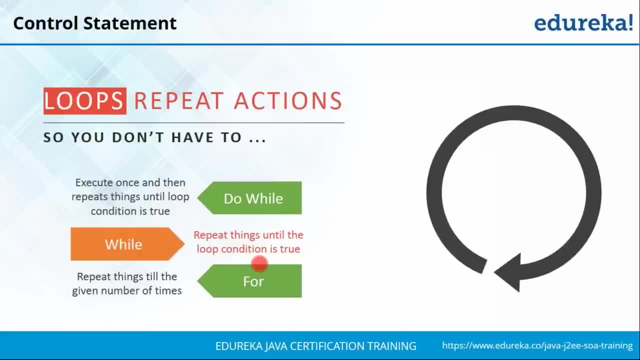 iterations that have to happen. So what happens is it runs for an uncertain number of times And once you've met your condition, then you come out from the loop statement. The only difference between do-while and while is that do-while executes at least once before. 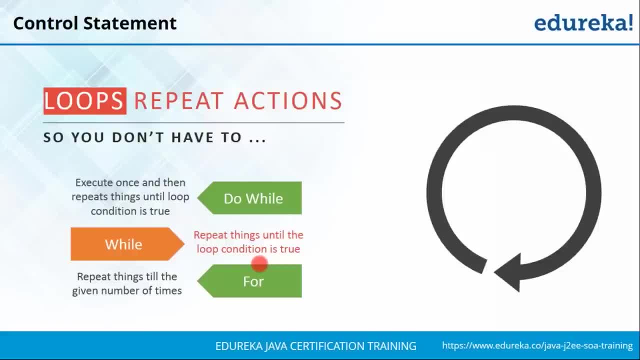 the condition is checked, whereas while checks the condition and only enters the statements After that, you have for loop. Now, for loop is also an entry control loop, but the difference being you're going to use the for loop when you know the number of times you're going to repeat something. 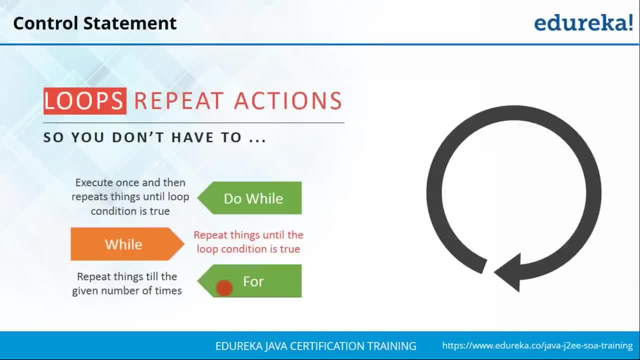 So let's say you want to execute a certain set of statements 10 times, then you can put it in a for loop And specify it has to run for 10 times. So I hope you're clear with respect to the three types of loops we have. 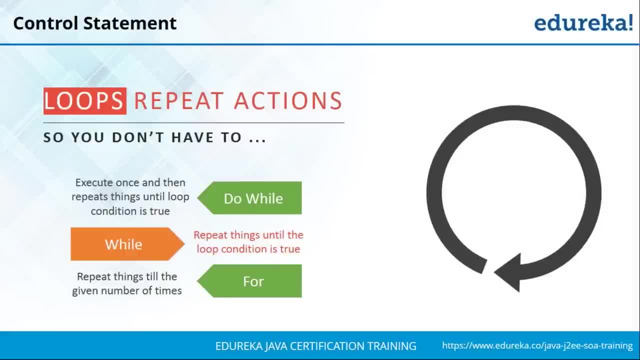 Okay, Divya is clear. So is John Ajay, Santosh Prashant Anna. That's great to see guys, So please let me know at any point if you're not following me or if you do have any doubts. 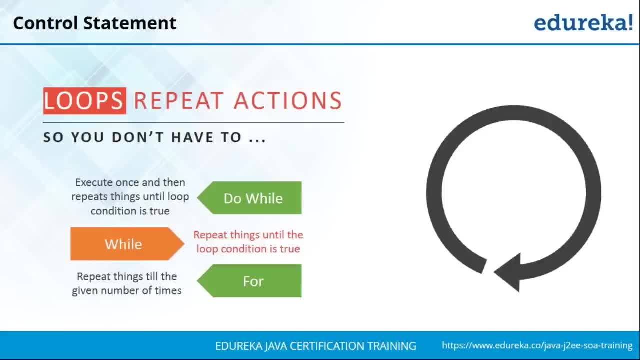 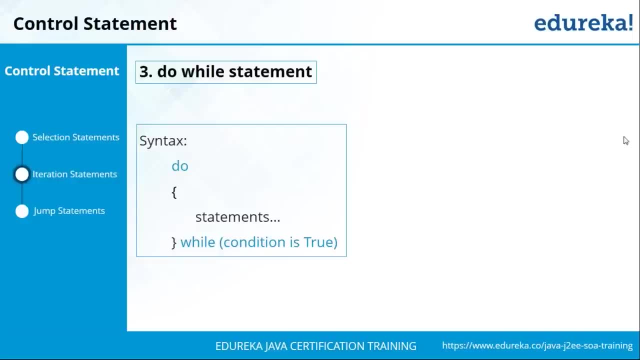 let me know. I'll be able to clarify them and their itself. Now, moving forward, let's look at the do-while loop. Now. the syntax for the do-while loop is quite straightforward: You're going to specify the keyword do first, and then you're going to specify this corresponding 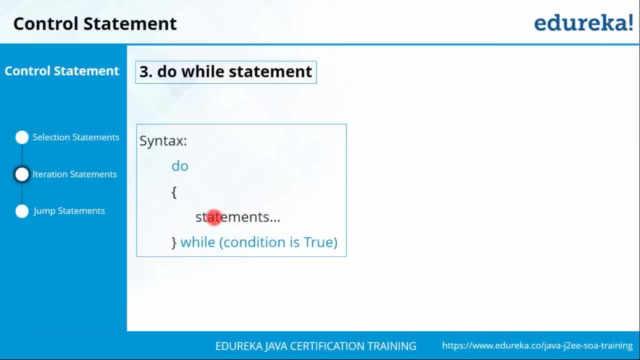 variable that you need to execute multiple times. So once the statement gets executed, only then do you come to the while part where you're going to check the condition. If the condition is true, then you go back to the do statement inside the loop and then. 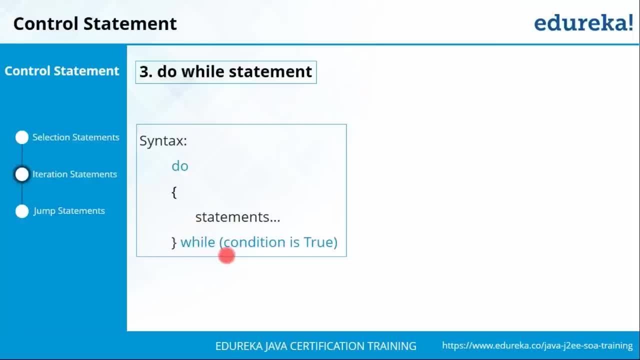 you execute that statement. Once you've executed that statement again, it comes out to the while you check the condition and then again, if it's true, it'll keep going back and doing the same until the condition is false. So you need to understand how the cycle works. 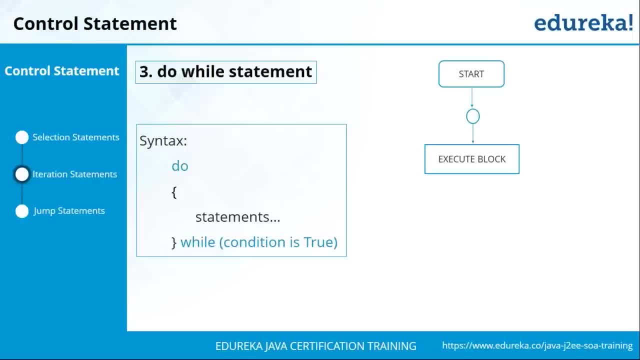 So let me give you an example for that. So you always start to a point and then you execute the block of code that you want to execute. This runs at least once. Then what happens is you check if the condition is true or false. 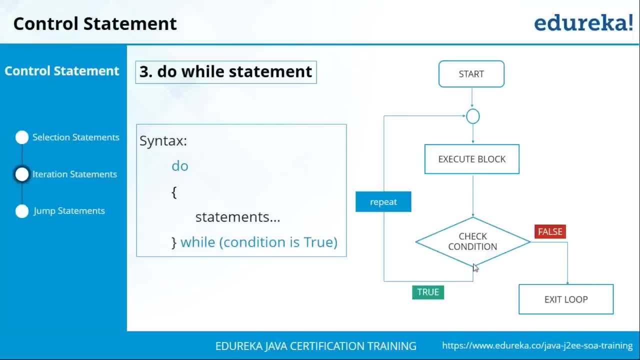 Now in case, if it is false, then you exit the loop, But if it's true, you're going to go back to the point of do and then you're going to repeat the same execution of the statements. So are you clear with respect to how a do-while statement works? 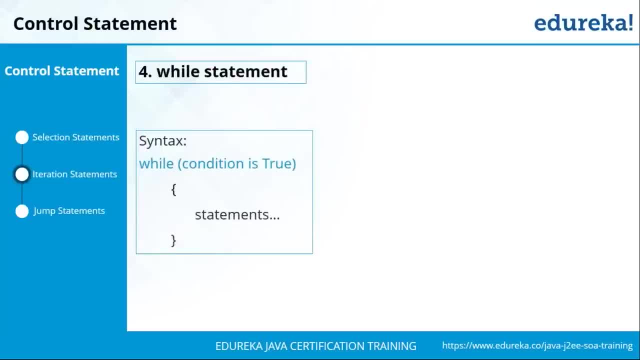 Alright. So after that we're going to look at the while statement Now. So with the do-while condition you had a first do, then you execute the statement and then you check the condition. But here what happens is first itself while checks if the condition is true. 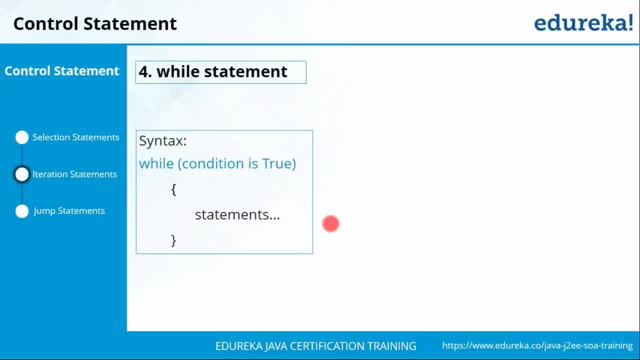 Only if it is true does it enter and then execute the following statements: So every time before you enter the loop you're going to check the condition is true or false. So you're going to start the prod and then you're going to check the condition- straightforward. 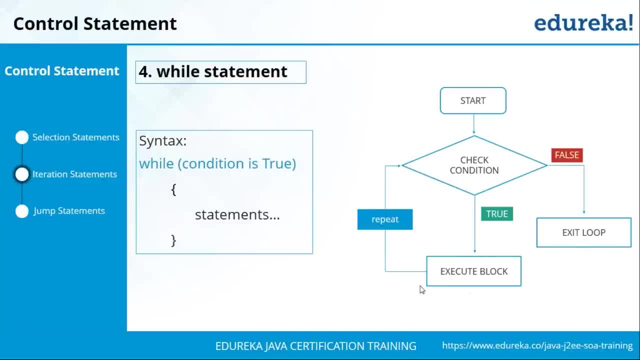 So if it is false, you're going to exit from that loop, But if it is true, then you're going to go back and keep repeating till the condition turns false. I hope you have understood how the while loop works and the difference between do-while. 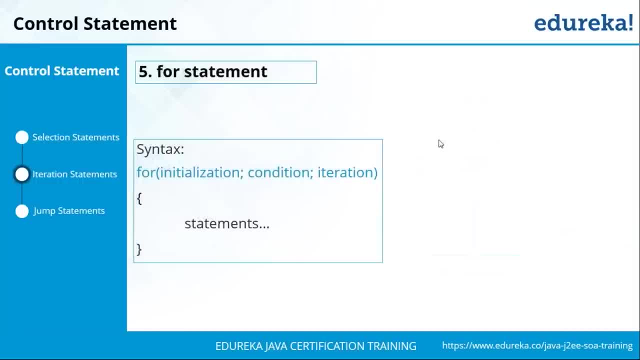 and while loop. Alright, Now, finally, we have the for statement. Now the for statement, as I have mentioned, is used when you have to run it a limited number of times, So the syntax for for is slightly different. Here you're going to have three major concepts. 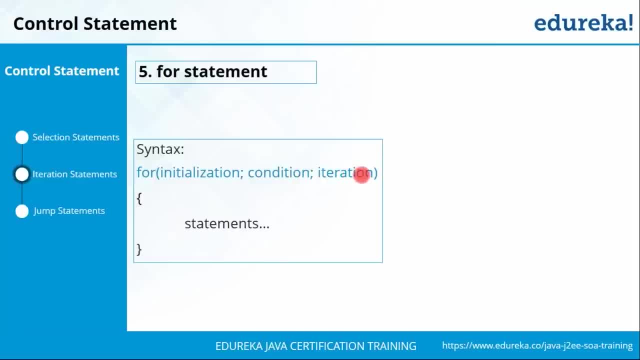 You're going to have an initialization, you're going to have a condition and then you're going to have an iteration. So, basically, what happens is you initialize a variable here to the value that you want, then you're going to specify- You're going to specify- the condition based on which it is checking. 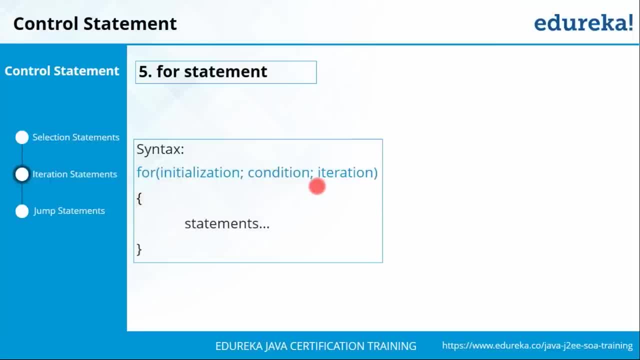 And finally, you're going to specify the iteration. So let's say you want to execute a statement five times, then you can initialize the variable value to one, then you can check if it is less than or equal to five, and then you can. 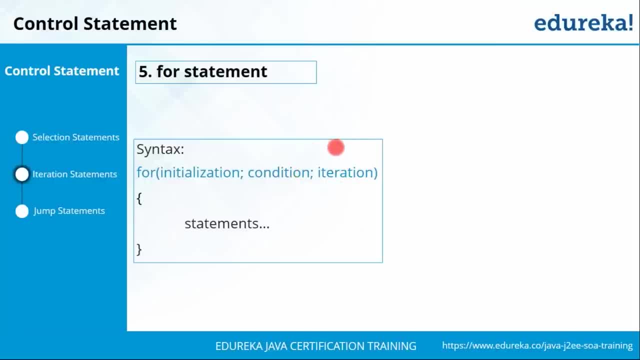 always iterate it using an incremental operator. So for five times the statement present inside will get executed. So again, if you look at the flow of for loop, you can start the code. You first begin by initialization, then you move forward and check the condition. 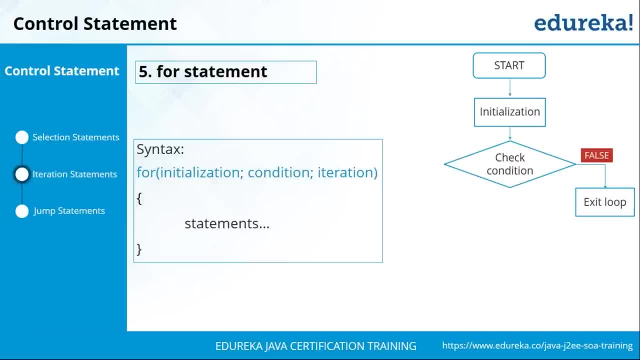 Now, If the condition is false, then you exit the loop, But if it is true, you will execute the corresponding statements. Once you've completed the execution of the statements, then you go ahead and iterate the value and go back to checking if the condition is true or false. 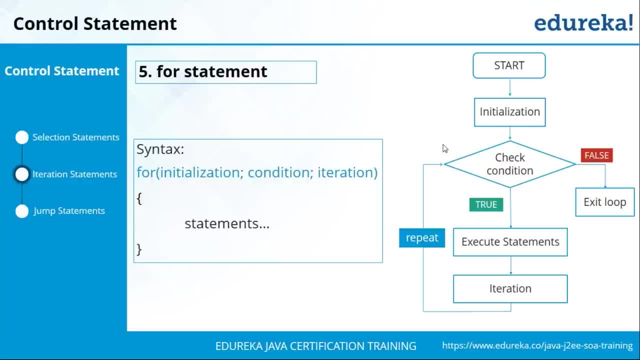 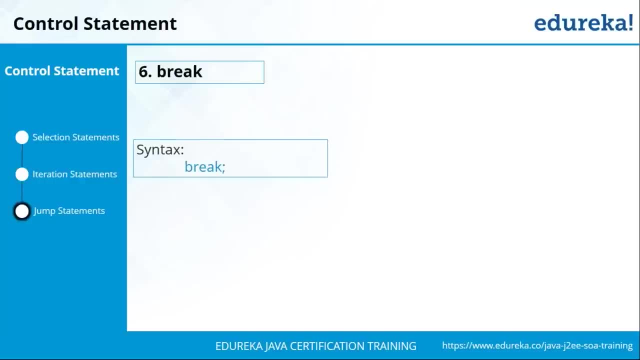 So are you clear with respect to how the do, while and for loop works. Now, don't worry, I'll be giving an example to understand each of these loops, one after the other. Now, finally, you have the break state, So let's say you're. 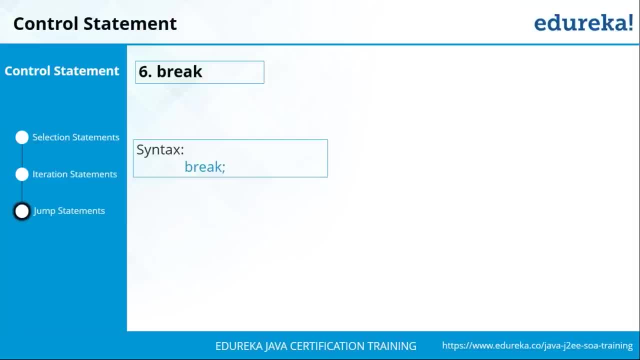 Not going to run a loop for infinite number of times, but there should be a point when you need to leave out from that loop, And that is exactly why the break statement comes into picture Now. using the break statement, you can leave the control of the loop when a specific condition 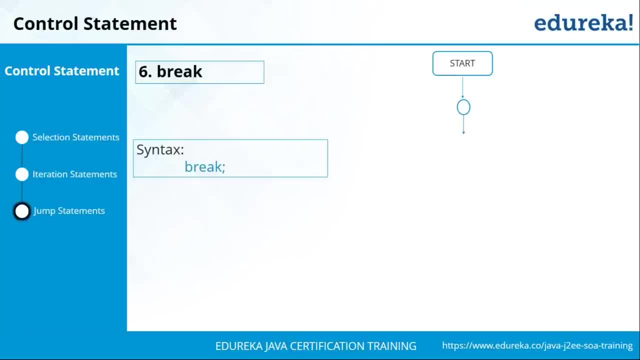 is met. I'll show you a flow of this that'll give you a better understanding. Now you start execution of your code. then you're going to check the loop condition. So basically, you're going to write a break statement inside a loop, or you've seen it? 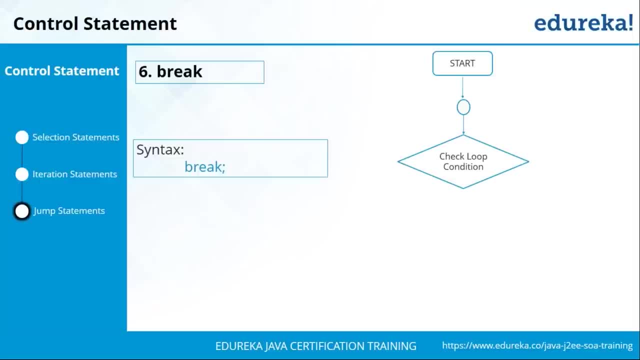 earlier, also in the switch case condition, Now in the switch case statement. So what happens is that if a case is executed, then you break out from the control of the switch case and that's where you use break. So what happens if you do not use a break statement inside switch case is that every 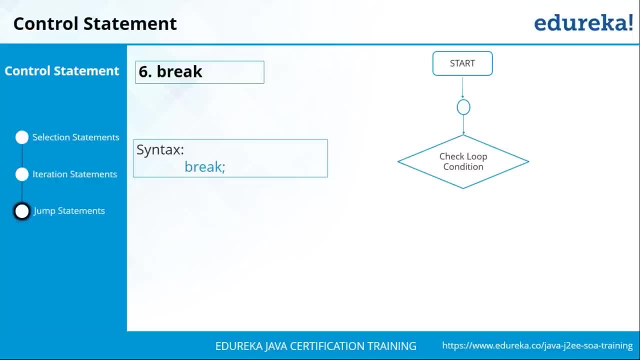 corresponding case after the case you wanted will get executed. So I'll show you the example for that as well, but for now let's try to understand this. So once you've checked your loop condition, if it is false, you'll exit from the loop. 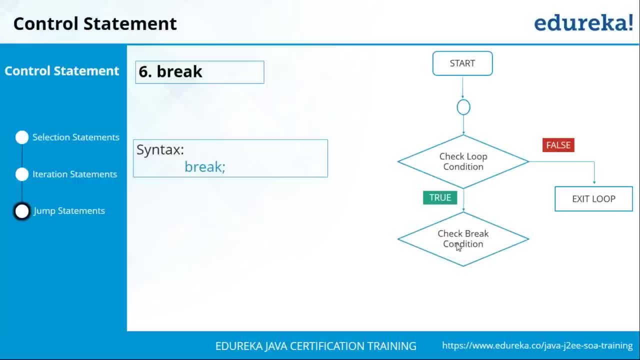 But if it is true, you'll come down and you'll check. if the break condition is true- Let's say it's going to be true- then you're going to execute from that loop. But if it turns out to be false, then you're going to execute the statements that are remaining. 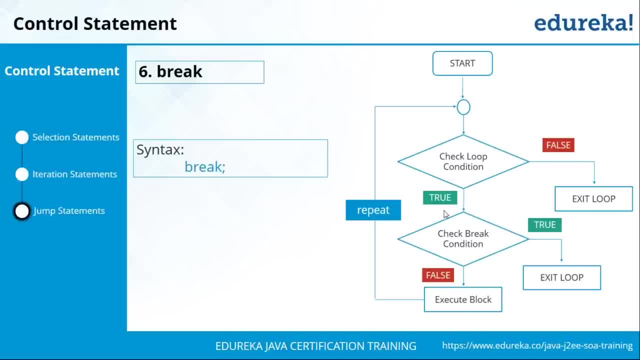 in the loop and then go back to repeating that loop. So every time while the loop is getting executed, you're going to check if the break condition is met. If it is, you leave from the loop. and if the break condition is never met, then you'll. 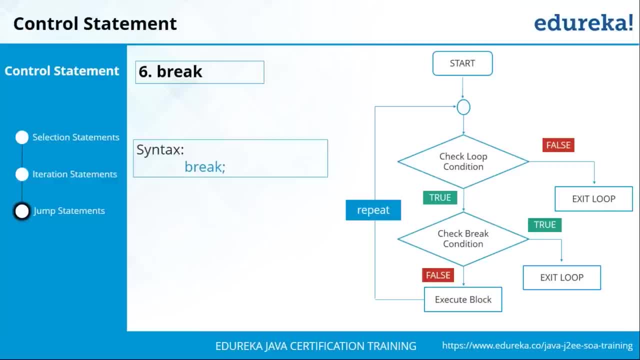 exit from that loop as well once you've completed the execution of that loop. But opposite to the break statement is the continuous statement. Now, with continuous, what happens is that Every statement that is after the continue keyword does not get executed if the continue. 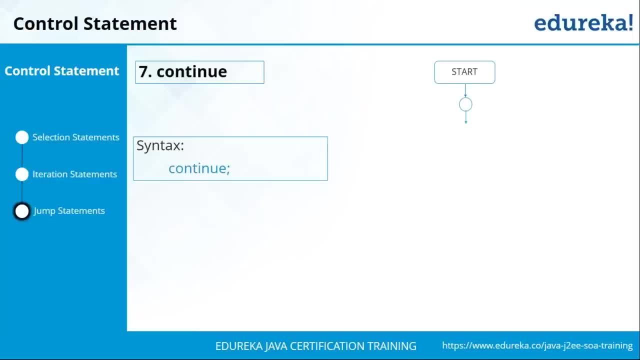 keyword is true- So let's say you're going to start execution of a program- then you're going to enter the loop condition. If it is false, you're going to exit from that loop, and if it is true you're going. 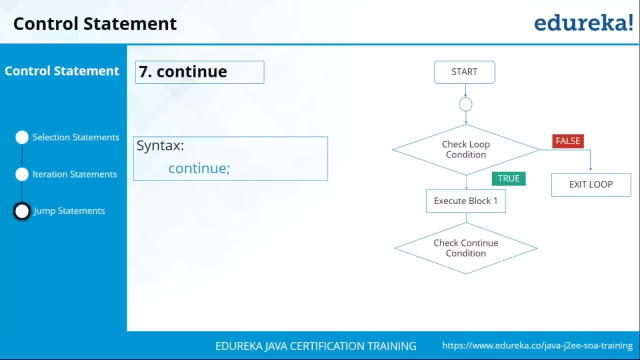 to execute a certain set of codes. Now, in between these codes you have your continue keyword. So if the continue condition is considered to be false, then every statement after that will get executed and you will go back to execution of that loop. 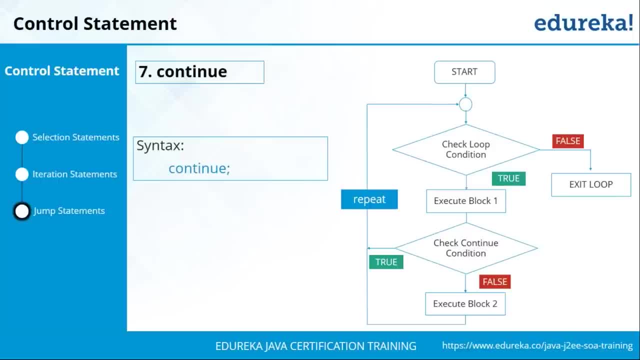 But let's say it is true. If it is true, then what happens is that every statement that is after the continue keyword does not get executed in that iteration of that loop. So every time a continue keyword is found to be true, the execution of block two does. 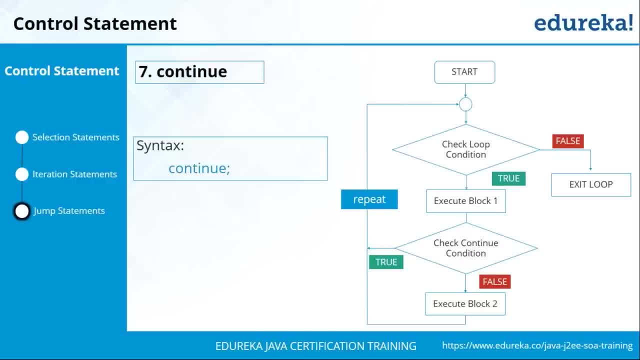 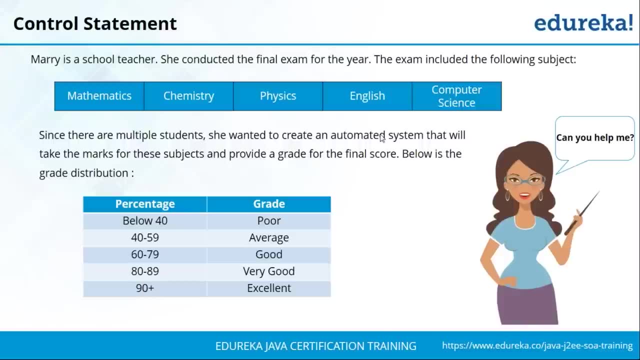 not happen. So I hope you're clear with respect to how the break and continue statement works. Now, to give you a better understanding of how the loops works, let's look at a use case here. Mary is a school teacher. She's conducted final year exams for her students for five different subjects. 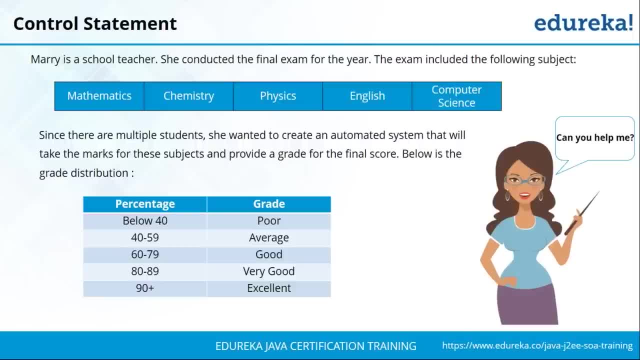 Now, as there are multiple students, she wants to create an automated system that will take the marks of each of the students, calculate the final score and then give a grade distribution for these students. So she's also given us a grade distribution chart here. 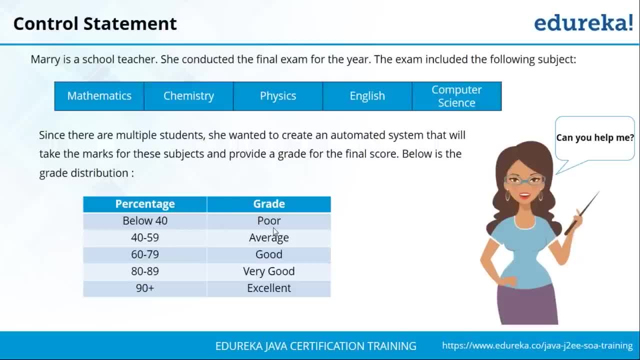 So if the student has scored below 40%, then he's going to get a poor grade, But if he scored 40 to 59, he gets an average. Similarly, 60 to 79 gets him good, 80 to 89 gets him very good and 90 plus gets them. 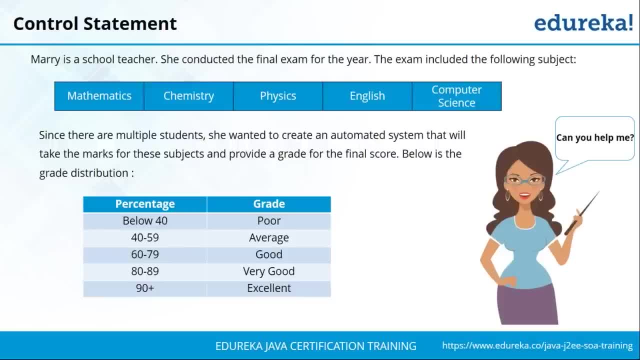 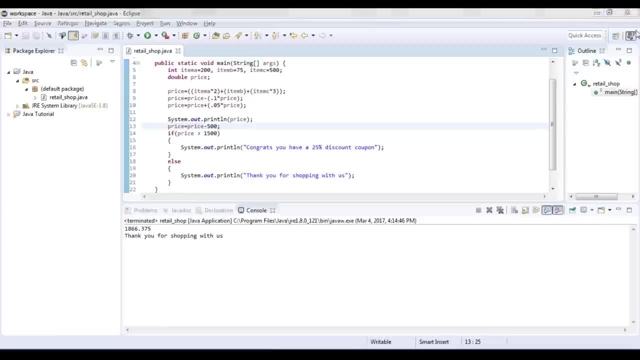 excellent. So we're going to write a Java code that makes use of loops as well as control statements to achieve this. So let's see how it's done. For this, I'm going to create a new file To do that. you can either go back to your project, right-click and select new option. 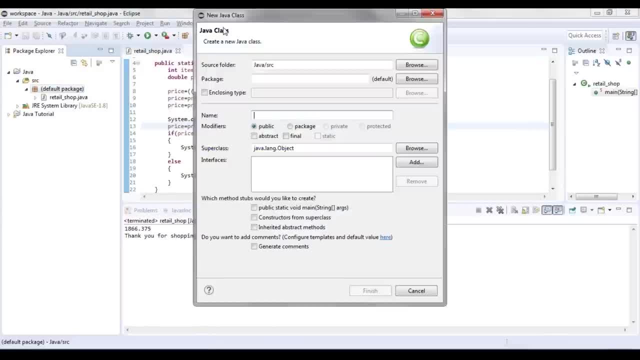 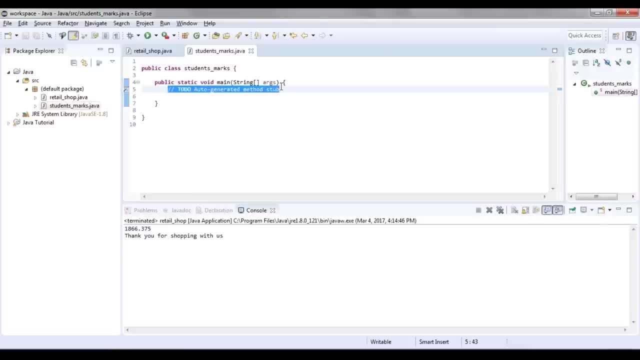 from there or you can directly click on the new class option here. Once you've set the name, click on finished and you have your new class created. So I basically have five different subjects for which I'm going to take the marks. 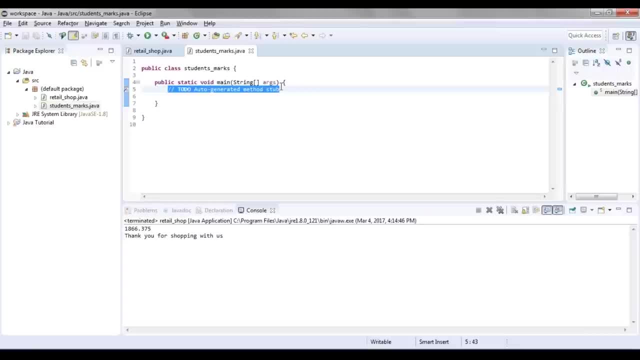 So I'm going to assume the marks. The marks are going to be in whole. so what I'm going to do is that I'm going to consider the marks to be integers. So int. we had maths, physics, then you had chemistry, English and finally you had computer. 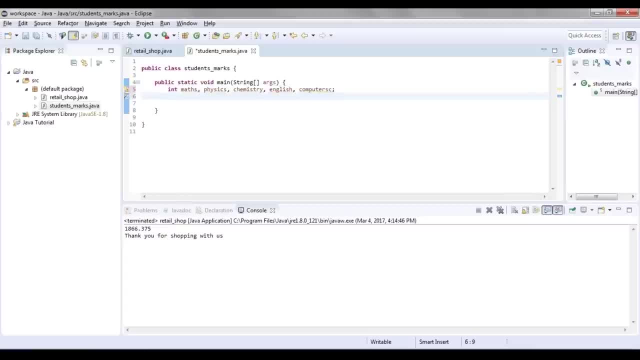 science. Now I need to store the total marks somewhere, so I'm going to declare a double variable. that is final score. So now it's time we begin with our looping statement. So what I'm going to do is that I'm going to start off with a do while statement. 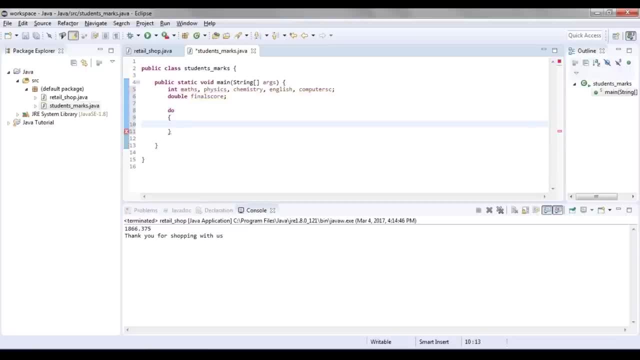 I'll say: do then open parenthesis and then enter into it. So always make sure, when you're writing a code in Java or any programming language for that instance, you follow the indentation, because this will also help you identify where you've gone wrong and whether, if you've missed any parenthesis or such, 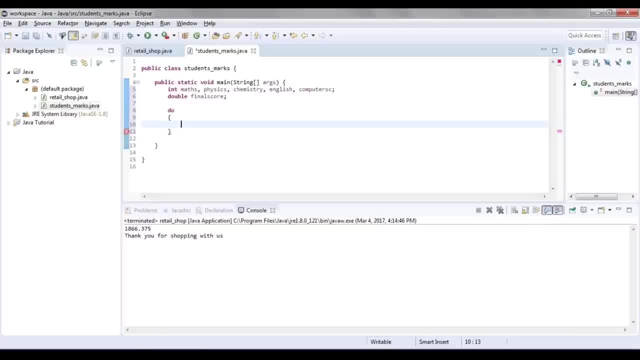 So always follow the indentation rule. So the first thing what I'm going to do is that I'm going to take the subject-wise marks for each student. I need to take the match marks first, So this statement will request for the marks for match. 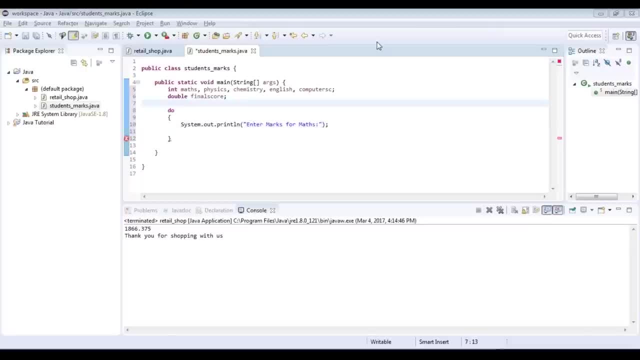 It'll print out a statement that says: enter marks for match. Now it's time we go ahead and take the input from the user. Now, before you go ahead and take the input from the user, there's one thing that you need to do is that you need to create an input object. 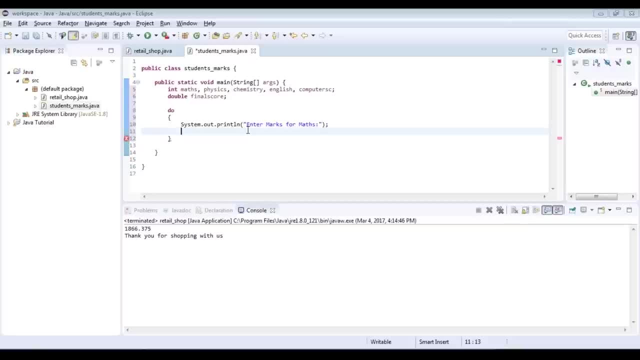 So I've already discussed this with you. everything that we do in Java is through objects as such. Now, to create an object for taking input, I'll show you the syntax: it's going to be scanner, followed by the variable name through which you're going to take the input. 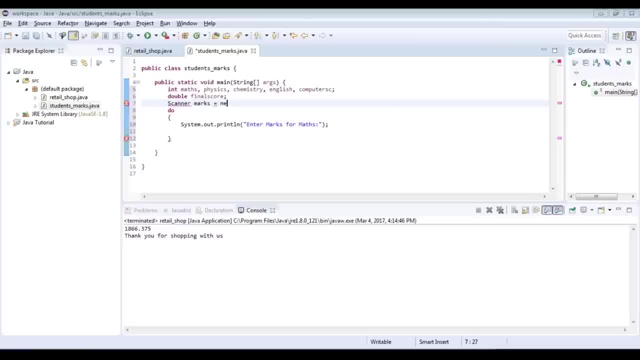 So in our case, I'm going to call it marks equal to new. Now, new is a keyword through which you're going to create a new object, So new, and then you have to specify the original class to which it belongs. So that's again: scanner here. 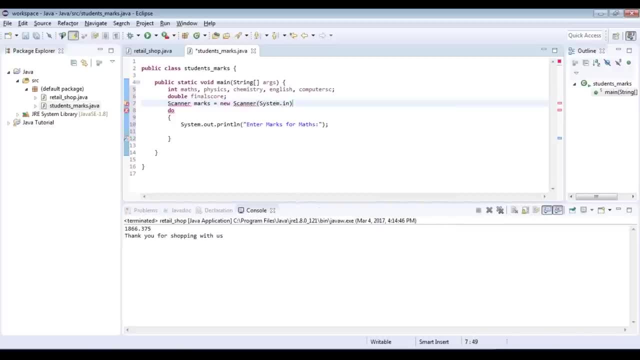 And then you need to specify system in Now. you need to specify the class to which it belongs, So that's again scanner here- And then you need to specify system in Now. this is one of the statements through which you're going to create the object. but 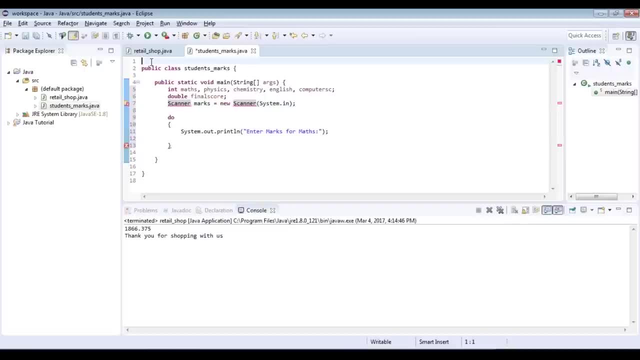 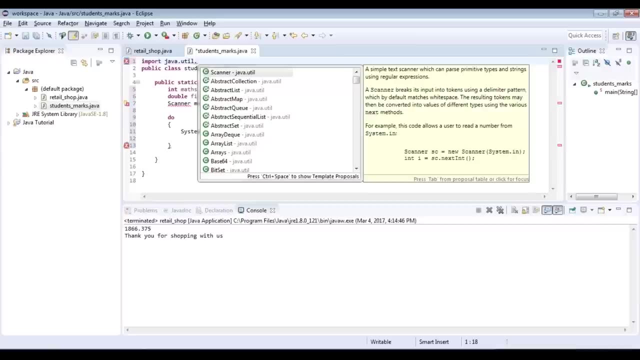 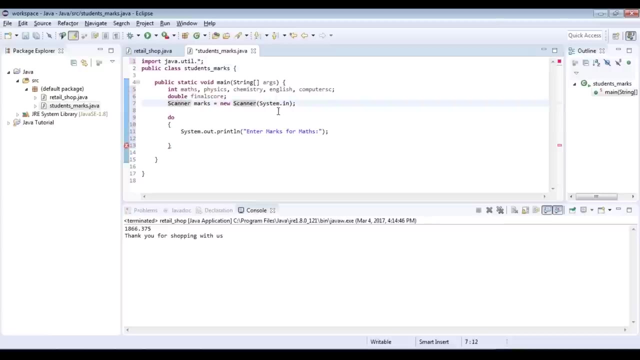 before that you need to import a certain package from the Java library. So to do that, just type import javautilstar. Now this basically imports everything from Java's util package. Now, once you've done that, you can use the scanner function. 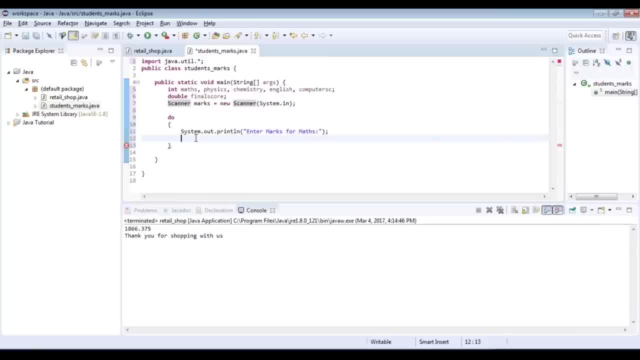 So, to take an input from the user, what you need to do is specify the variable in which you're going to take the input. So in our case- I'm going to start off with- maths is equal to the object that is used for input. 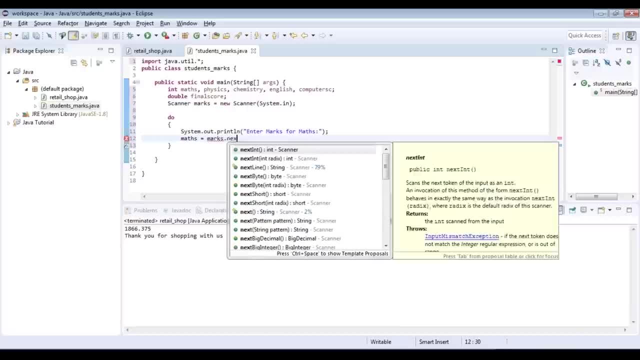 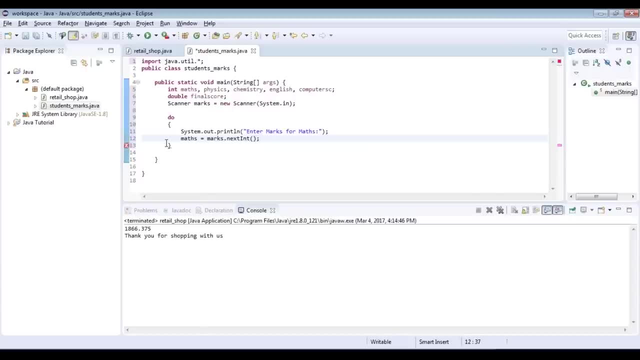 So in our case it's marks dot, next int. So what this basically means is that the next integer value that is being given by the user should be taken and stored inside maths. So are you clear on how to take input from the user in Java. 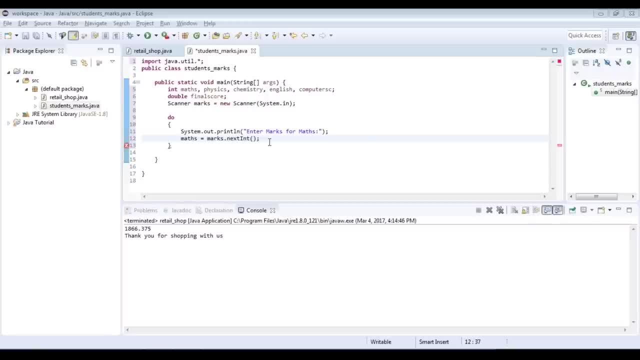 Okay, Prashant is clear. so is Bharat, Henry. Dave, That's great to see. Now I'm going to take marks for the next five subjects, So rather than typing it out, I'm going to just copy paste this: 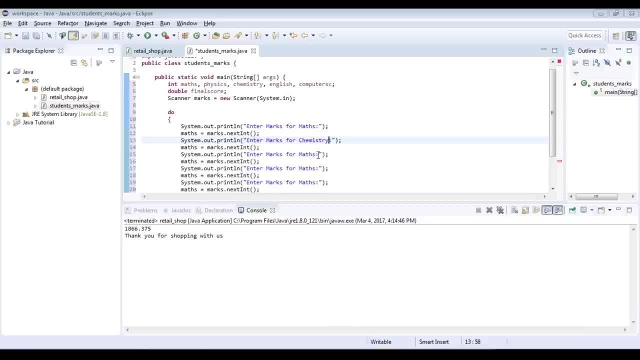 So maths. after that you have chemistry, You have physics, You have English And finally you have computer science. Change the corresponding variables as well. Now, this is for chemistry, so let's rename it to chemistry. The next one was for physics. 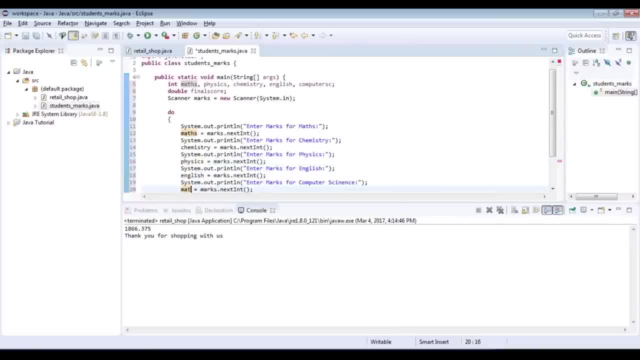 Then we had English And finally computer science. So with this I have taken the marks from all the students. So now it's time I go ahead and compute his final score. Now to do that, what you're going to do is that you're going to write. final score is. 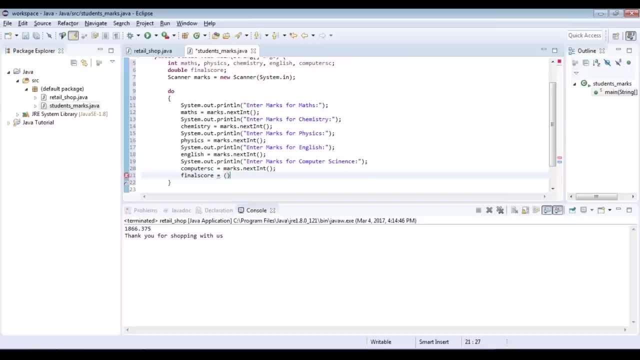 equal to. Then you have to add all the marks and then divide it by five, since we have five subjects. So let's add each of these marks, That's maths Plus English, Plus Chemistry, Plus Physics And finally computer science. 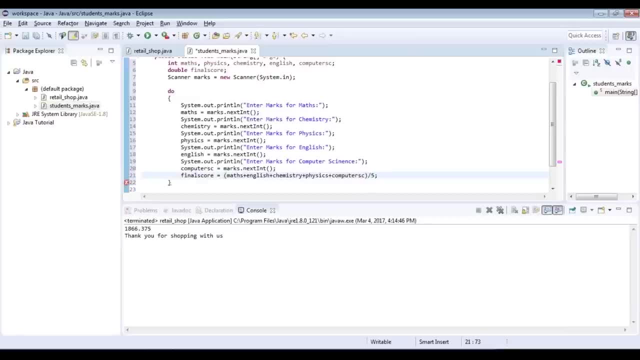 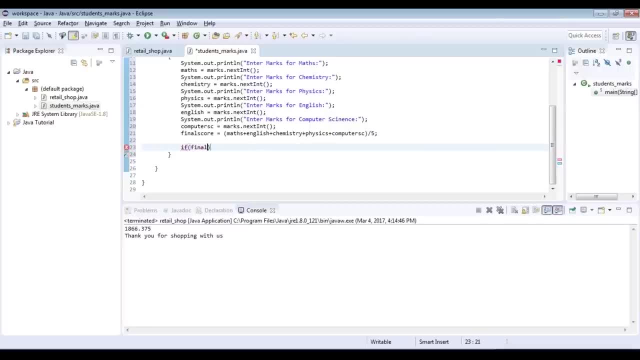 Now, the first thing that we're going to do is we're going to create an if-else grade. So we're going to create an if-else ladder for this. So if my final score is greater than 90, then he's going to get excellent. 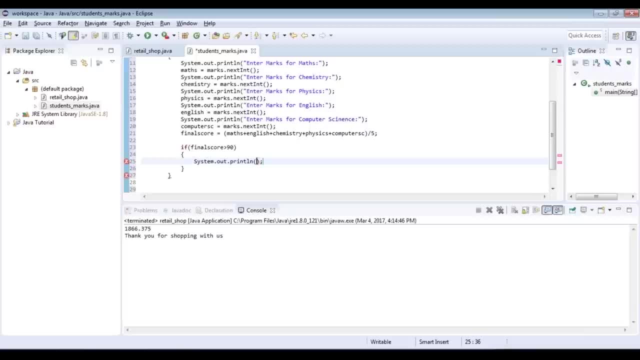 I'm going to say else. if That is, if the first statement is not true, then check Final score: greater than 80. So, if you remember, So if you remember, the second statement was between 80 to 89. Now, if it is not greater than 90,. 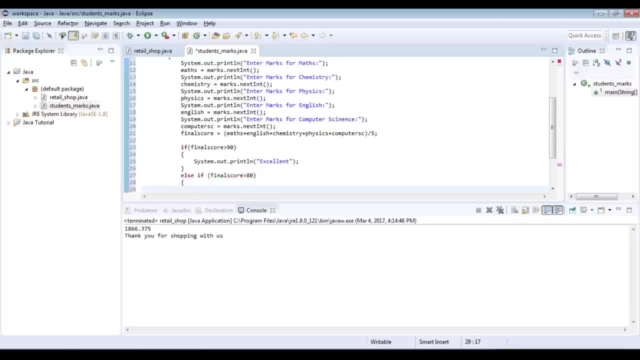 only then will it come to else, if part. So here I'm gonna say: very good Again, I have another else if Else, if final score is greater than 60. And if it is greater than 40, then I'm just gonna print average. 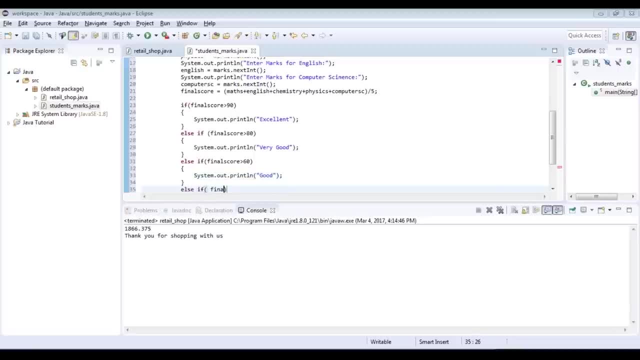 Then you have another else. if where, if my final score is greater than 40, then I'm just gonna print average. Now, after this, I'm not gonna write an else. if ladder, I'm just gonna write else. The final result, that is, if he's got below 40%. 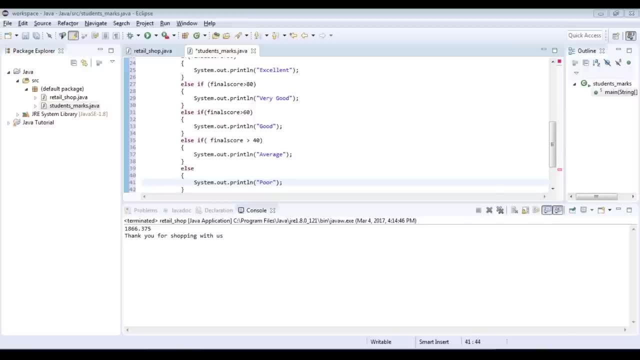 that is poor. Now, here what we've done is that we've used the if-else ladder and specified which grade to get in case of a specific range. So now what you need to do is you need to still specify the while condition here. 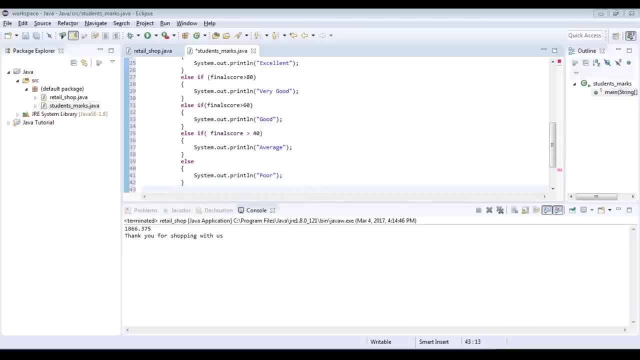 But before that, you need to understand when to exit from that. Now for that, what I'm gonna do is that I'm gonna write an output statement. We're gonna set up right here, let's say, an output statement. Let's go to our Kotlin window to correct it. 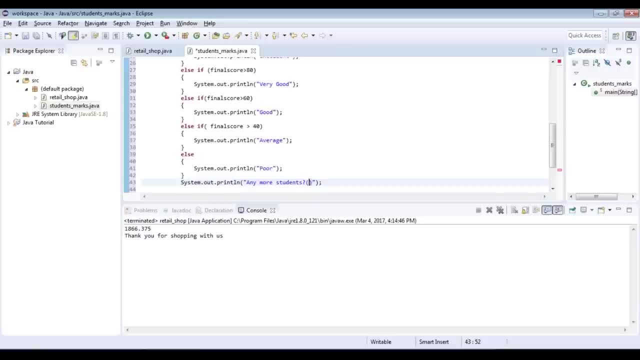 You can also see here. let me show you how. So we're gonna go to Kotlin and we're gonna set up a value in the native field And I'm gonna leave it at 10.. So we're gonna go to Kotlin. 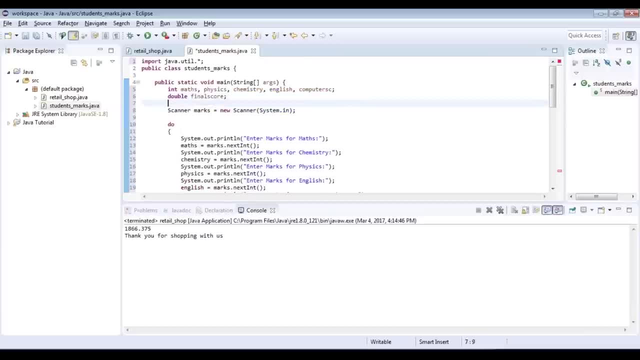 and we're gonna set up our new variable. We're going to set up a new variable here And here I'm gonna say: if last word and the variable class is equal to 10, then I'm gonna set up another variable. 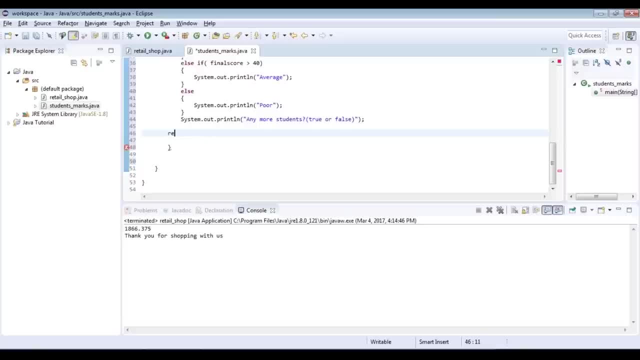 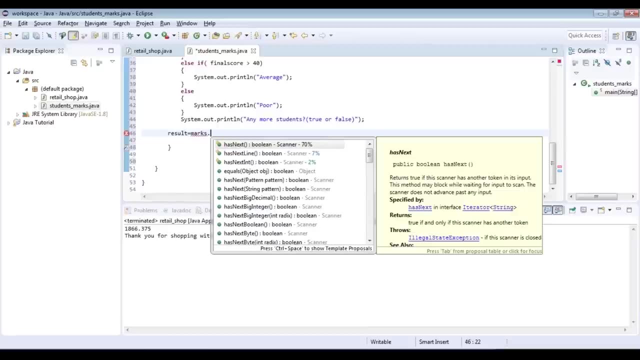 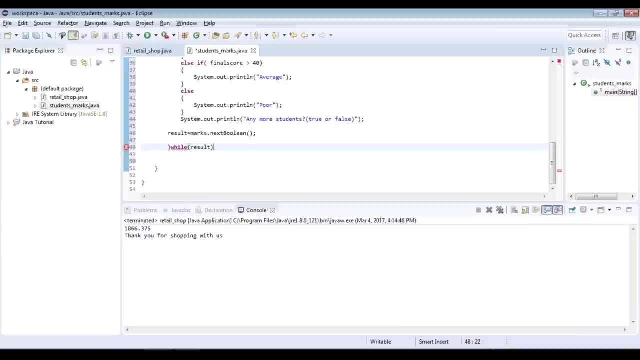 And I'm gonna set up a new variable. So I'm gonna go back to Kotlin and I need to know Again: use our input variable, that's marksnextBoolean. That is, the next Boolean value that is inputted should be stored inside result. That is, while my result statement is always true, keep executing this statement. 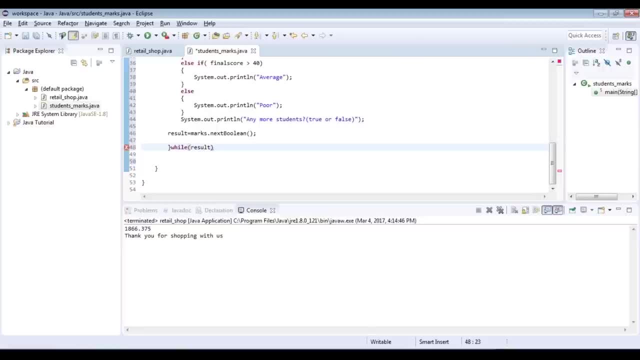 So when you say while result, it basically means till the time my result value is false, keep executing the set of statement. So any questions till here on how we've used the if-else ladder or how to use this do-while loop? 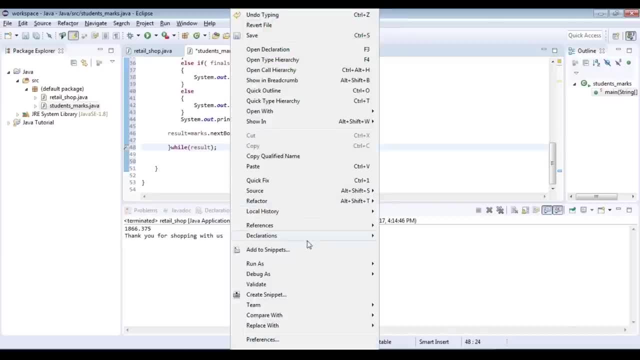 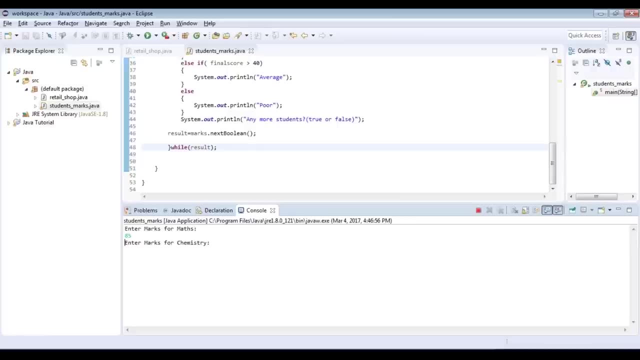 Alright, repeat. So let's go ahead and execute this program. So it's asking me to enter the marks for maths. Let's say 85, then chemistry is 47,, 56,, 75,, 92, and then you get a grade that is true. 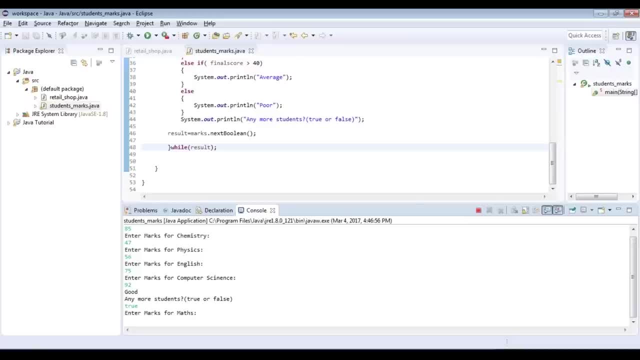 So in case, if I say true, it's gonna again ask me the marks for maths. So again, let's do it. Let's go with 75,, 84,, 92,, 48, 56, and then you can see the corresponding result. 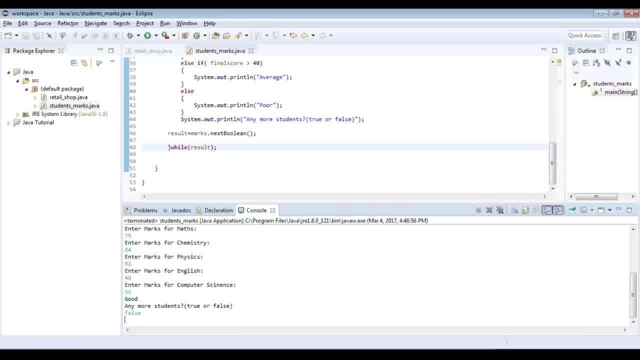 So finally, let's say, if I want to say false, it exits from that program. So are you clear with respect to how the do-while loop is executing? Alright, now, same thing can be also changed to a while loop. Now, all you need to do is that you need to remove the while from here. go back to where. 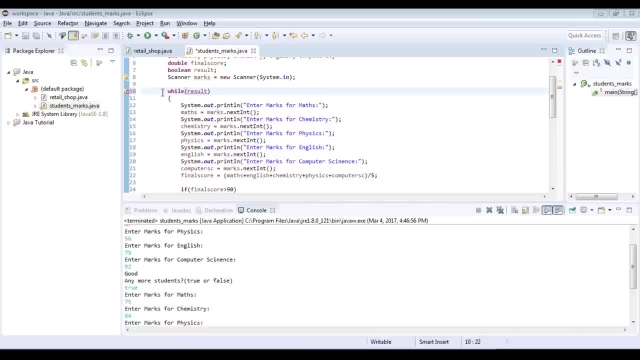 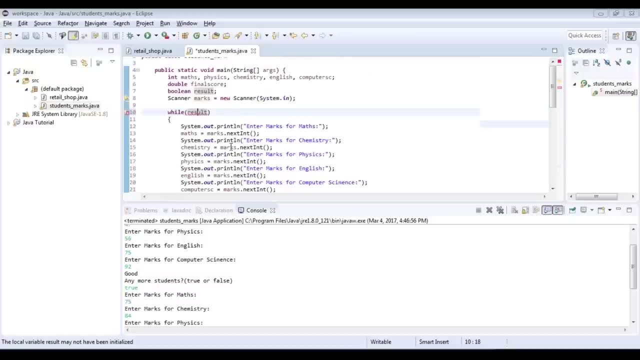 you've written, your do go there And then mention the while loop. So here what is happening is that first you're checking the result and then you're gonna enter this loop. Now, before you go ahead and enter this loop, this value has to be assigned to be true. 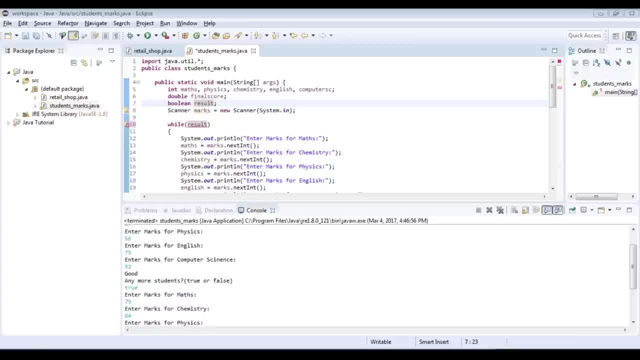 Because until and unless the statement is true, it will not enter this condition. So what I'm gonna do is that I'm gonna initialize it to be true and then I'm gonna begin the execution of the statement. So are you clear with respect to how do-while and while differs between both. 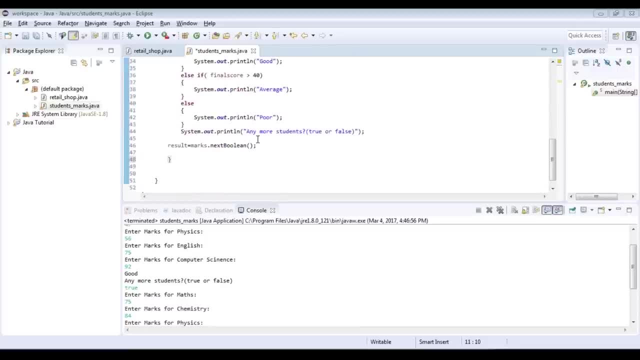 So here, basically, it will run infinite number of times till you're gonna enter a false value. But in the previous case it's gonna execute at least once and then it'll ask if you have any specific values and keep running till you enter a false value. 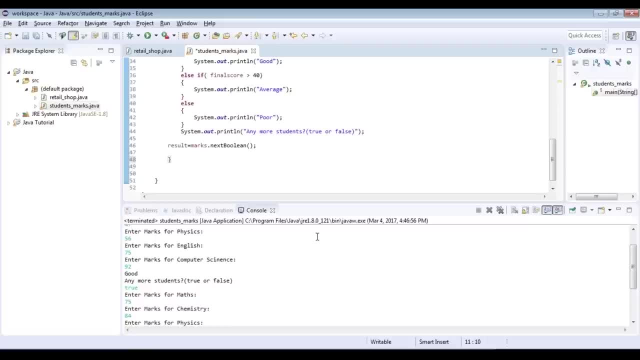 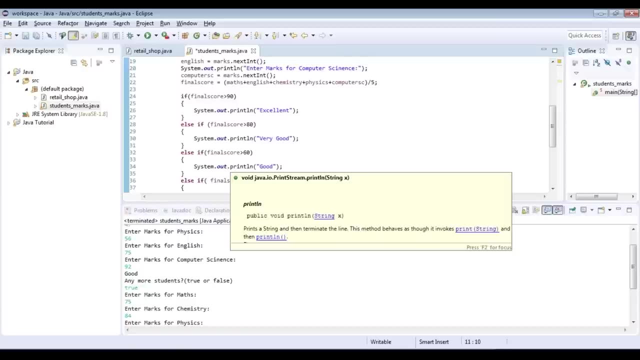 Now in the do-while loop it executes at least once. but the while loop will execute only if the condition is to be found true. Now, in the same case, let's say you know the total number of students beforehand itself, Then what you can do is that you can use a for loop here. 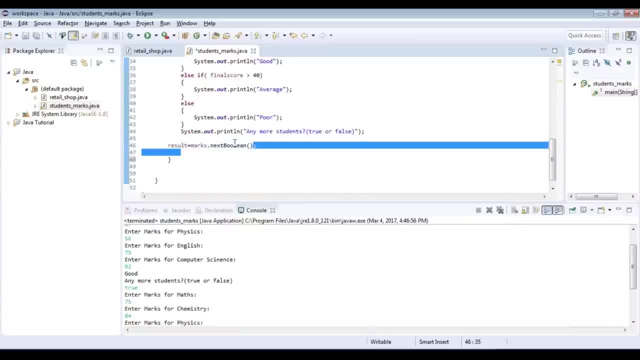 So what I'm gonna do is that I know the number of students. so I'm gonna remove this last statement from here And, before I enter my loop, what I'm gonna do I'm gonna ask the number of students. Once you have that, you're gonna assign it to a corresponding value. 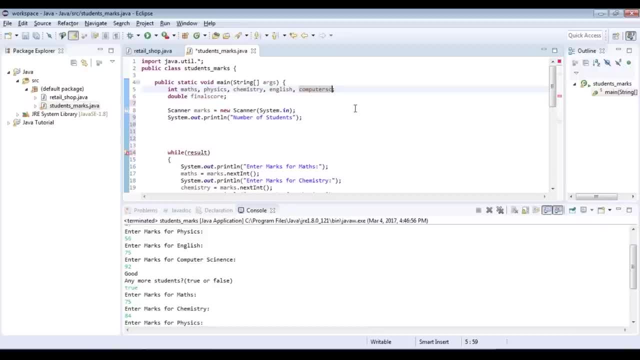 Since I don't need this, I'm gonna remove it. Let's say: here I have another integer value, that is student number. So again, let's say student number is equal to my marks. Okay, Next dot, next enter. That is the next integer value entered should be my number of students. 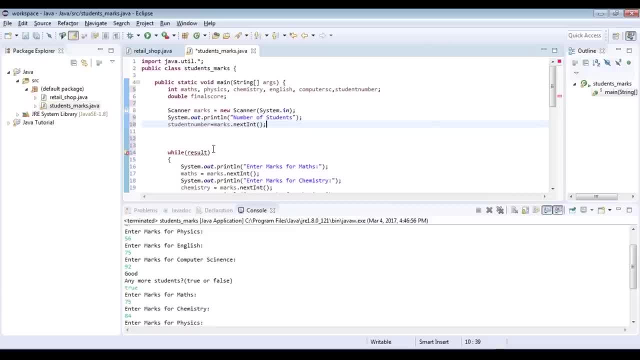 So with this you've already established the total number of students for whom you wanna enter the results. Then you're gonna go ahead and execute the for loop. If you remember the command for for, it is for, and then you begin with your operation. 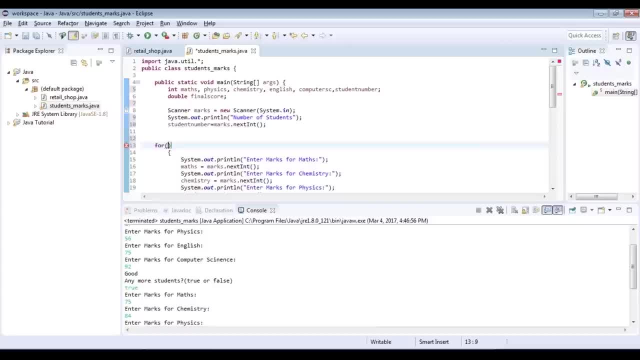 So here you need to start with initialization. So I'm gonna use a variable known as i, which will increment its value and always keep comparing with the number of students. So let's say int i equal to zero, because always the numbering in Java programming be. 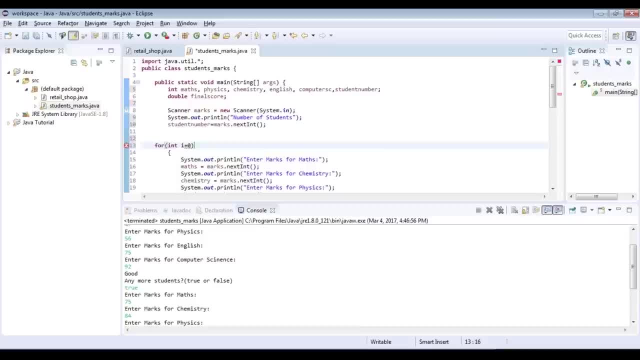 it the numbering of array, be it the number of looping, everything is suggested to start from zero. The counting system in Java or most programming languages, starts from zero instead of one, So it's always recommended that you start from zero Now, for i is equal to zero. 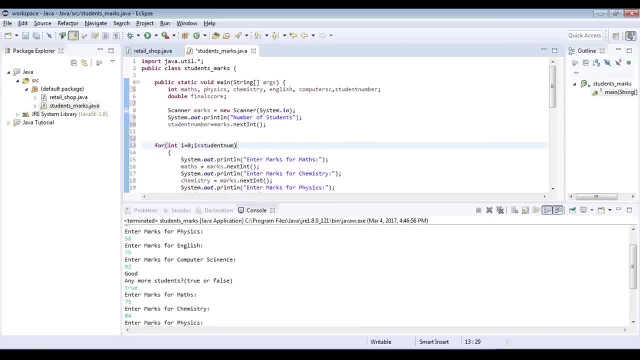 i less than student number. And after the execution of each statement, I wanna increment the value of i by one. So i plus plus. So any doubt with respect to the syntax of the for loop? Okay, Prashant is clear. so is Bharat Sandeep Santosh. that's great to see, guys. 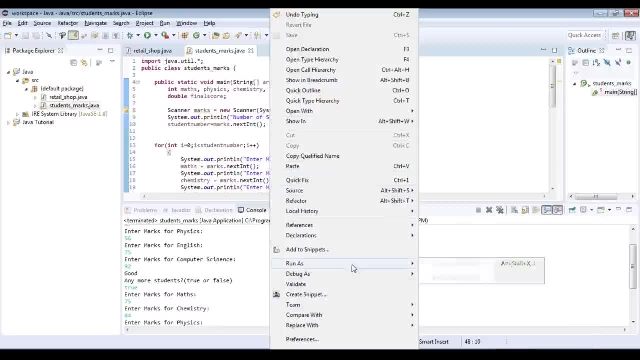 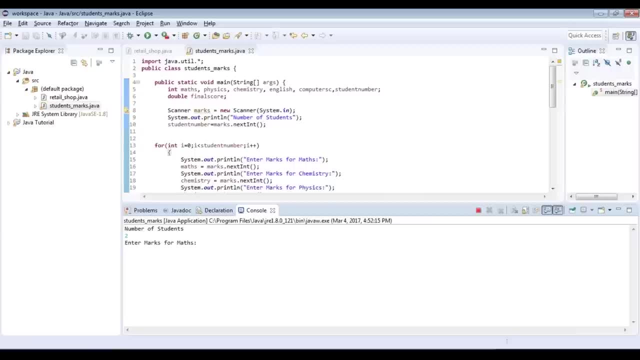 So now let's save this and re-execute this code once again. So run as Java application. You're gonna ask the number of students. let's say two, enter marks for maths. So you've got your result for first student. let's try it again. 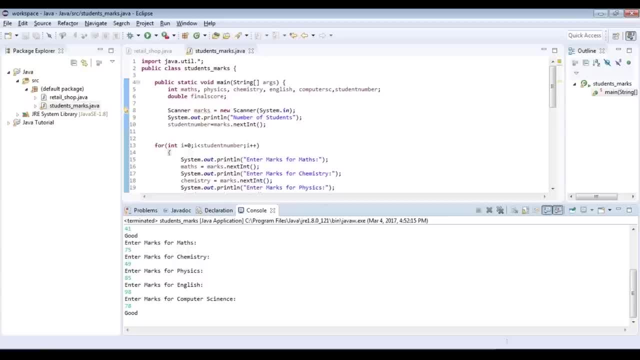 It's got good and then you can see it has exited from that loop. So our loop has run twice. So any questions with respect to how the for loop works, or the while or do while? Okay, so now that everyone is clear with respect to how the for and do while loop works. so 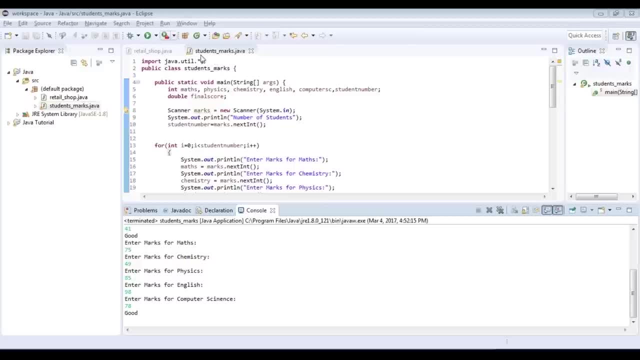 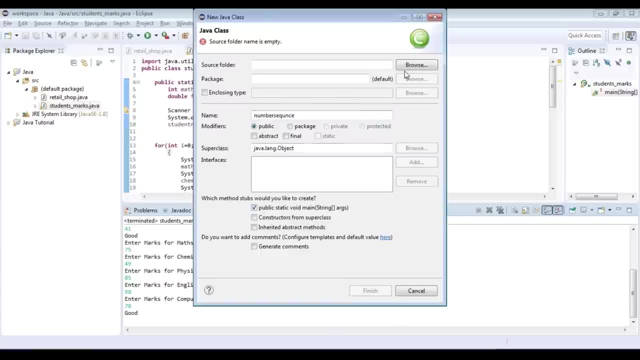 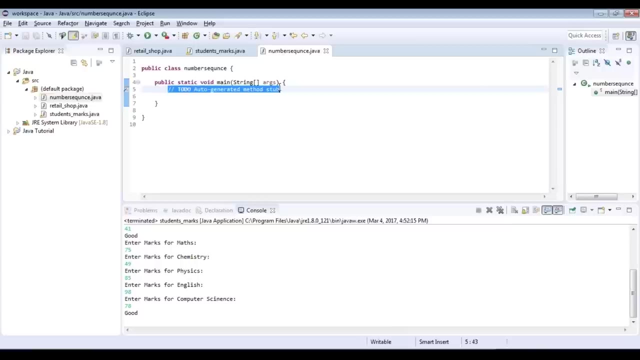 now let me show you another program where you're gonna be using both break and continue. Let me create a new class. let me call it number sequence. So here, what I'm going to do is that I'm going to run my for loop 50 times. 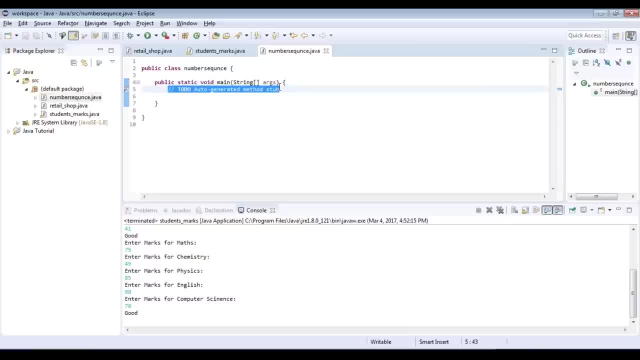 But inside my for loop I'm not going to print even numbers And in case if my number crosses 20, I'm going to break out from that loop. Let me show you how it's done. So let's say: for i equal to 1.. 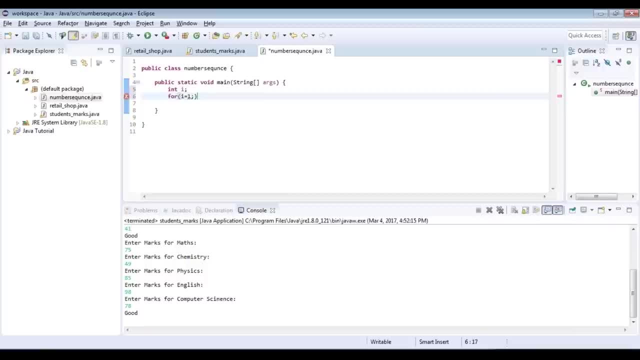 Now, in this case, my counting has to start. Start from 1, because I'm going to check from 1 to 50.. i less than equal to 50 and i plus plus. Now, inside this, you need to specify both your break and continue statement. 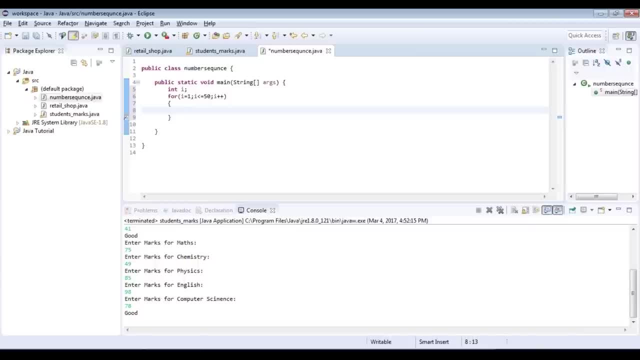 So, first thing, let me check if the number is odd or even So. to do that, all you have to do is say if i modulo 2.. So if my number divided by 2. Is going to be equal to 0., 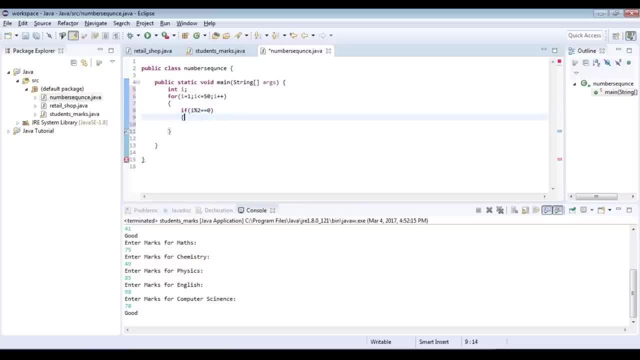 Then that means that the number is an even number, Because all even numbers, when divided by 2, gives me a reminder 0. So in that case I'm going to write a continue statement. That means, don't bother with the statements after this. go ahead to the next iteration. 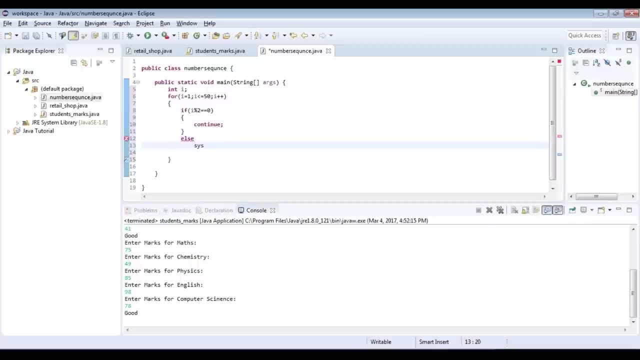 If not, then else I'm going to print that number. So what happens here is that it's going to run and print all the odd numbers Till 50. Save it and let's execute this So you can see all the odd numbers are printed. 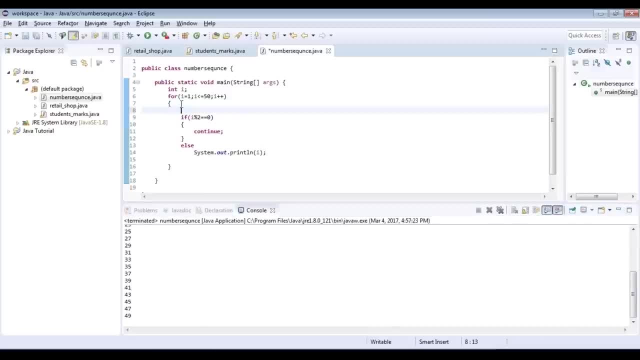 But let's say I don't want to print the numbers that are more than 20.. Then I'm going to write another statement If i greater than 20.. In that case, break. So you need to change it to else if. and then let's run this again. 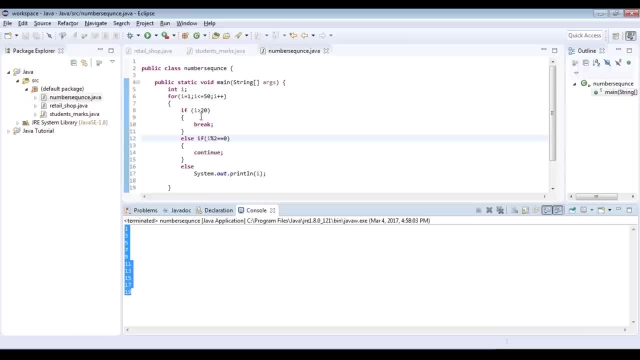 So you can see here, initially when it was printing till 50. But at this point, when it is greater than 20. It's breaking out from that loop. So I hope you're clear with respect to how the for loop works, How the while loop works. 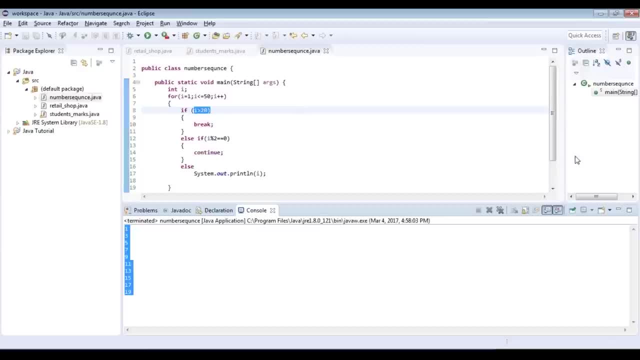 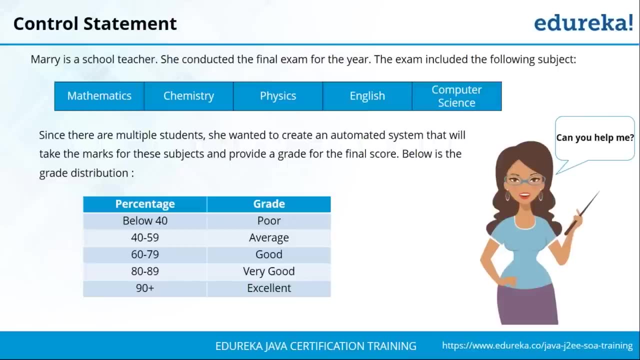 How the do while loop works And how the break and continue statement are part of this programming stack. So I've got a confirmation from Divya Prashant Bharat, So that's great to see guys. Now I hope you guys are trying out these codes simultaneously. 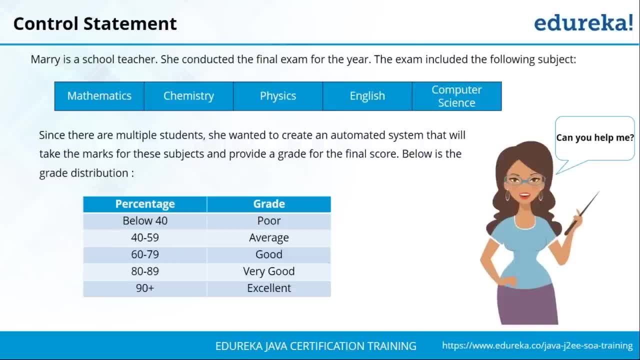 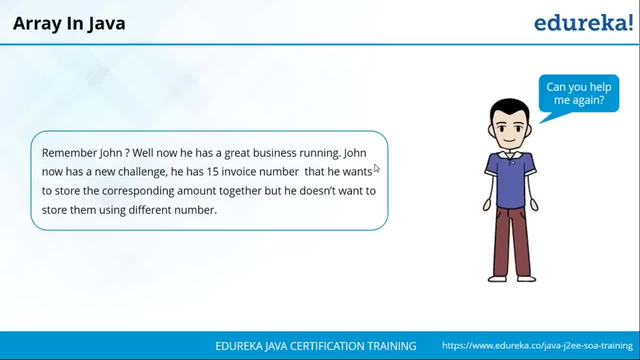 So that, in case You're facing any challenges, You can let me know and I'll be able to assist you as well. So, moving forward, we're going to talk about the next concept, that is, arrays in Java. So remember our good old friend John. 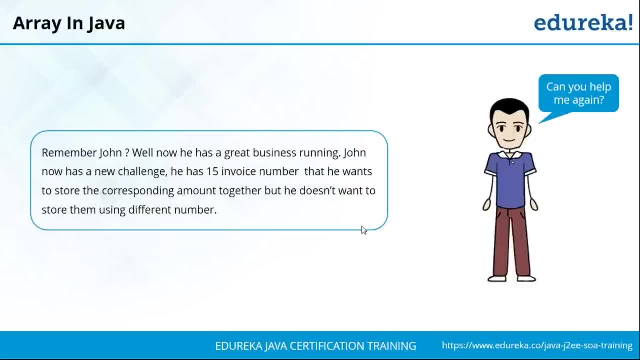 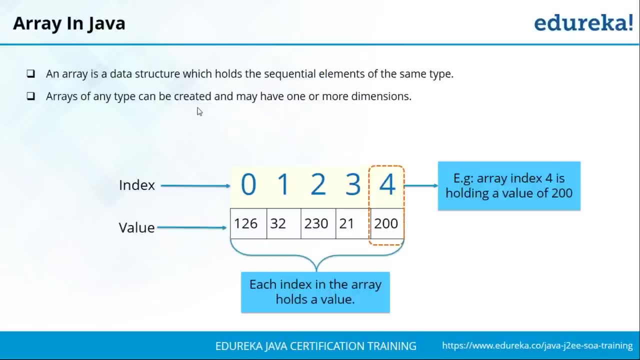 John is facing a new problem now. Now John has 15 invoices that he wants to store with the corresponding amount, But he doesn't want to store them as different number. Now, to solve John's problem, we have a data structure that is array. 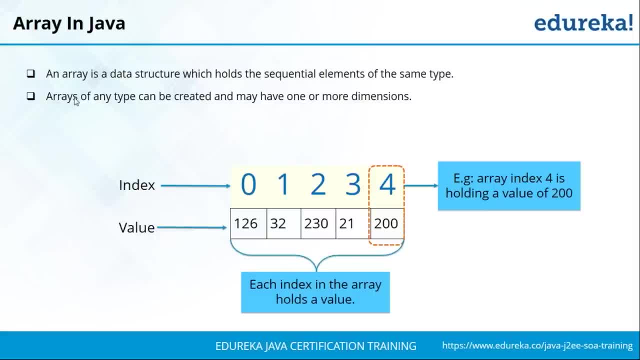 Now an array is used to store elements of the same type in a sequential order. Now an array can also be single dimensional or multi-dimensional, and each array has mainly two components Now. the first is its corresponding index and the second is the corresponding values. 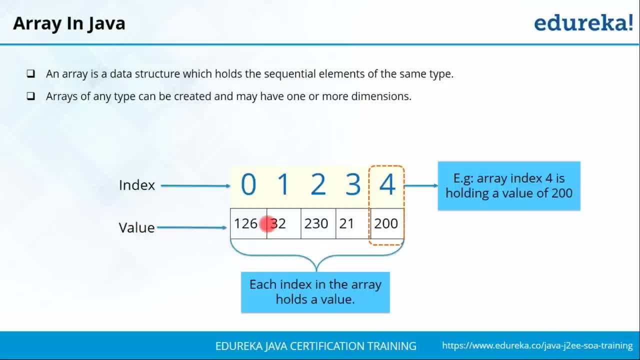 So when you have a sequence of values to be stored, they'll be stored in the value segment and the index is something that gets automatically incremented based on the number of values you want to store. So the indexing starts from zero and goes on till n minus one of the size of the array. 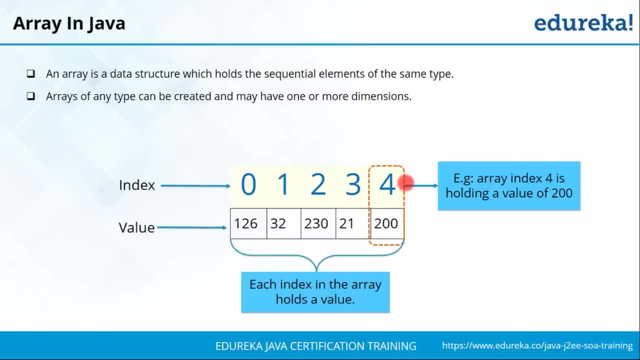 So let's say, if you want to store 15 numbers, Then It starts from zero and goes all the way to 14.. But let's say, if you want to extract a specific value from an array index, That is, let's say you want the fourth value present there. 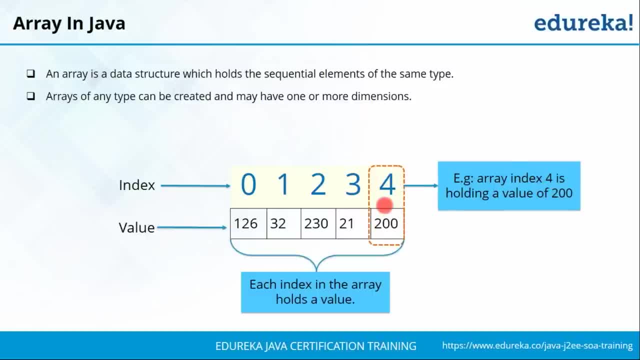 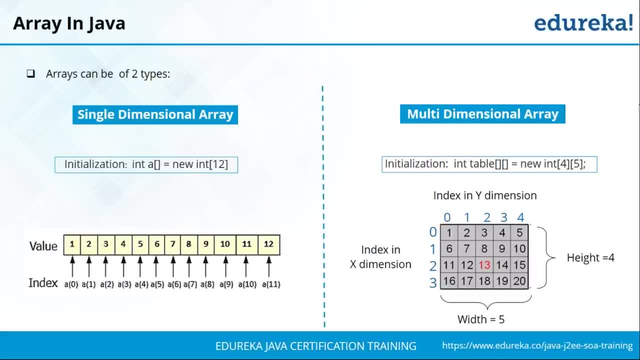 Then you need to only specify the corresponding index and the value can be extracted from this. Now, I've already told you there are two types of array. You have the single dimensional array and you have the multi-dimensional array. Now for initializing the single dimensional array, you have this following syntax: where: 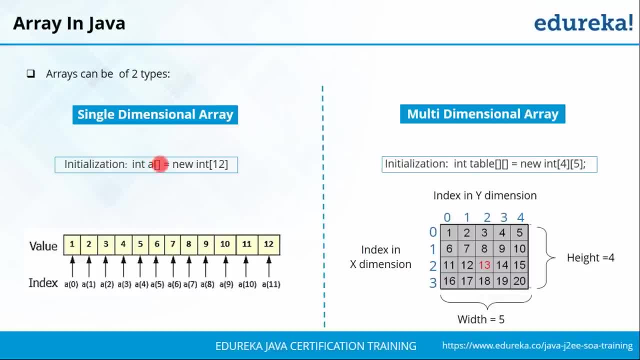 you specify the data type of the array, then the name, and then you use square parenthesis. This is to help Java understand that it is going to be an array. Then you need to specify the keyword new I had mentioned to you earlier as well. You're going to use new to create new objects. as such, 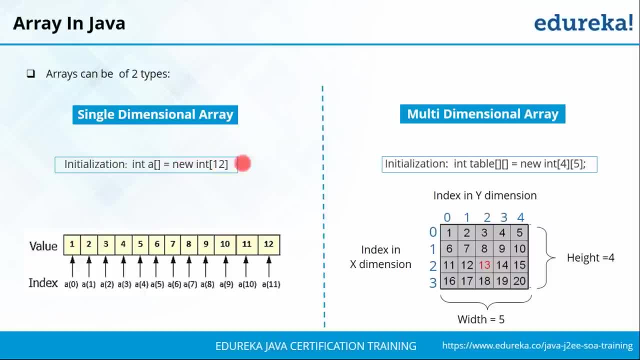 So here array is also an object, and then again the data type as well as the size of the array. So below you can see we've created an array with the name A, of the size 12. The indexing starts from zero and goes on all the way to 11 and corresponding values. 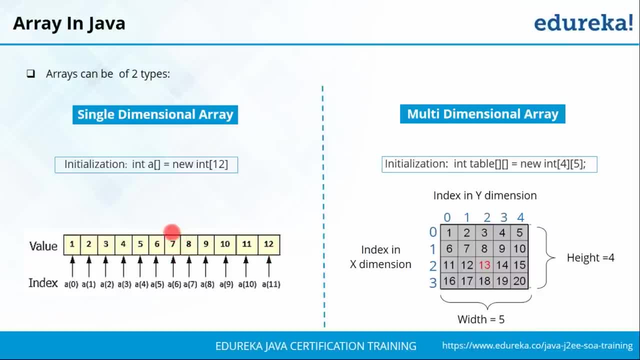 are being stored here. So let's say, if you want the value of seven, Then all you need to do is take A of six. Now, when we talk about a multi-dimensional array, your data is going to be stored in a matrix format. 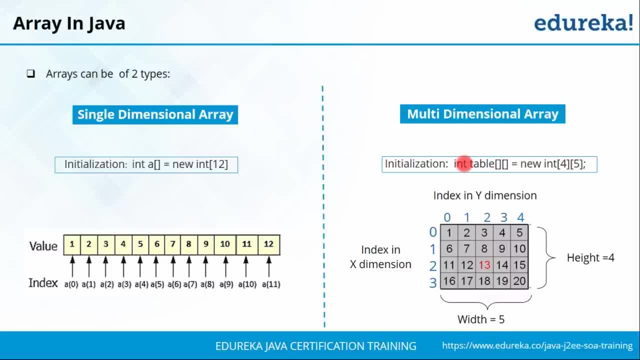 So you can see, the initialization is also slightly different. You again specify the data type, the name of the table, then you're going to use two sets of square brackets. Now, this is to help Java understand that this is not a single dimensional array, but a multi-dimensional. 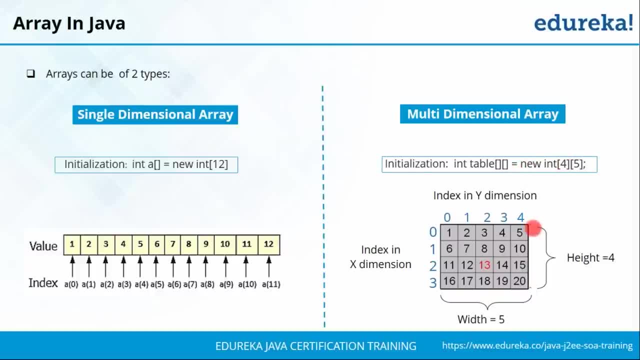 array. Then again the new keyword comes, followed by the size of the multi-dimensional array. So here you can see that this is an array. So here you can see. we specified the number four and five. This is to help Java understand that I need four rows and five columns in my table. 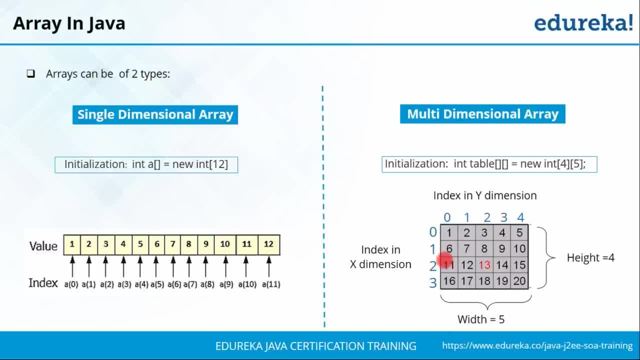 So you can see here the array indexing starts from zero to three for the rows and zero to four for the columns. So this is how your multi-dimensional array looks like. It's similar to a matrix that you use in mathematics. So I hope you're clear with respect to how an array looks like and how to initialize. 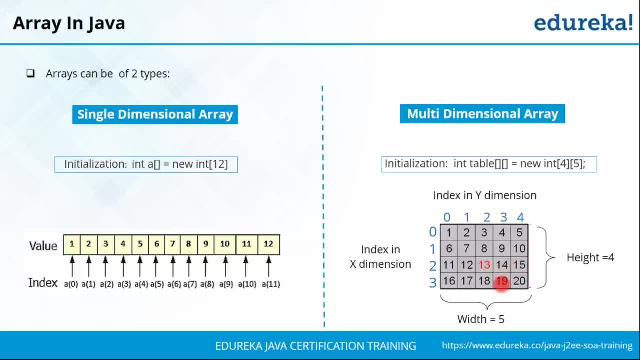 one, because we're going to go ahead and help John out with his invoice problem. All right, So Divya has given me a confirmation. So is Bharat, Adam, Henry Prashant. Let's go back to our Eclipse. So here let me create a new class. 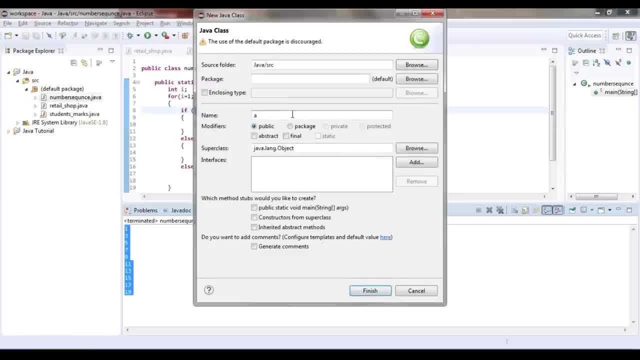 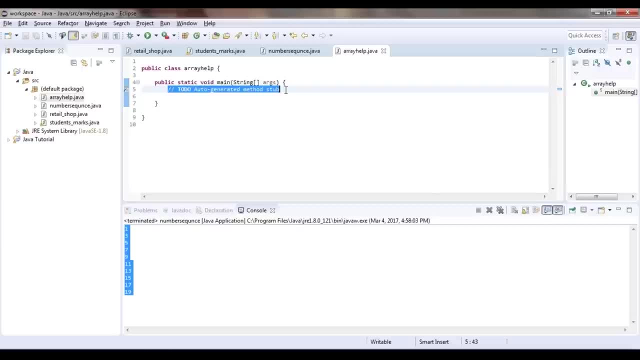 I'm going to call it array help. So we need a two dimensional array. So again, this is going to have amount. So what I'm going to do is that I'm going to make it a multi-dimensional array of double form, So double. 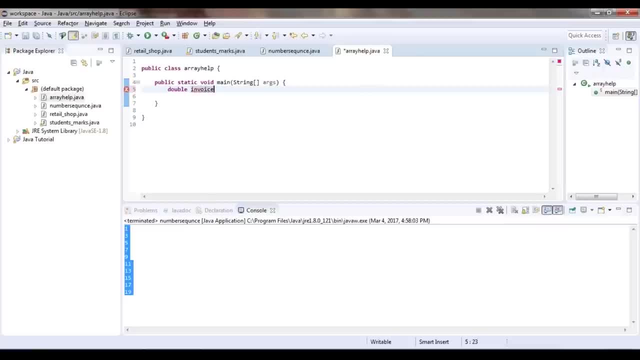 I'm going to say invoice, and then you need to specify that it's a multi-dimensional array. So two square brackets and then equal to new double. So here you need to specify the size of the array. Now John had told us he had 15 invoices and he also said that he wants to store the invoice. 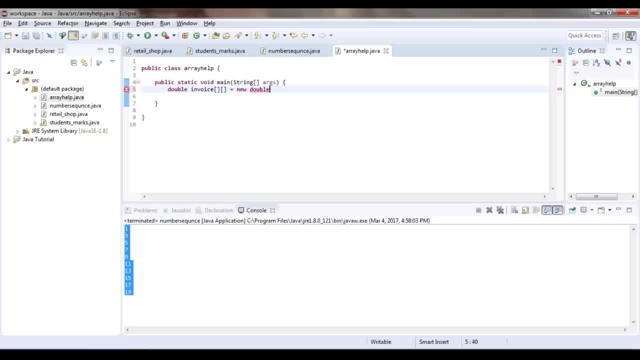 number with the corresponding amount. So, basically, I'm going to create a new tool, Two dimensional table, which is going to have 15 rows and two columns. Now, to do that, you need to first say 15 and in the second case it's going to be two. 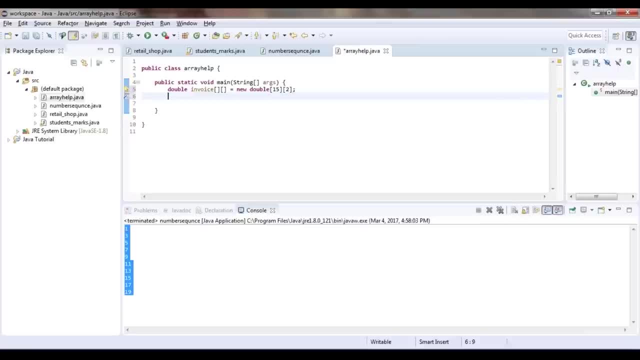 So any doubts on how to create a multi-dimensional array? All right. So to access a multi-dimensional array, what you're going to need is that you're going to need multiple nested for loops. So let me just show you how it's done. 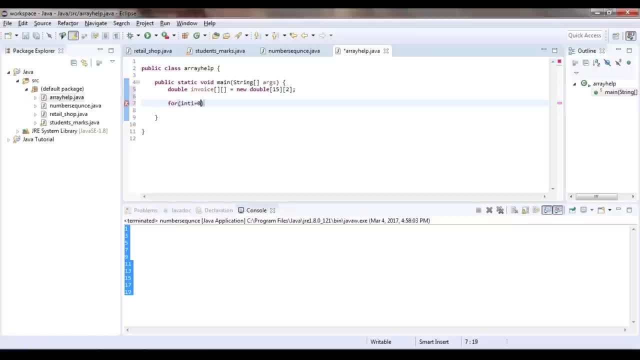 So let's say for int i equal to zero, My i should be less than 15- that is the row number- and i plus plus Now for j equal to again zero, j less than two j plus plus. So here, first I'm going to ask him to enter the value. 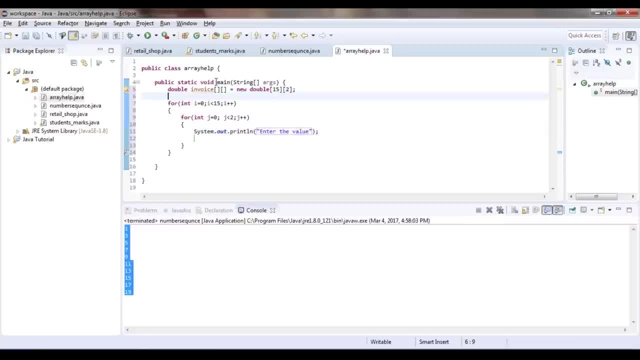 And then I'm going to take the input Now again, if you remember how to take input, you need to first import util javautil star. So this command completely loads the utils and you can go ahead and then create a scanner. object: new ca scanner. 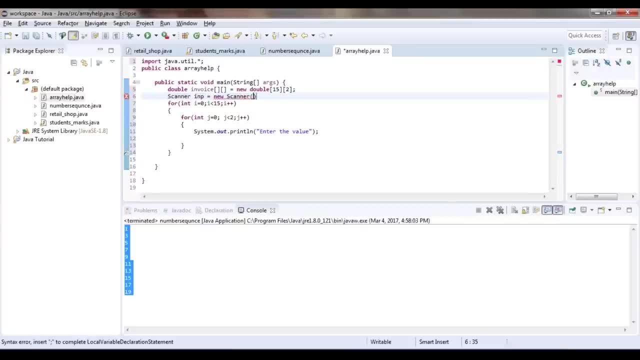 util, util, util, util. And this is a system input, so sysinput. So now it's time I take the input from the user and then store it into my invoice table. So invoice of i, that is my row and my column is equal to input dot. next double. 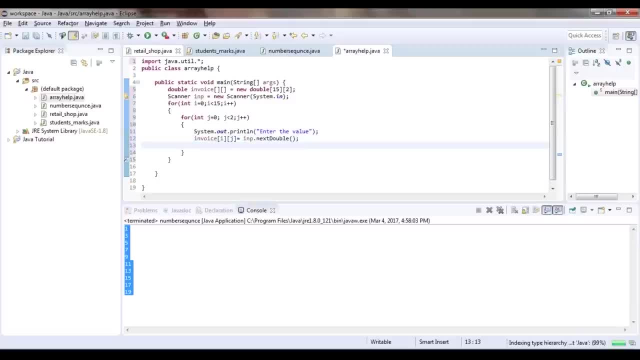 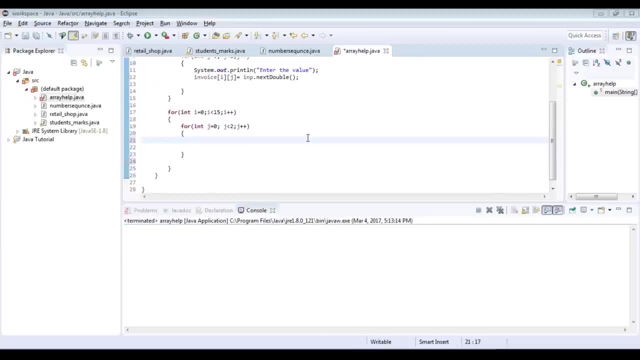 So are you clear on how to take an input for the array? No Printing out the output. what you're gonna do is that you're gonna use a system output in which you can directly print the value, Which is, if i, comma, j, then a colon. 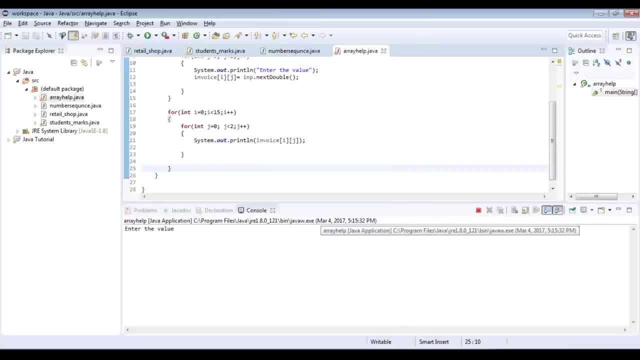 So let's just run this program. It's gonna ask me set of values. So I'm gonna give random set of values here, So let's say 157.0.. So you have your complete set of values that is being displayed here. 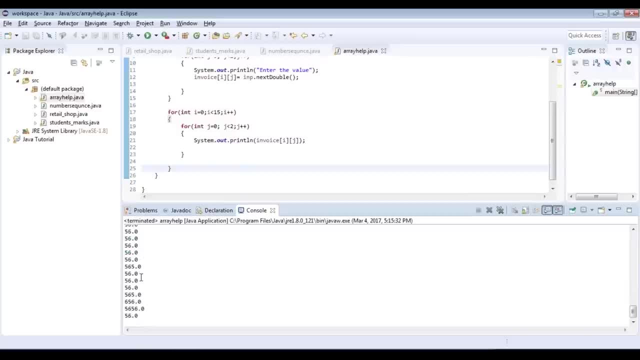 So are you clear with respect to how arrays work and how we've stored it separately. Now, this is just a sample value, so don't go by that, But again, I hope you enjoyed this video. I hope you got the idea of how to use arrays. 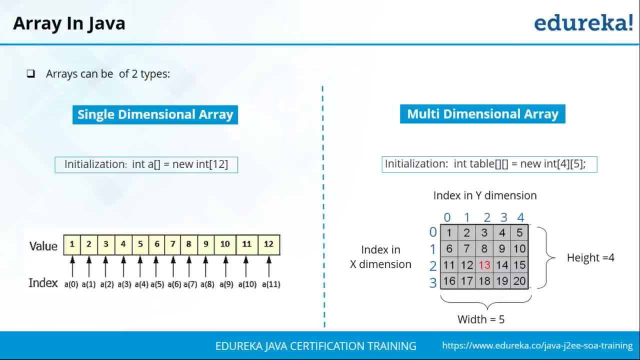 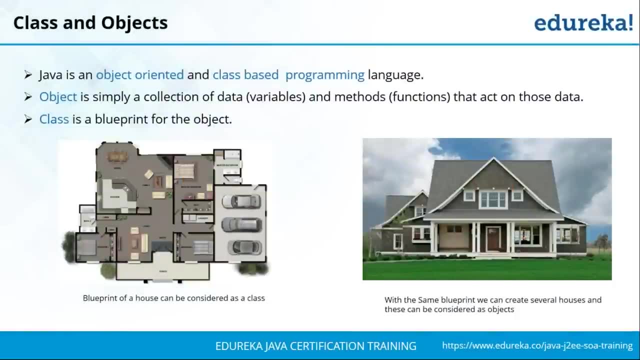 So, coming back to our presentation, we've helped John solve with it And finally, we come to our final topic, that is, the object oriented programming. Now, everyone of you already heard about object oriented programming style. I've also discussed about how everything is considered. 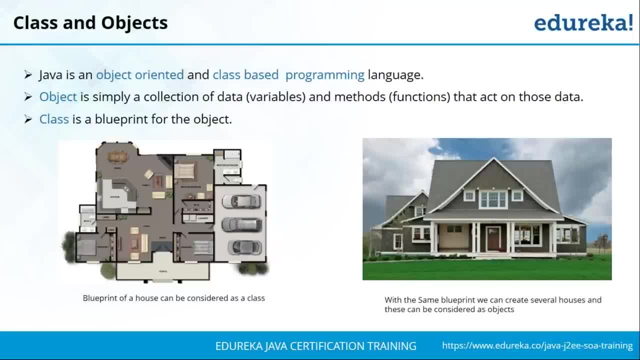 to be an object in Java. But let's just give have a brief overview of what a class is and what an object is here. After that we move forward to discuss the four main concepts of object oriented programming. Java is object oriented and a class based programming line. 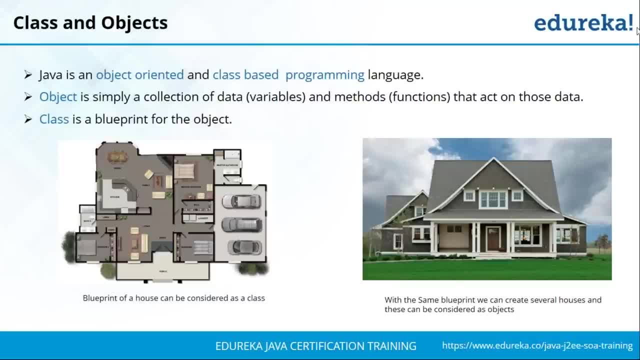 So we've seen how Java is a class based programming style and I've already told you, everything here is considered to be an object. But then you may have been wondering: what is an object in itself? So, basically, when you talk about an object, anything that exists can be considered to be an object. 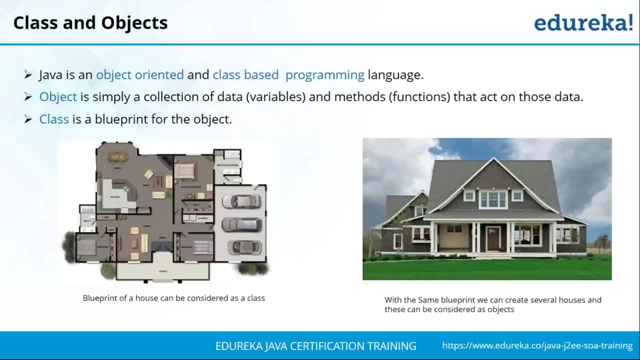 So let's say you and I are actually objects from the human class. Or let's say your dog or your cat is an object from the animal class as such. So I hope you get the idea. So in a class you're gonna define what are the basic functionalities. 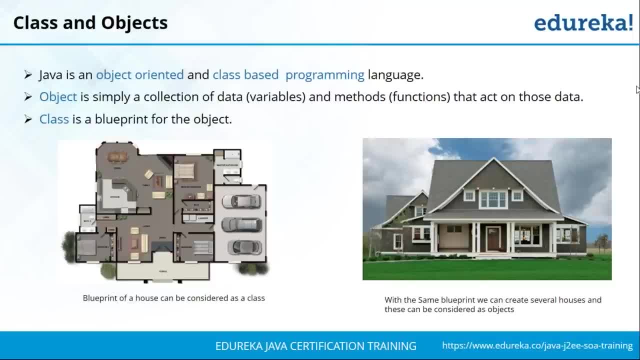 each of the objects should have, but each object is unique when compared to each other, Like how you and I are not the same, but even though we are objects from the human class. Now, to give you a better understanding: here you can see how a blueprint of a house is depicted. 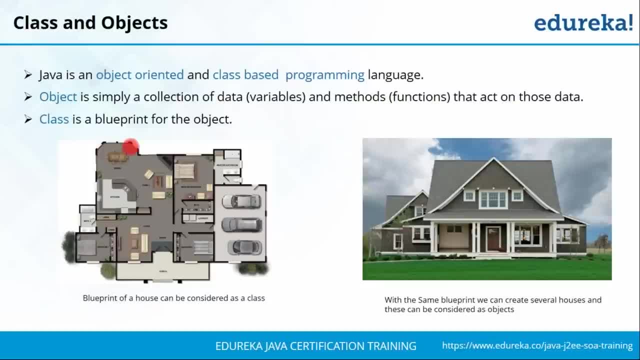 Now this, basically, is your class. This tells you how the house should look like, But your individual house in itself is an object. It may have the same features as the class, but there would be certain changes with respect to this And you cannot expect all the houses. 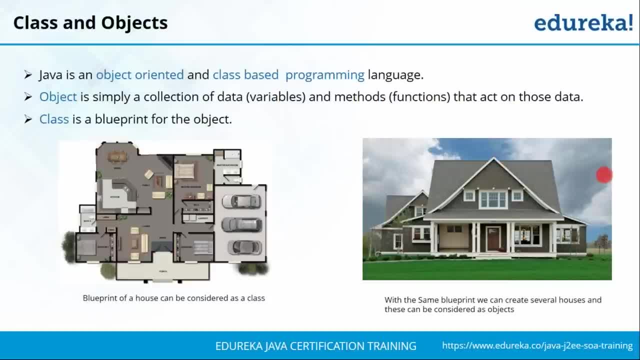 designed with the same blueprint to be the same, because there may be slight variations as such. So are you clear with respect to what is a class and what is an object. Now, to call any programming language as an object-oriented programming language, there are mainly four concepts that it needs to cover. 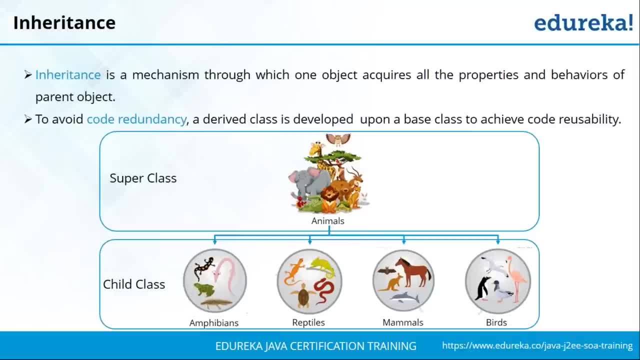 Now, the first concept that we'll be discussing is inheritance. Now, basically, inheritance is a mechanism through which one object acquires all the properties from its parent object. So we've already seen this concept. actually, I just gave you an example as well. 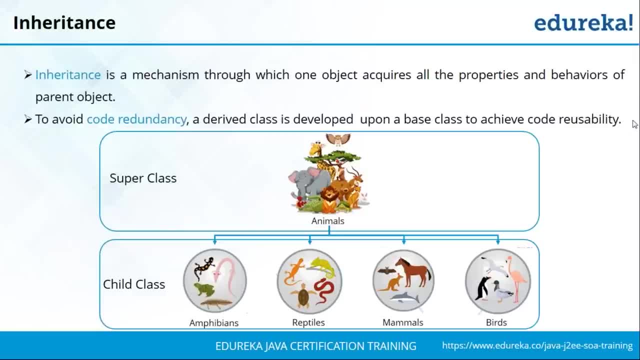 Now, if you see in the image here, it's referring to the same example where your super class or your parent class is animals, but when you look at the child class, it can be amphibians, it can be reptiles, it can be mammals or it could be birds. 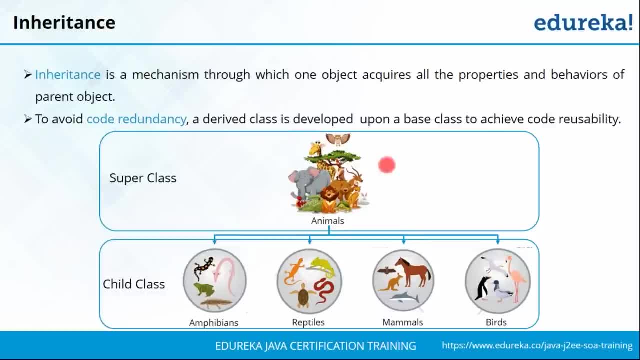 But when you look at their parents, it's considered to be animals as a super class. Now, through inheritance you can achieve code redundancy And you can highly make use of code reusability. So let's say there's some common function or some common variable that you want to be present. 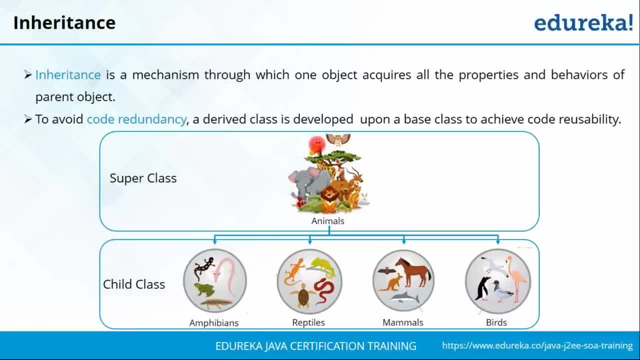 across multiple classes, then all you need to do is specify that into the base class or the parent class. Then all the childs that we're inheriting from this class will have the same set of variables or functions. Now talking about functions. functions, basically, are set of codes. 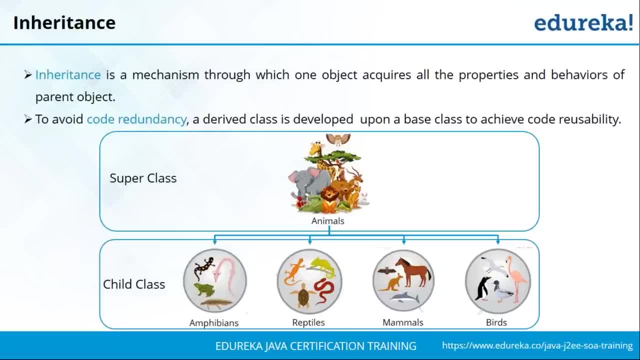 So these codes would perform a specific operation and give you the desired result. Again, functions are quite handy when you have to perform specific set of operations with different sets of values. Now, don't worry, we'll be talking extensively about functions as well as these concepts. 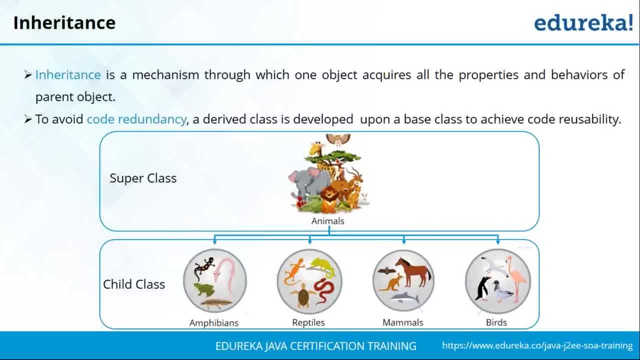 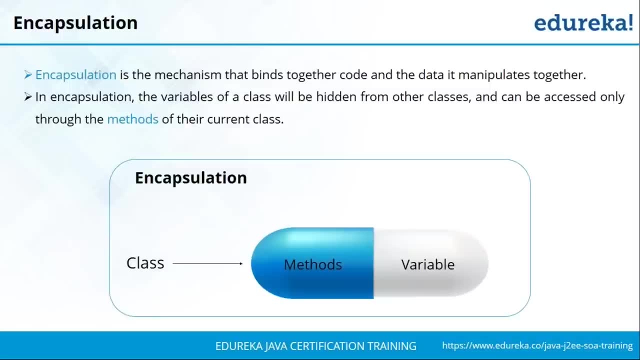 in our upcoming session, but let's just have an overview of these concepts as well. After that we have the encapsulation concept. Again, encapsulation is a highly useful concept in object-oriented programming. Now, through encapsulation, what you're gonna ensure is that 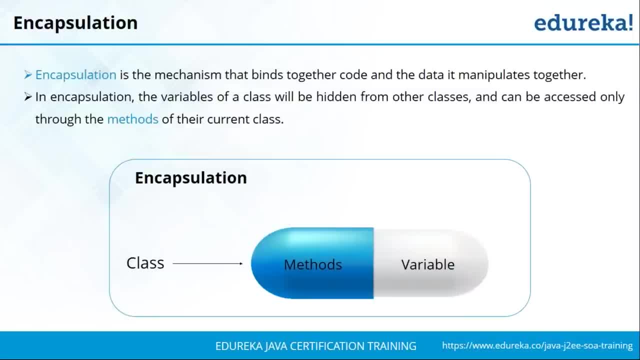 now, the variables that are present in a class can only be modified or changed by a method present in the same class. So let's say you have multiple classes that are linked to each other and one class is trying to change the value of a variable present in the other class. 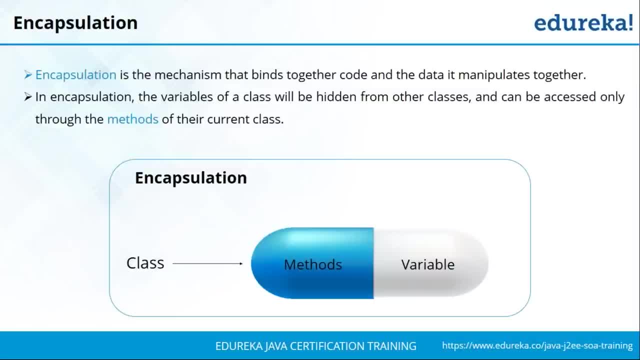 Now this is not directly possible. To do that, you need to have an object from the class in which you want to change the variable name. So basically, what you're doing here is that you're binding the code and the data manipulation together. 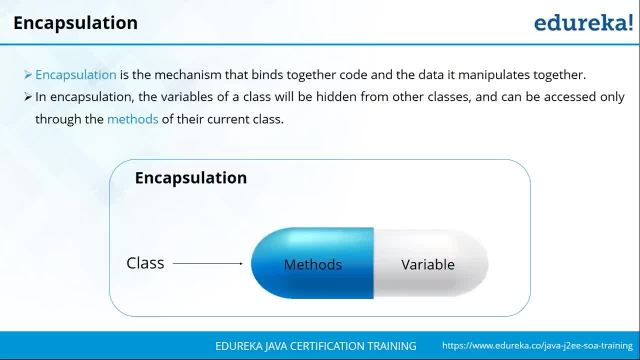 That is, if an object belongs to a class, then only a method from that class can change the value of that object. So are you clear with respect to encapsulation and inheritance. Okay, Prashant is clear. Bharat Henry Divya. 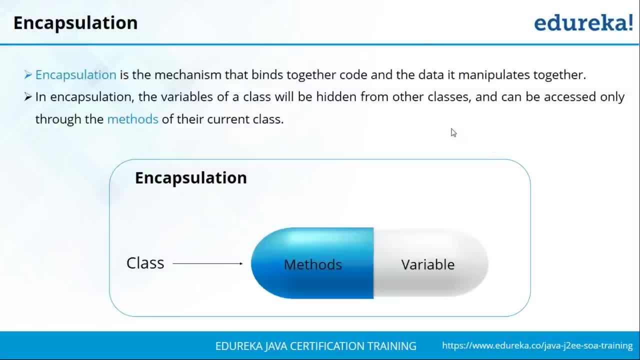 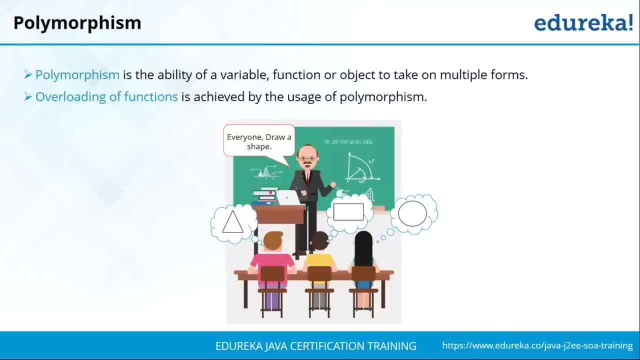 that's great to see. Now, moving on, the next concept that we're gonna be discussing about, that is polymorphism. Now, a polymorphism basically is ability of a variable or a function, or even an object, to take multiple forms. 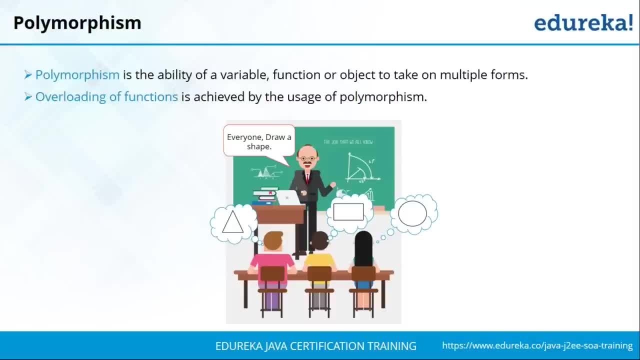 So here we're not gonna go in much in detail with respect to how a polymorphism is applicable here, because one of the key achievements that you're gonna get through polymorphism is obtained through function overloading, And I'll just give you an introduction. 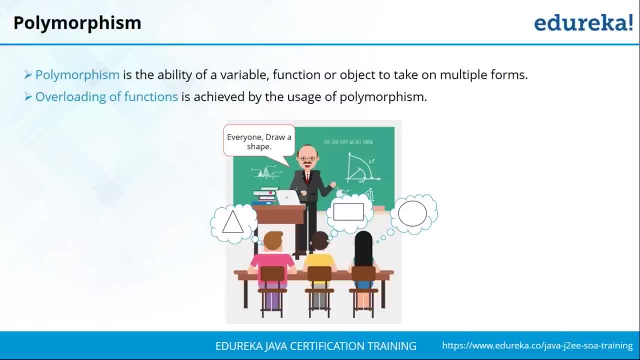 of function overloading here. So let's say you're writing multiple lines of code. And again let's go into the example itself. Let's say you wanna draw a specific diagram. Now you're gonna have multiple functions present already as part of your program. 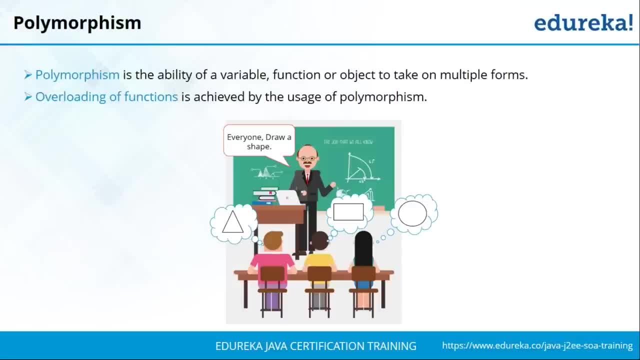 So the functions that deal with drawing. I'm just gonna call them draw. But based on the values that I pass to these functions, it is going to draw different shapes. So let's say, in case of a rectangle, I'm gonna need two values, that is. 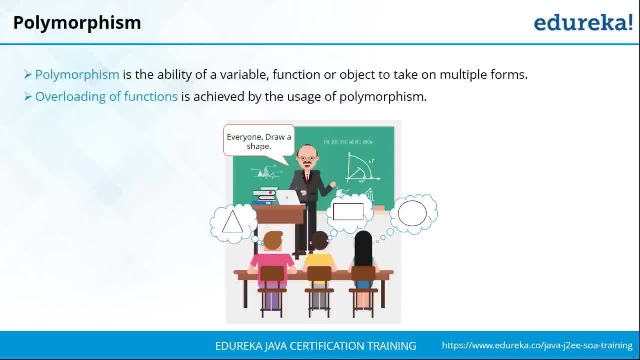 length and breadth. Let's say, in case of a circle, I'm gonna need at least the radius of it. I hope you get the general idea Based on the values that you pass. different functions will be called. That serves different purposes. 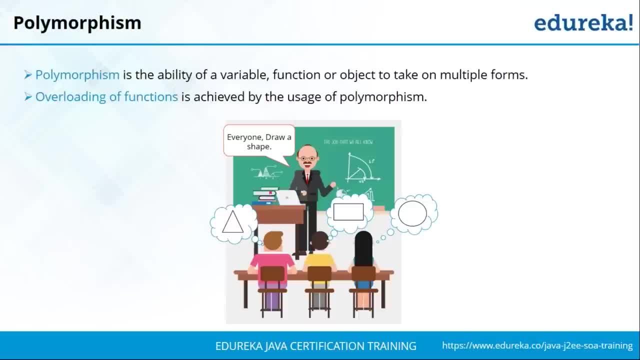 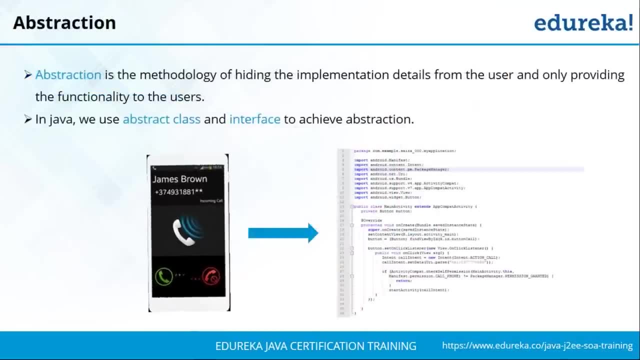 So this is achieved using function overloading. Now, don't worry if you're not clear with this, I'll be talking about this extensively in our next session. Now, final concept that we are talking about is data abstraction. Now, basically, when we talk about data abstraction, 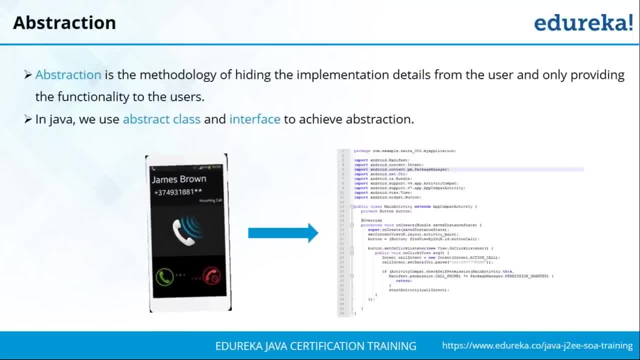 it means that you're hiding the details and only showing the essential details. Now, if you look at the image here, basically whenever we get a call, we just see an option to either pick it up or cancel it, But in truth, there are a lot of codes. 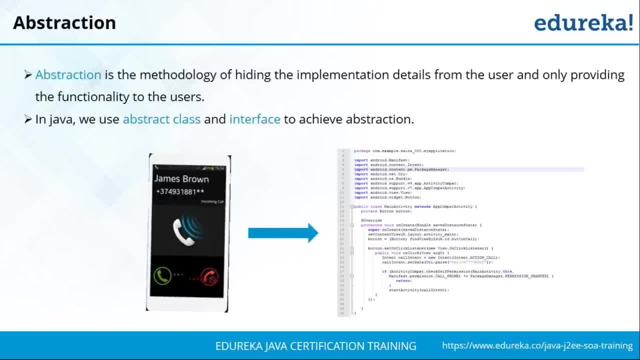 that run for every action that you do, But we do not need to worry about that. All we need to do if we need to pick up a call is either swipe right or, if you wanna cut the call, you're gonna swipe left. 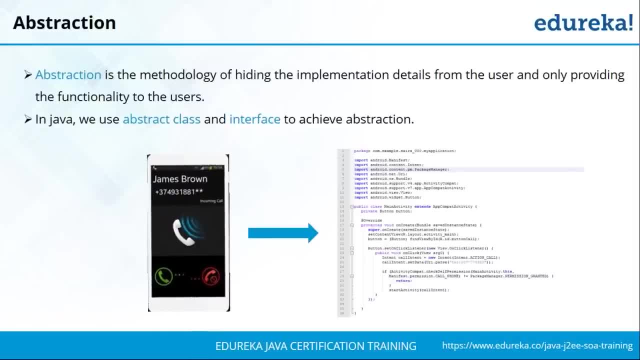 And in Java you're gonna again obtain abstraction through abstract classes and interfaces. This is something that we'll be covering as part of our upcoming sessions as well, So I hope with this you've got a complete overview of the various object-oriented concepts of Java. 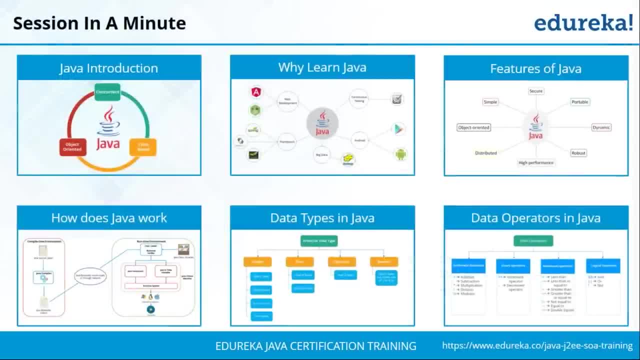 And moving forward. let's look at summary of today's session. We started with an introduction of Java. Then I helped you understand why learn Java. We saw the key features of Java, or the buzzwords as they are called these days- Then I helped you understand how Java works. 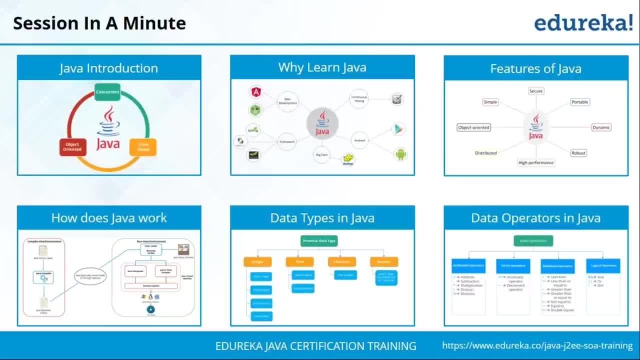 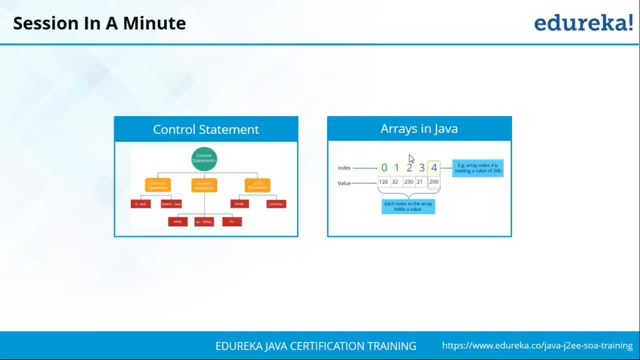 and we discussed the various data types and the data operators in Java. Finally, moving forward, we saw the various control statements and the arrays present in Java. So any questions with respect to Java, with respect to today's session? So all right. so the recording of this class.